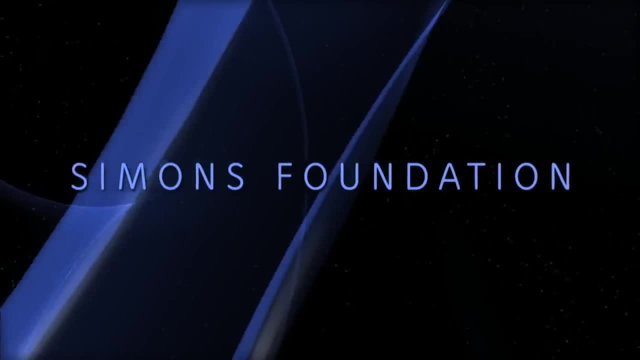 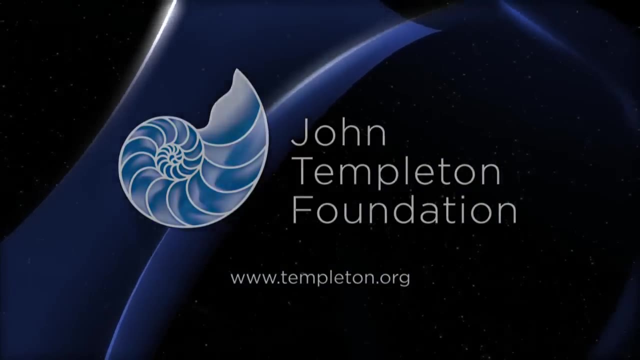 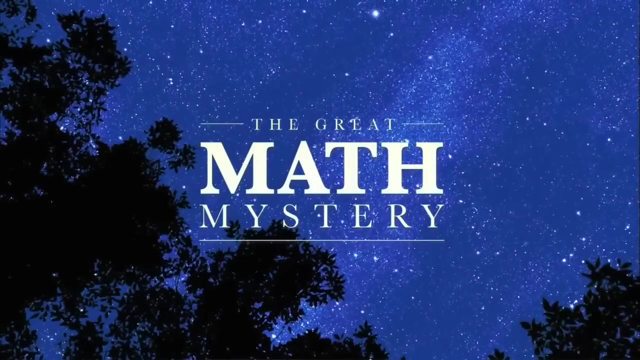 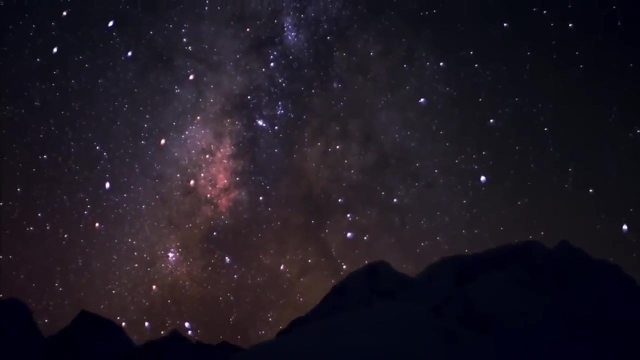 working to advance research in the basic sciences and mathematics. Additional funding is provided by the John Templeton Foundation and the George D Smith Fund. Human beings have always looked at nature and searched for patterns. Eons ago, we gazed at the stars. 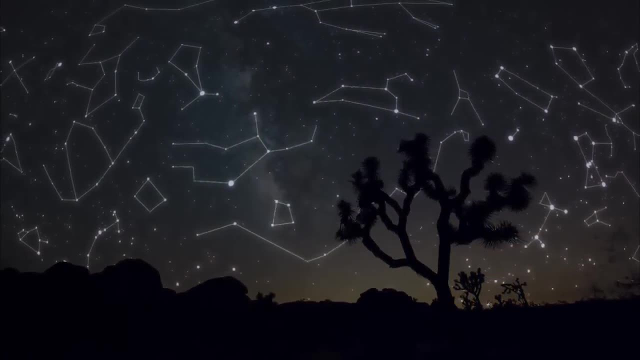 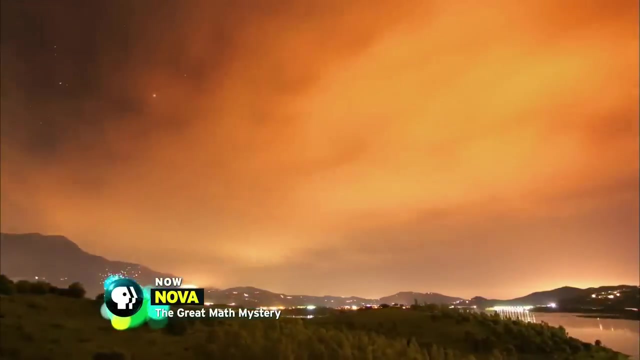 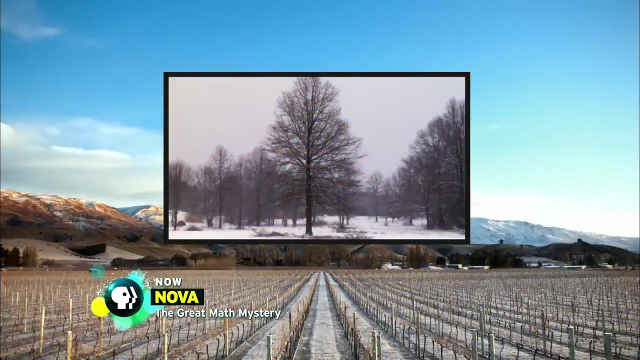 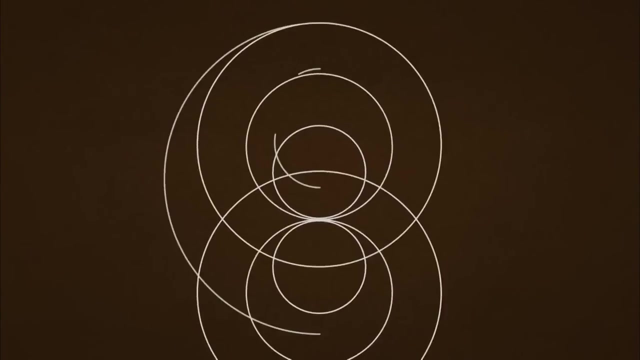 and discovered patterns we call constellations, even coming to believe they might control our destiny. We watched the days turn to night and back to day and saw the stars and seasons as they come and go and called that pattern time. We see symmetrical patterns in the human body. 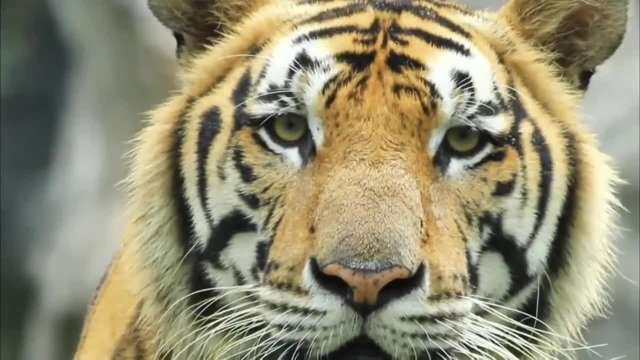 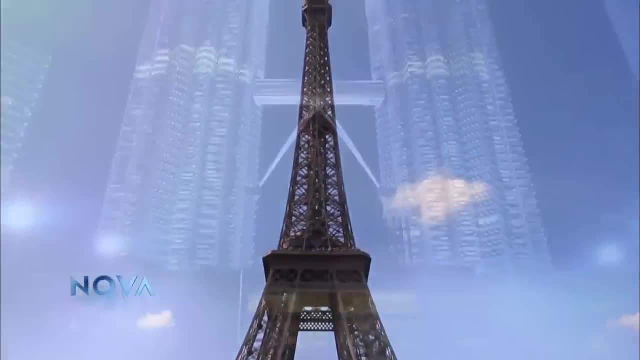 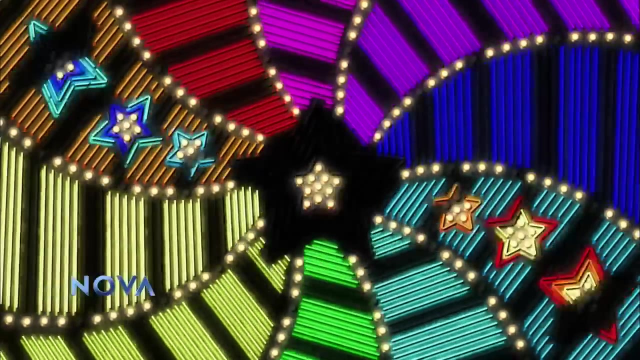 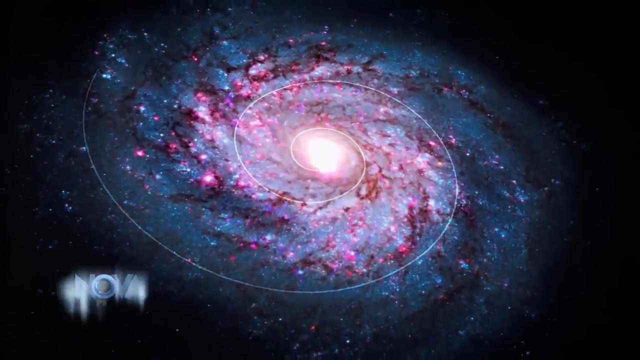 and the tiger's stripes and build those patterns into what we create, from art to our cities. But what do patterns tell us about the universe? Why should the spiral shape of the Nautilus shell be so similar to the spiral of a galaxy? 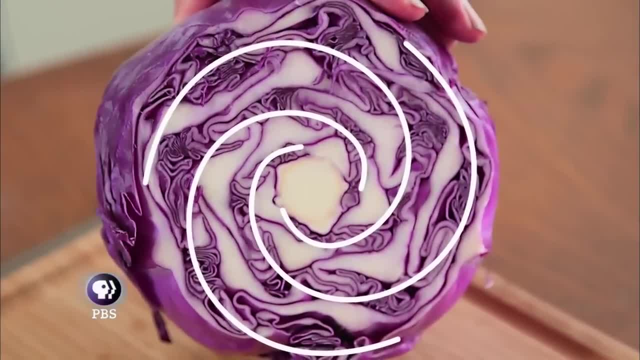 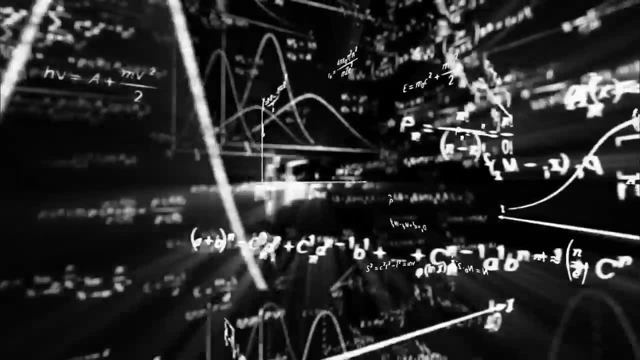 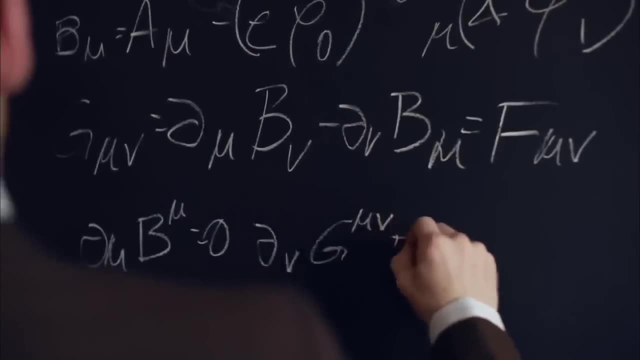 Or the spiral found in a sliced open head of cabbage. When scientists seek to understand the patterns of our world, they often turn to a powerful tool: mathematics. They quantify their observations and use mathematical techniques to examine them, Hoping to discover the underlying causes. 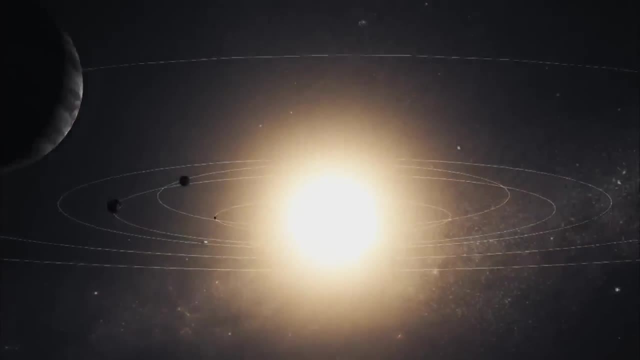 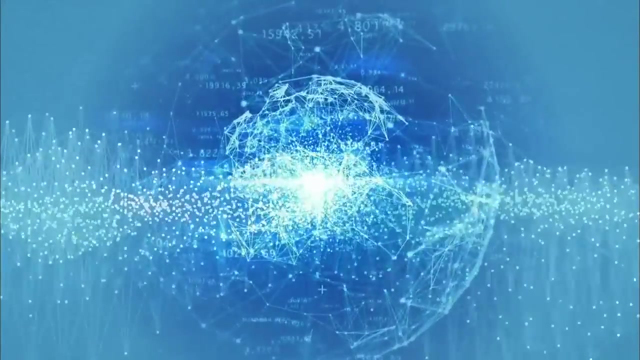 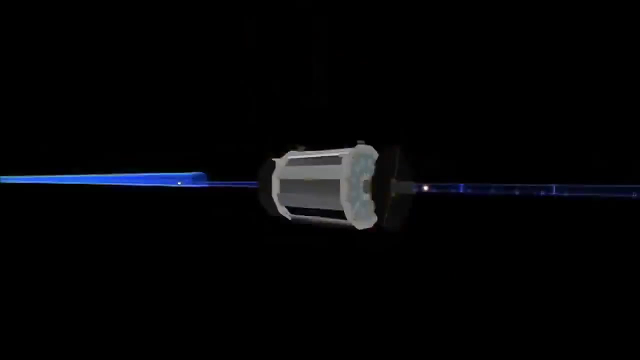 of nature's rhythms and regularities, And it's worked, revealing the secrets behind the elliptical orbits of the planets to the electromagnetic waves that connect our cell phones. Mathematics has even guided the way leading us right down to the subatomic building blocks. 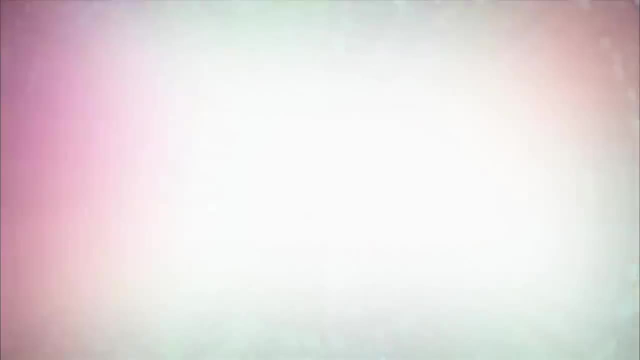 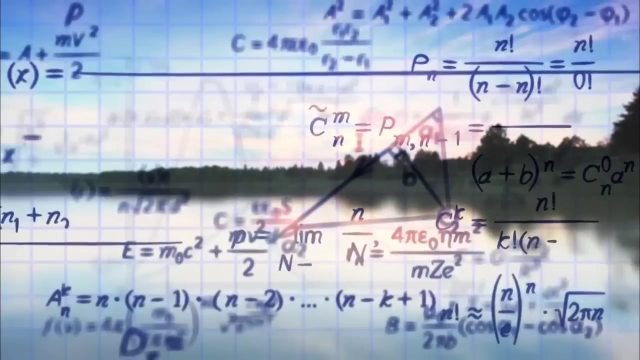 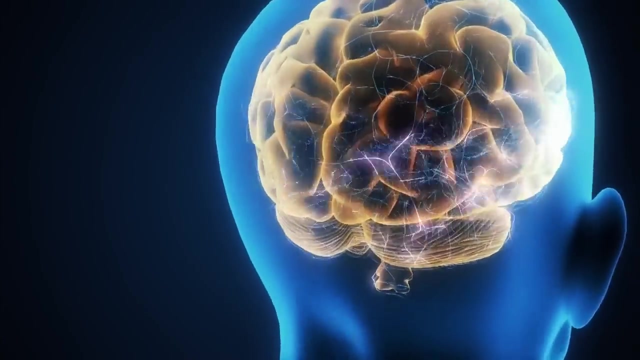 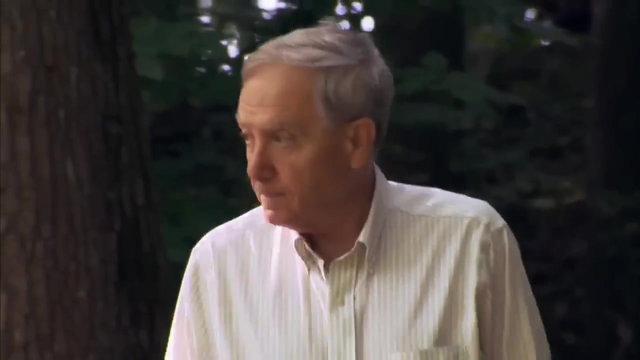 of matter, which raises the question: why does it matter? Why does it work at all? Is there an inherent mathematical nature to reality, Or is mathematics all in our heads? Mario Livio is an astrophysicist who wrestles with these questions. 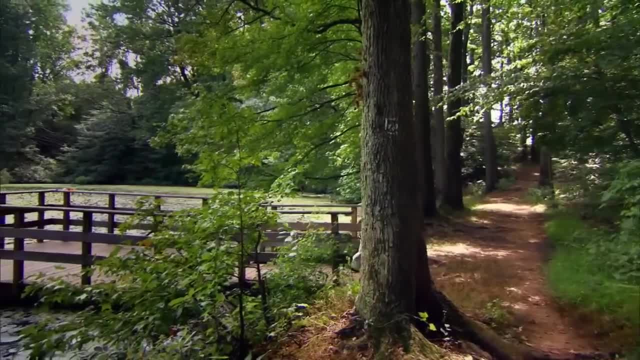 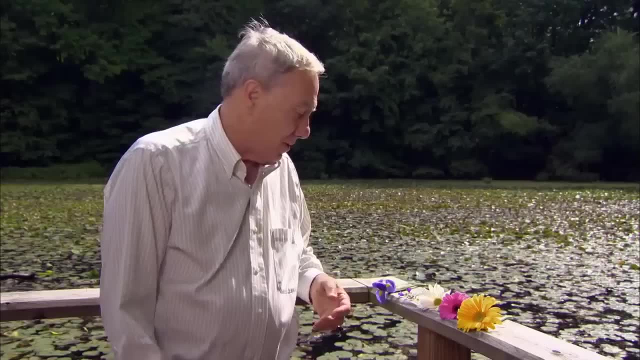 He's fascinated by the deep and often mysterious connection between mathematics and the world. If you look at nature, there are numbers all around us, You know. look at flowers, for example. So there are many flowers that have three petals, like this. or five like this. Some of them may have 34 or 55. These numbers occur very often. These may sound like random numbers, but they're all part of what is known as the Fibonacci sequence, a series of numbers developed by a 13th century mathematician. 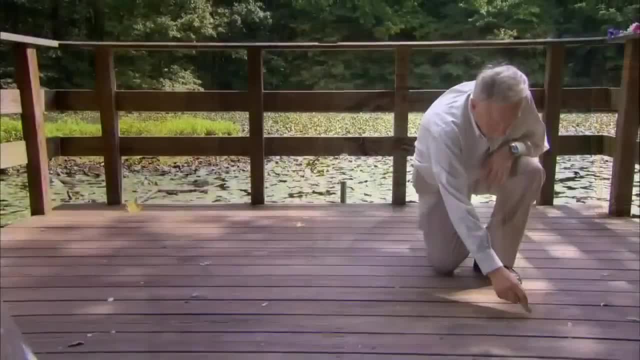 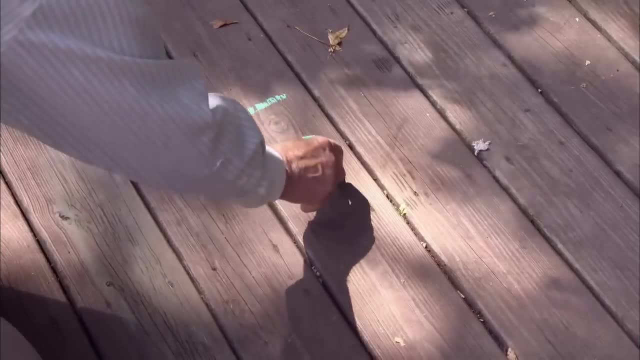 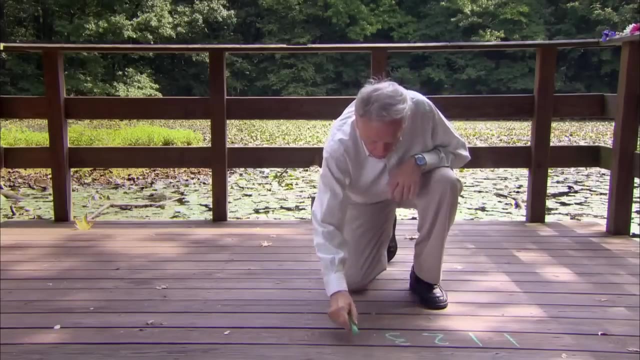 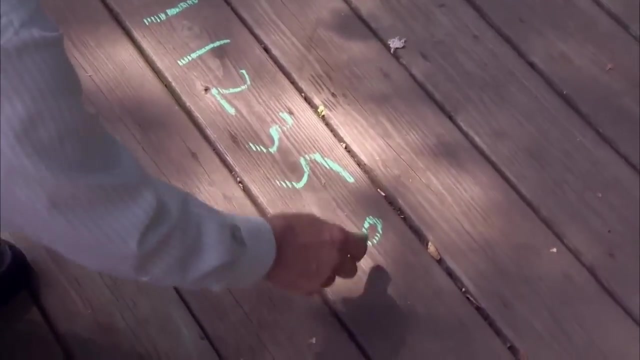 You start with the numbers one and one, And from that point on you keep adding up the last two numbers. So one plus one is two. Now one plus two is three, Two plus three is five, Three plus five is eight. And you keep going like this. 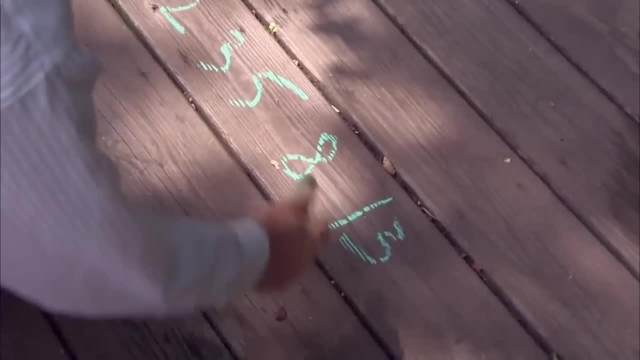 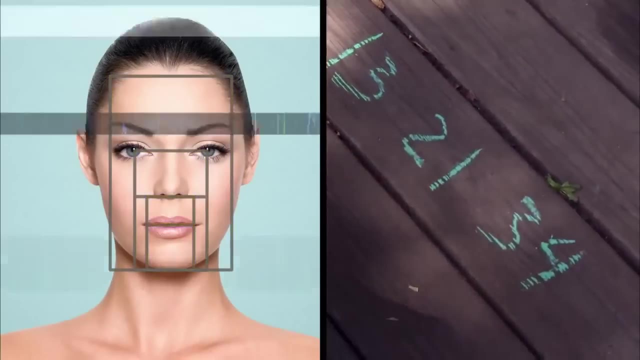 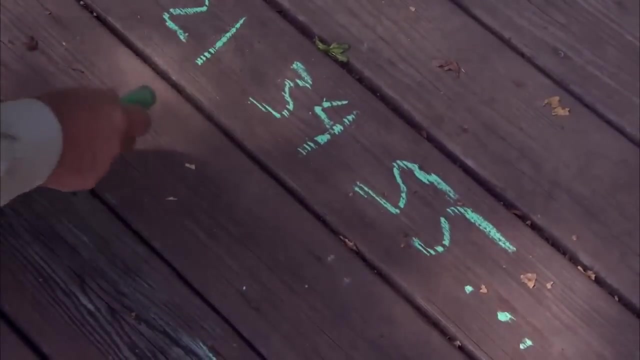 Today, hundreds of years later, this seemingly arbitrary progression of numbers fastens. But Fibonacci numbers fascinates many who see in it clues to everything from human beauty to the stock market. While most of those claims remain unproven, it is curious how evolution seems to favor these numbers. 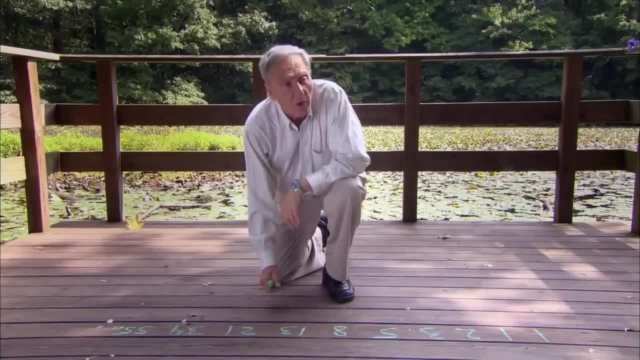 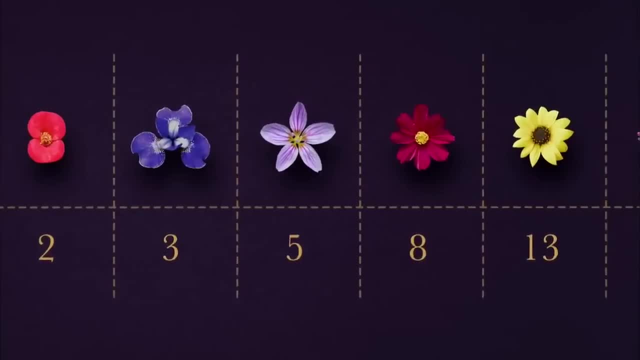 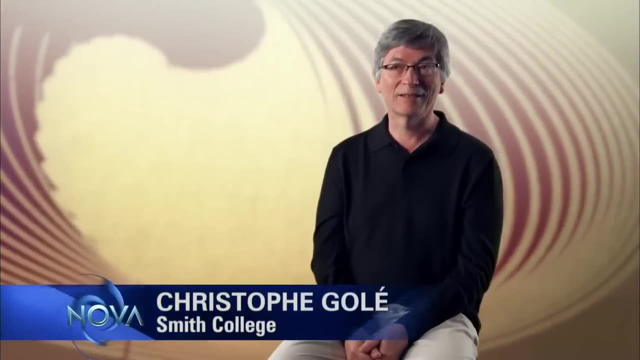 And as it turns out- I mean this sequence- appears quite frequently in nature. Fibonacci numbers show up in petal counts, especially of daisies. But that's just a start. Statistically, the Fibonacci numbers do appear a lot in botany. 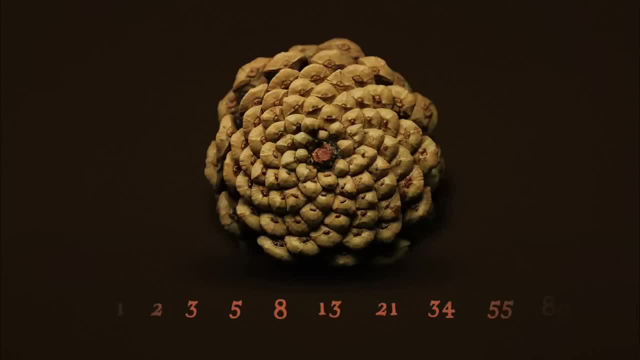 For instance, if you look at the bottom of a pine cone, you will see often spirals in their scales. You end up counting those spirals. You will usually find a Fibonacci number And then you will count the spirals going in the other direction. 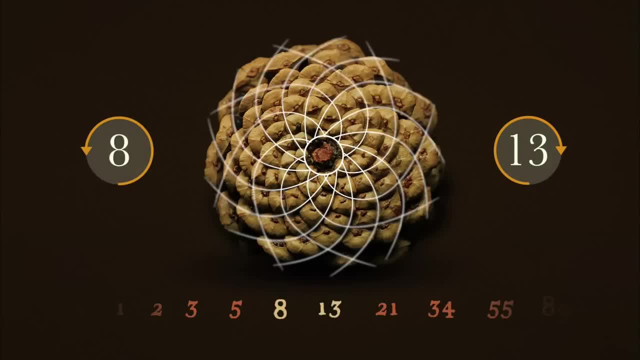 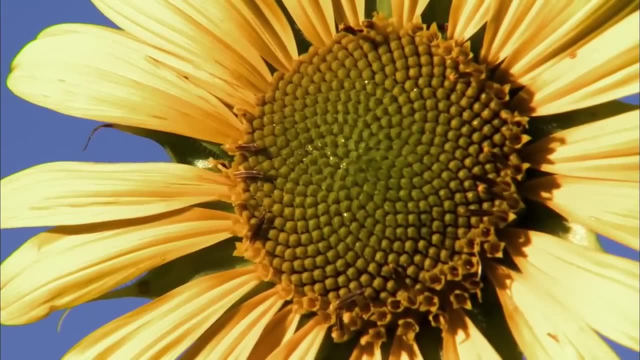 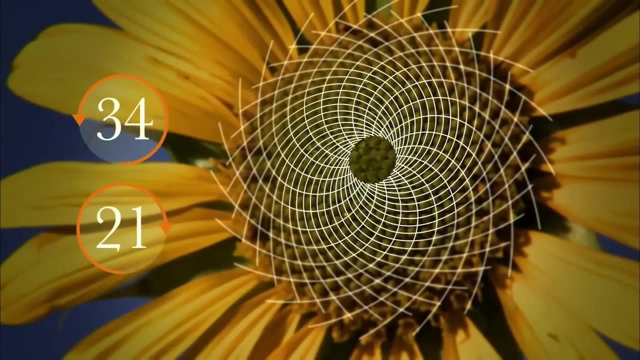 and you will find an adjacent Fibonacci number. The same is true of the seeds on a sunflower head: Two sets of spirals, And if you count the spirals in each direction, both are Fibonacci numbers. While there are some theories explaining the Fibonacci-botany connection, 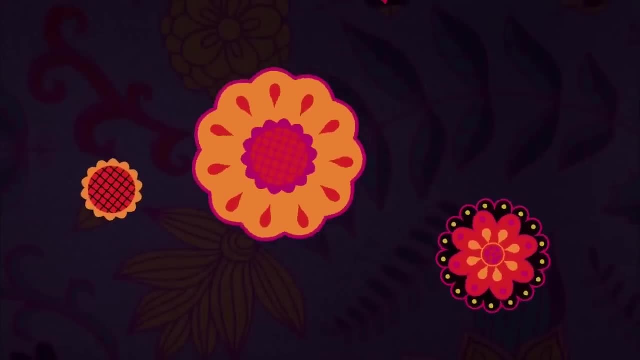 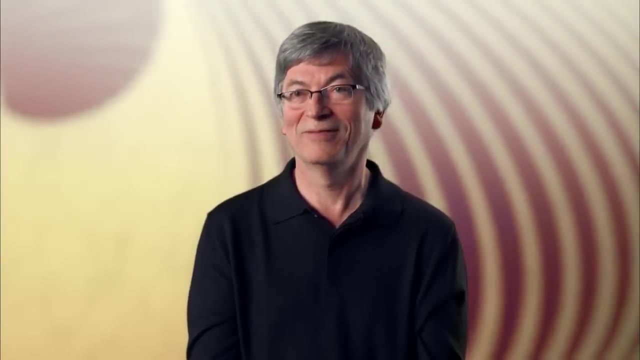 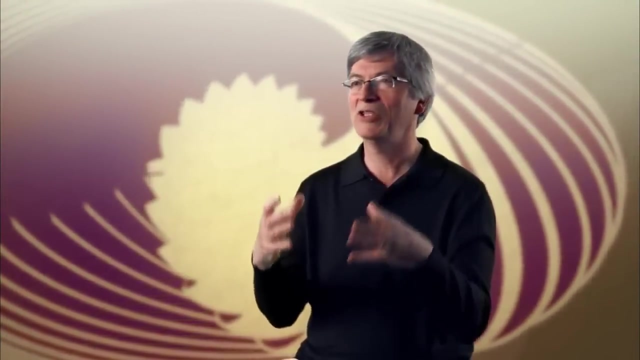 it still raises some intriguing questions. So do plants know math? The short answer to that is no, They don't need to know math. In a very simple geometric way, they set up a little machine that creates the Fibonacci sequence. in many cases, 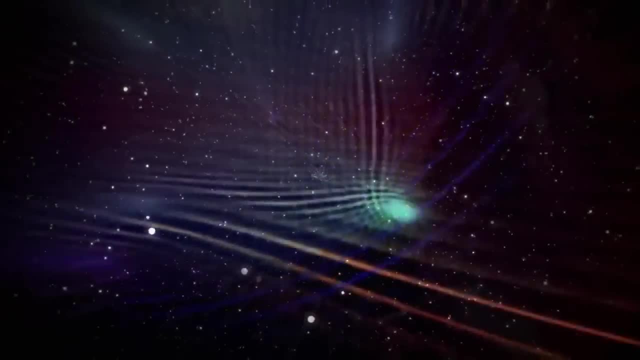 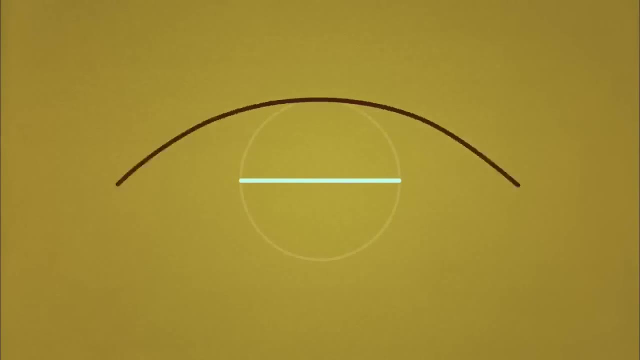 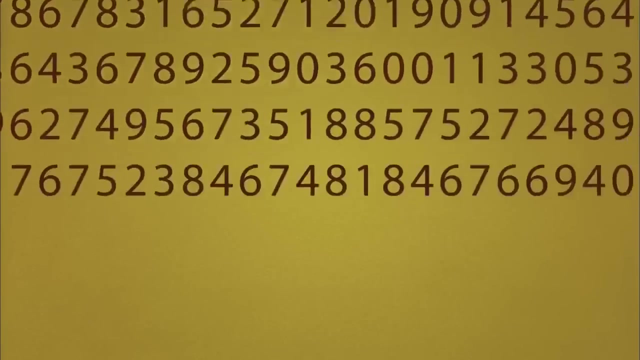 The mysterious connections between the physical world and mathematics run deep. We all know the number pi from geometry, the ratio between the circumference of a circle and its diameter, and that its decimal digits go on forever without a repeating pattern, As of 2013,. 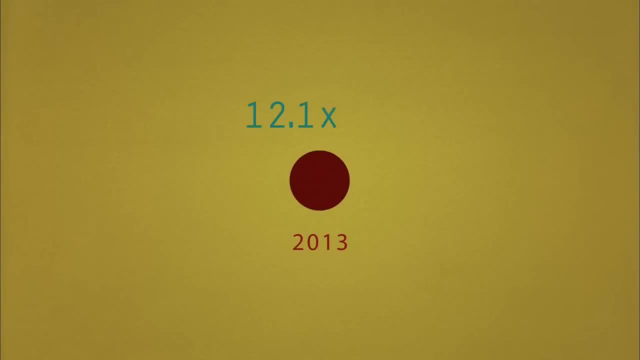 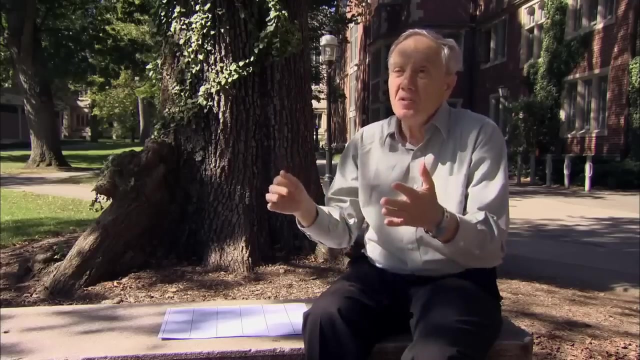 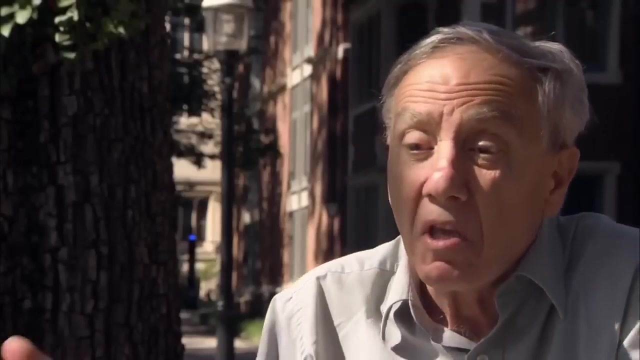 it had been calculated out to 12.1 trillion digits. But somehow pi is a whole lot more. Pi appears in a whole host of other phenomena which have, at least on the face of it, nothing to do with circles or anything. In particular it appears in probability theory quite a bit. 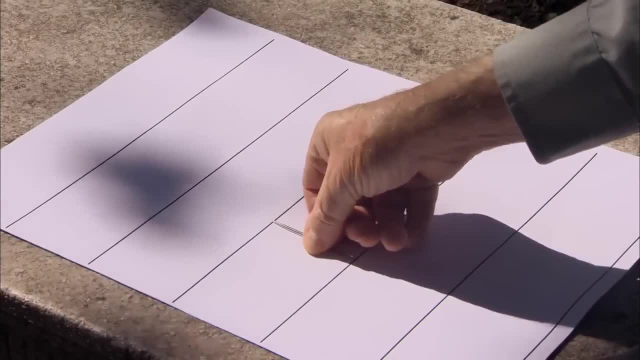 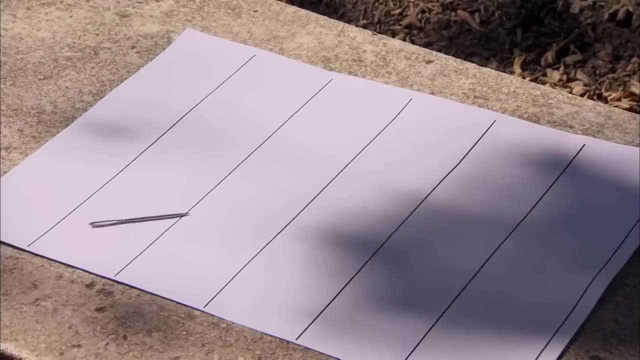 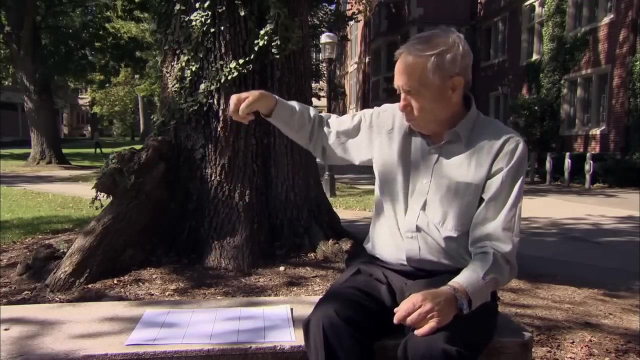 Suppose I take this needle so that the length of the needle is equal to the distance between two lines on this piece of paper, And suppose I drop this needle now on the paper. Sometimes when you drop the needle it will cut a line and sometimes it drops between the lines. 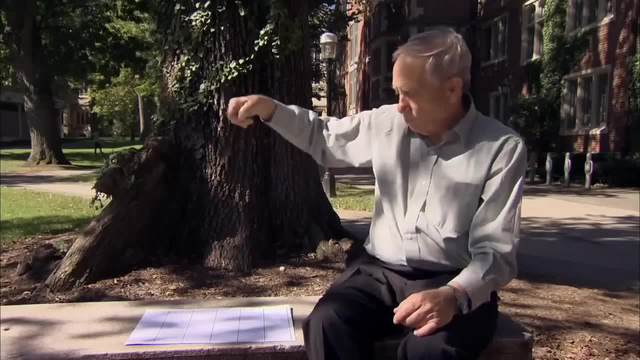 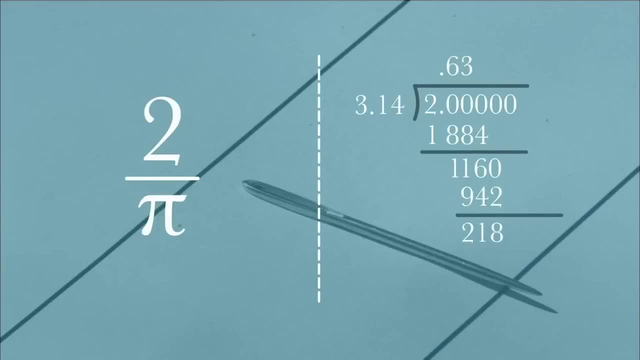 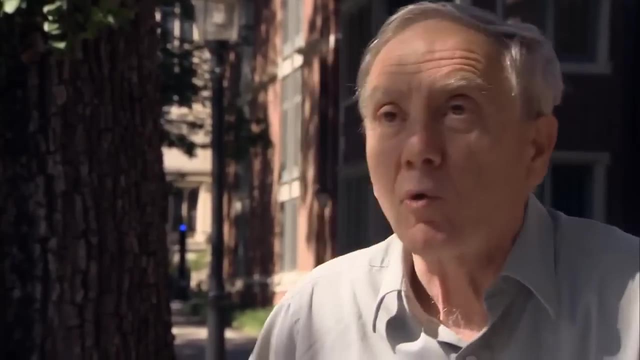 It turns out, the probability that the needle lands so it cuts a line is exactly two over pi, or about 64%. Now what that means is that, in principle, I could drop this needle millions of times. I could count the times when it crosses a line. 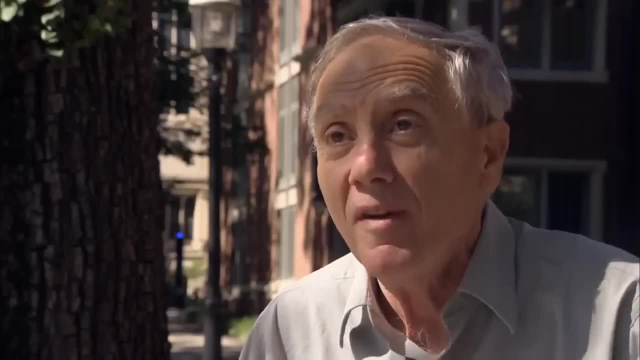 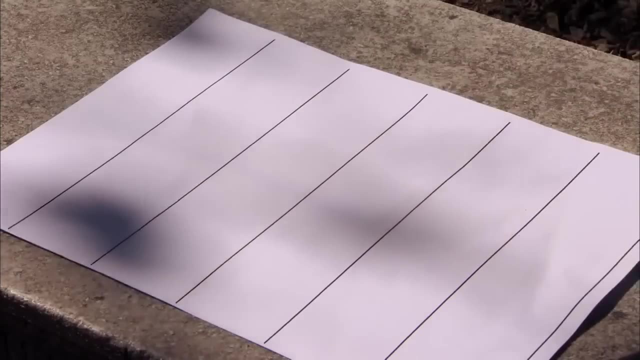 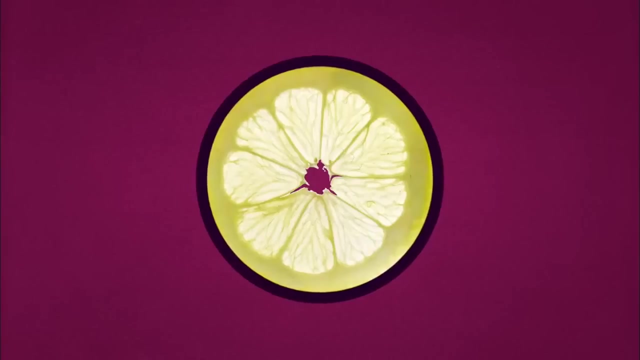 and when it doesn't cross a line. and I could actually even calculate pi, even though there are no circles here, no diameters of a circle, nothing like that. It's really amazing, Since pi relates a round object, a circle. 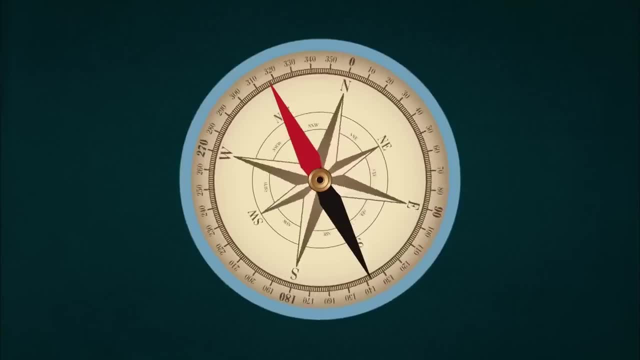 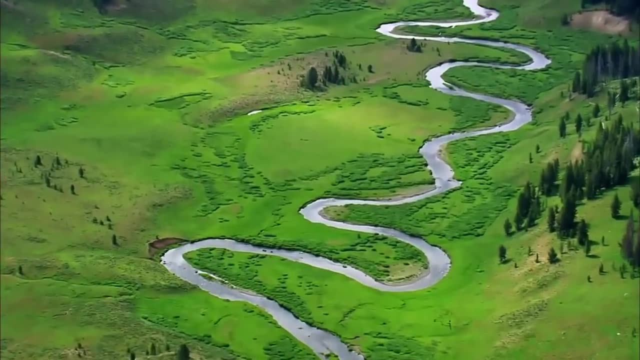 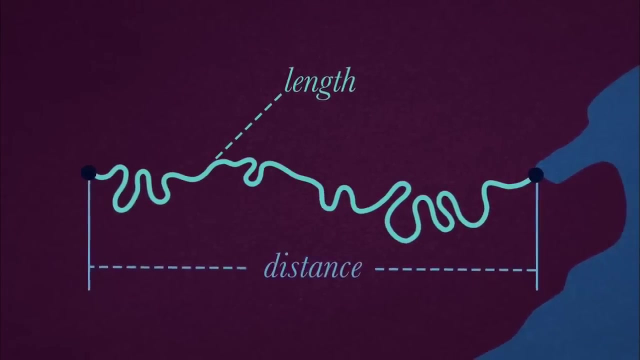 with a straight one, its diameter, it can show up in the strangest of places. Some see it in the meandering path of rivers, A river's actual length as it winds its way from its source to its mouth, compared to the direct distance, 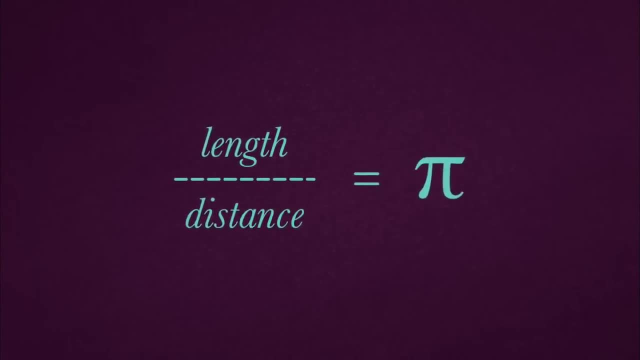 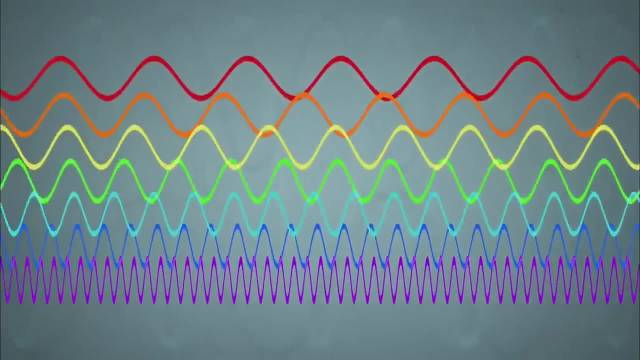 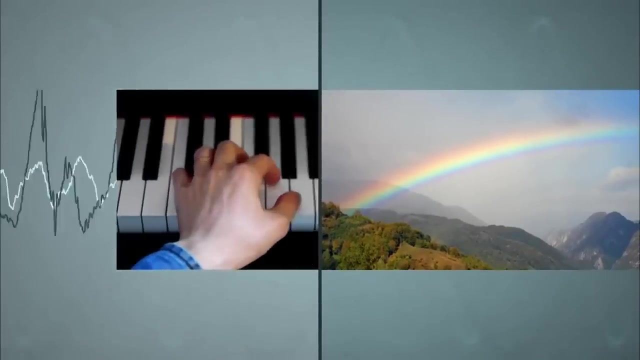 on average, seems to be about pi. Models for just about anything involving waves will have pi in them, Like those for light and sound. pi tells us which colors should appear in a rainbow and how Middle Sea should sound like, For example. pi can be heard on a piano. 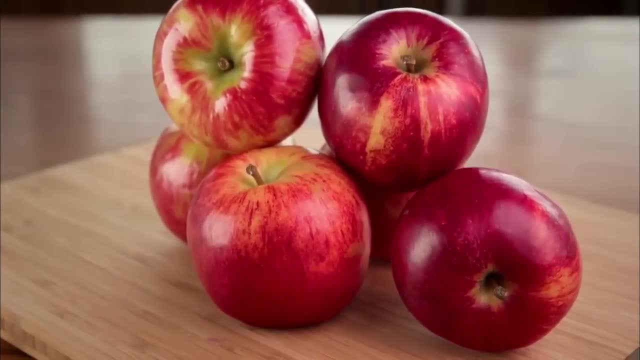 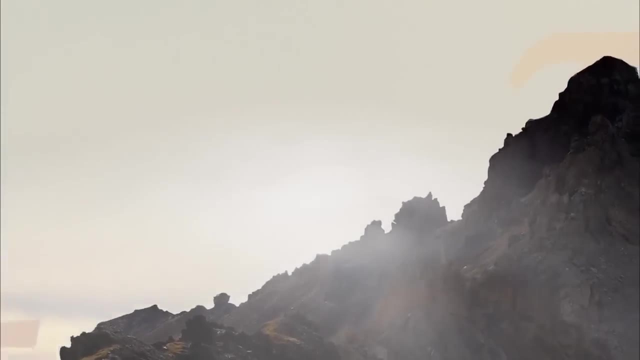 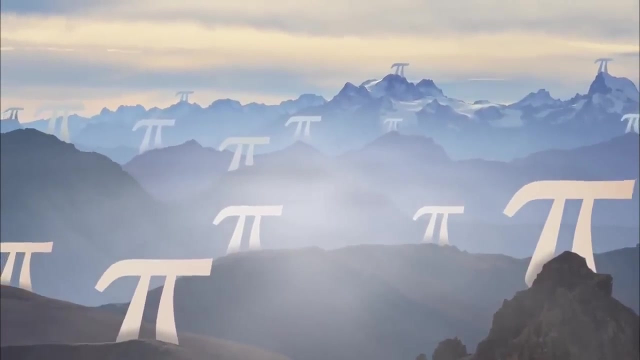 Pi shows up in apples, in the way cells grow into spherical shapes, or in the brightness of a supernova. One writer has suggested it's like seeing pi on a series of mountain peaks poking out of a fog-shrouded valley. We know there is a way. they're all connected. 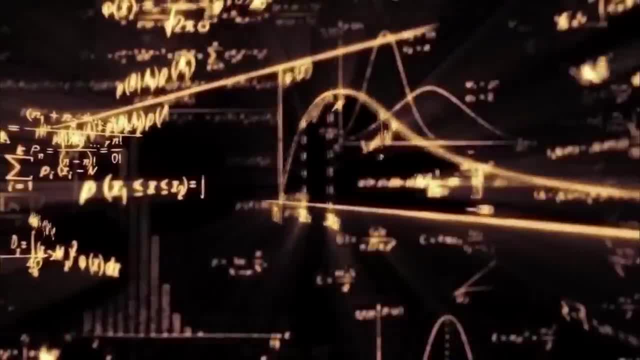 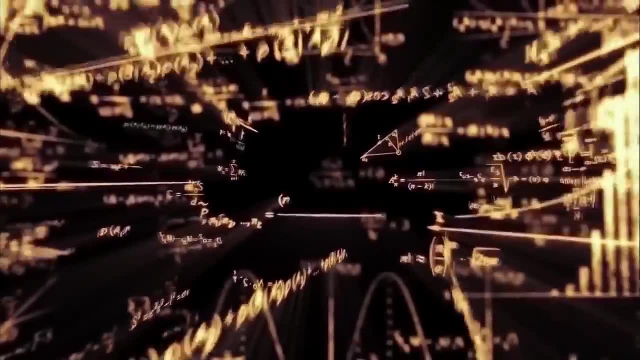 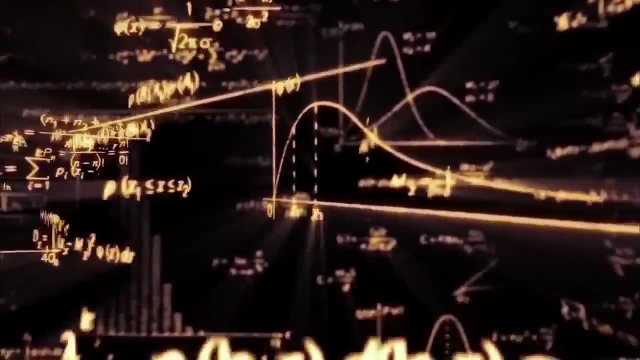 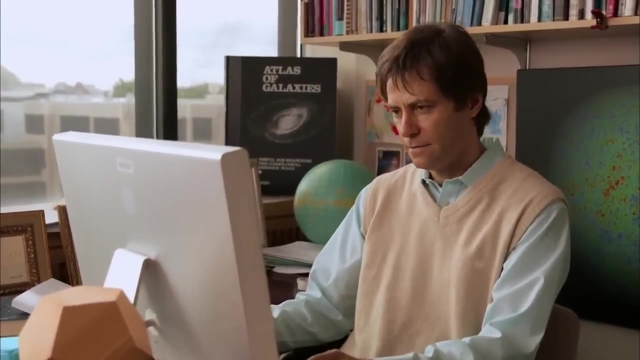 but it's not always obvious how Pi is, but one example of a vast interconnected web of mathematics that seems to reveal an often hidden and deep order to our world. Physicist Max Tegmark from MIT thinks he knows why He sees similarities between our world. 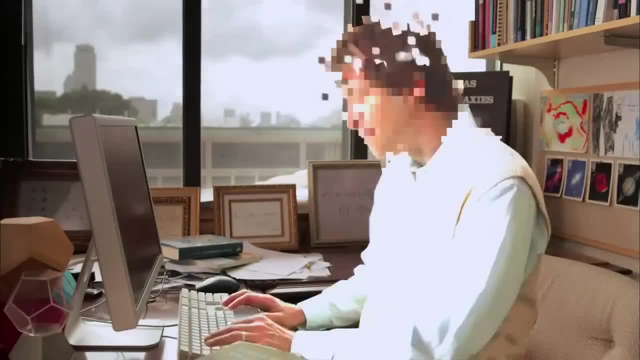 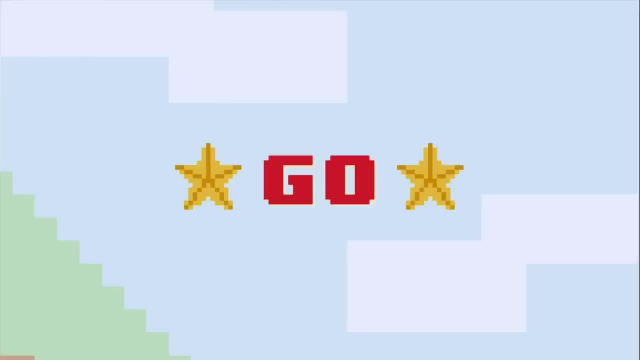 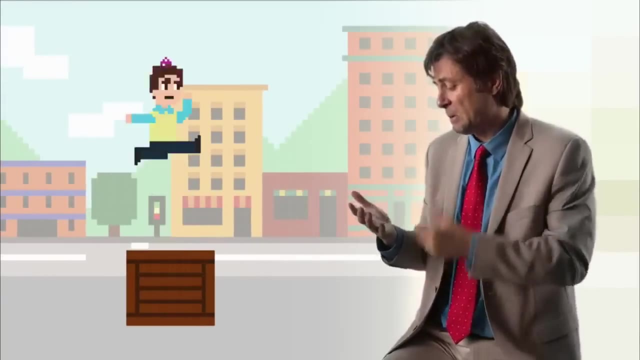 and that of a computer game. If I were a character in a computer game that were so advanced that I were actually conscious and I started exploring my video game world, it would actually feel to me like it was made of real, solid objects, made of physical stuff. 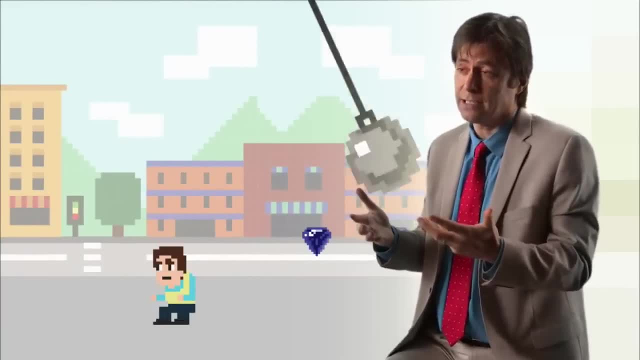 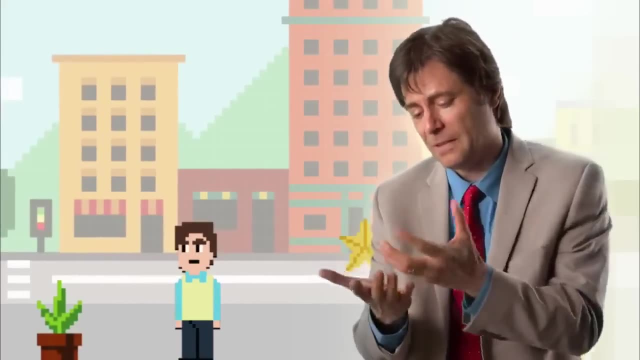 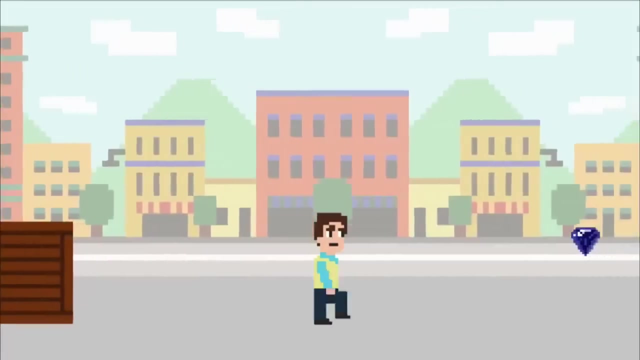 Yet if I started studying, as the curious physicist that I am, the properties of this stuff, the equations by which things move and the equations that give the stuff its properties, I would discover eventually that all these properties were mathematical, The mathematical properties that the programmer 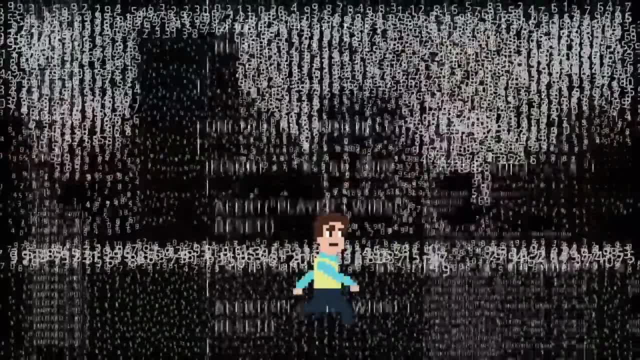 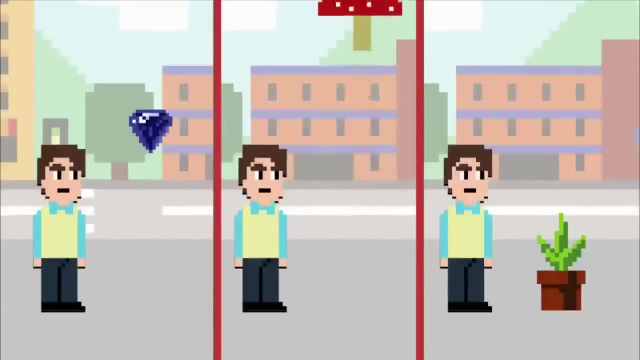 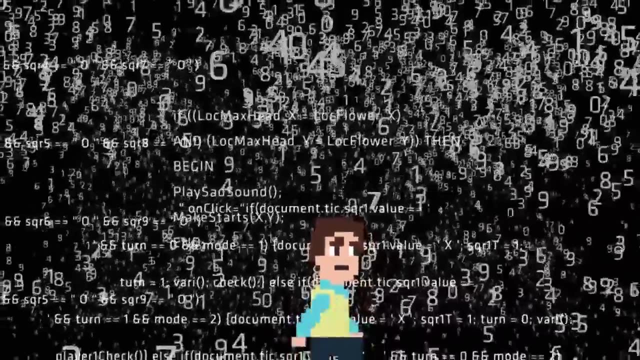 had actually put into the software. that describes everything. The laws of physics in a game, like how an object floats, bounces or crashes, are only mathematical rules created by a programmer. Ultimately, the entire universe of a computer game is just numbers and equations. 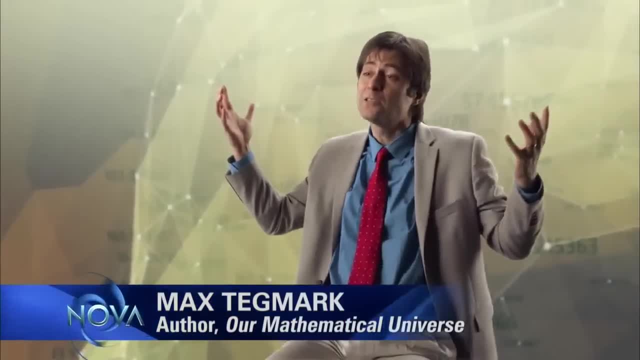 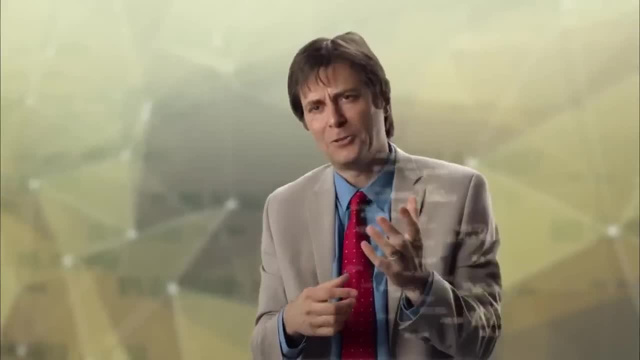 That's exactly what I perceive in this reality too, as a physicist: that the closer I look at things that seem non-mathematical, like my arm here and my hand, the more mathematical it turns out to be. Could it be that our world also, then, is really? 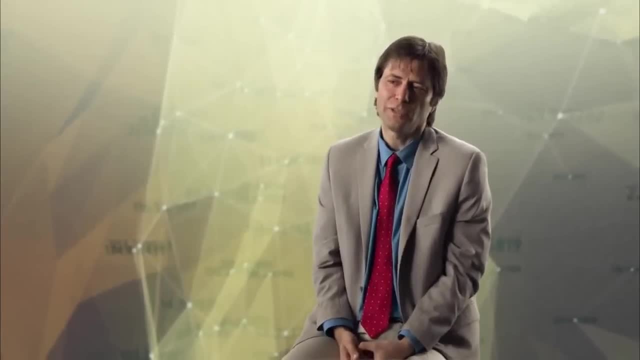 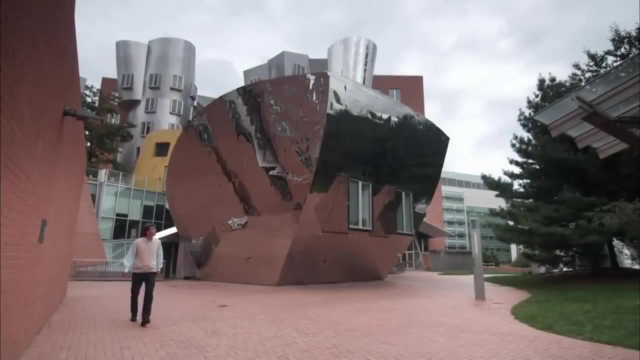 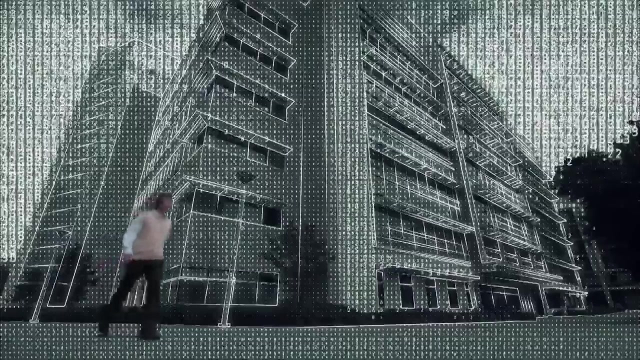 just as mathematical as the computer game reality To Max. the software world of a game isn't that different from the physical world we live in. He thinks that mathematics works so well to describe reality because, ultimately, mathematics is all that it is, There's nothing else. 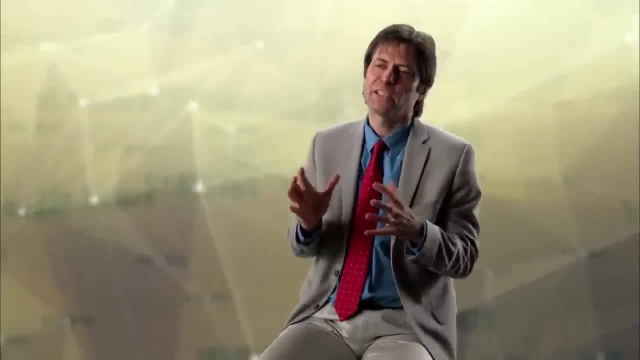 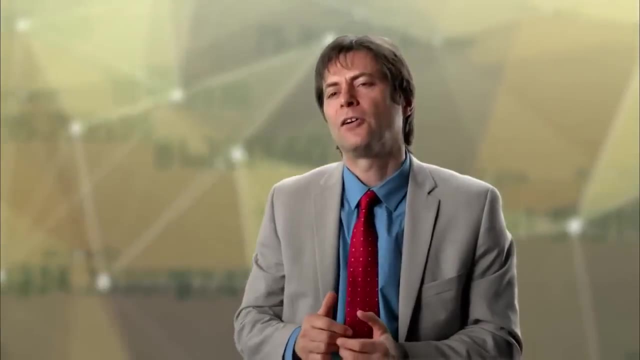 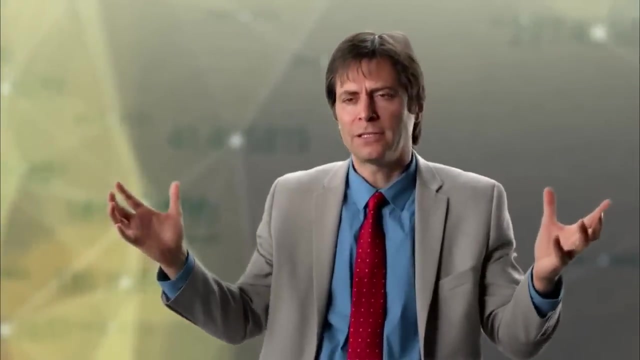 Many of my physics colleagues will say that mathematics describes our physical reality, at least in some approximate sense. I go further and argue that it actually is our physical reality, because I'm arguing that our physical world doesn't just have some mathematical properties, but it has only mathematical properties. 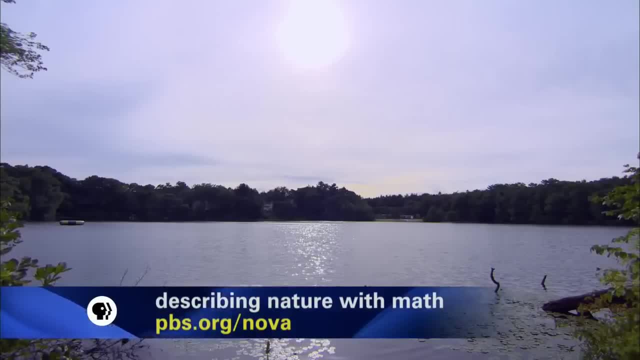 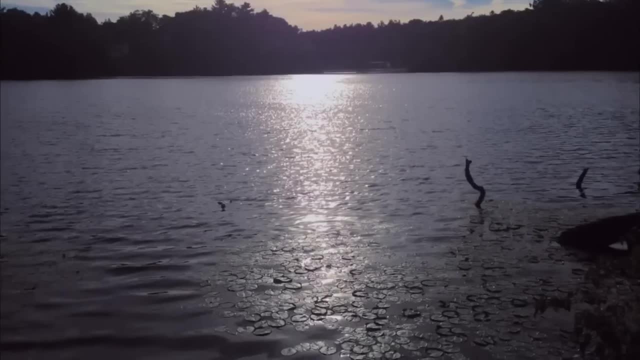 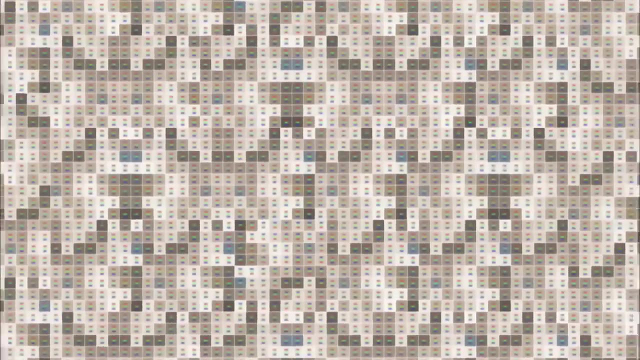 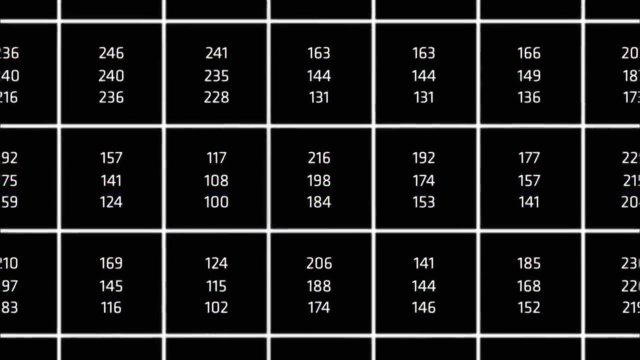 Our physical reality is a bit like a digital photograph. according to Max, The photo looks like the pond, but as we move in closer and closer we can see. it is really a field of pixels, Each represented by three numbers that specify the amount of red, green and blue. 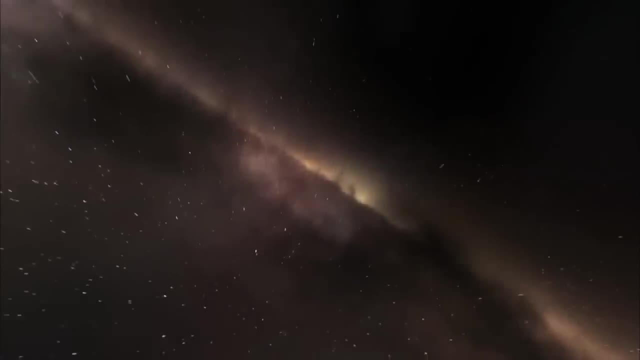 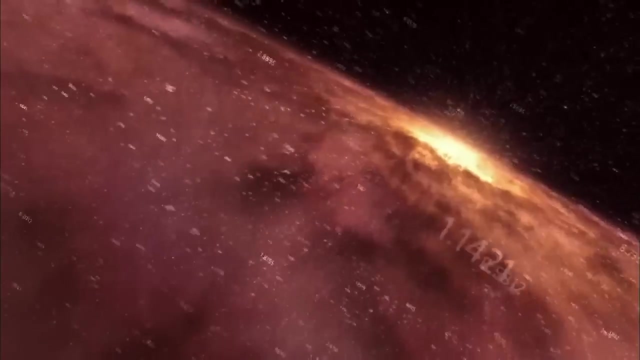 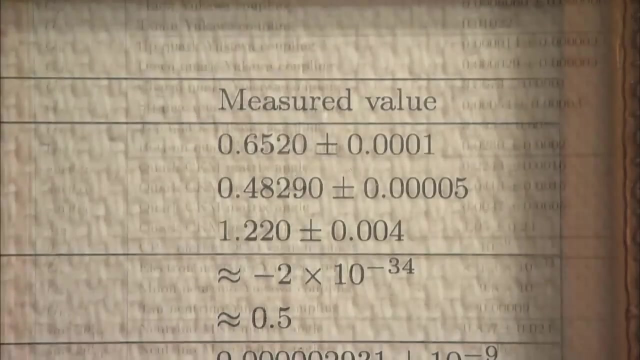 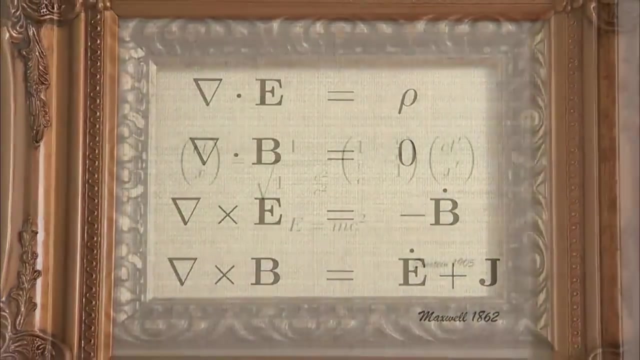 While the universe is vast in its size and complexity, requiring an unbelievably large collection of numbers to describe it, Max sees its underlying mathematical structure as surprisingly simple: It's just 32 numbers, constants like the masses of elementary particles, along with a handful of mathematical equations. 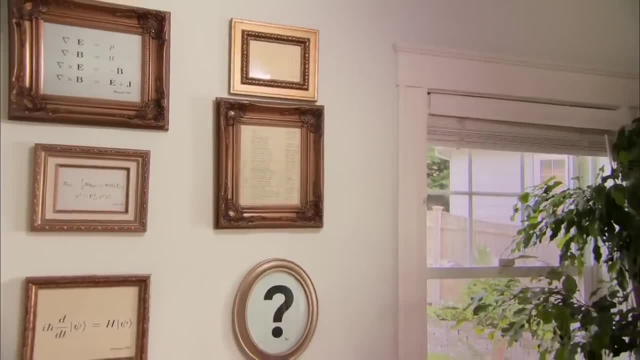 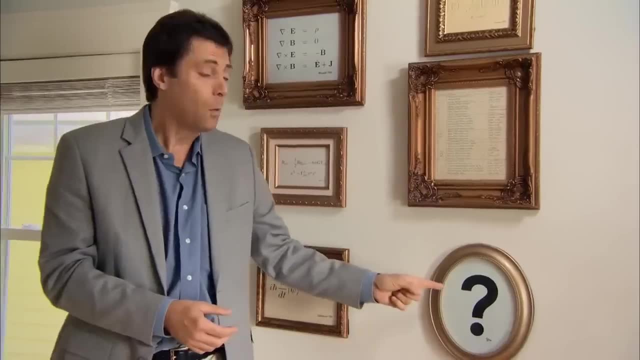 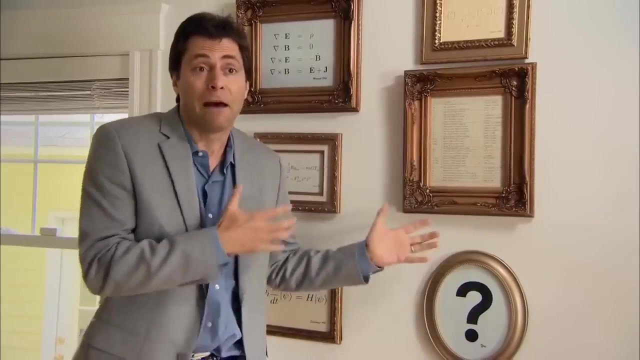 the fundamental laws of physics, And it all fits on a wall, though there are still some questions, But even though we don't know what exactly is going to go here, I'm really confident that what will go here will be mathematical equations, that everything is ultimately mathematical. 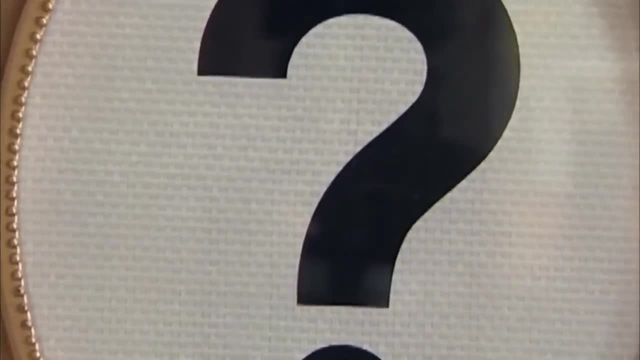 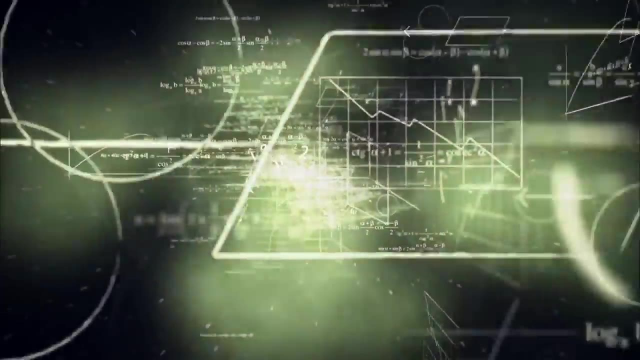 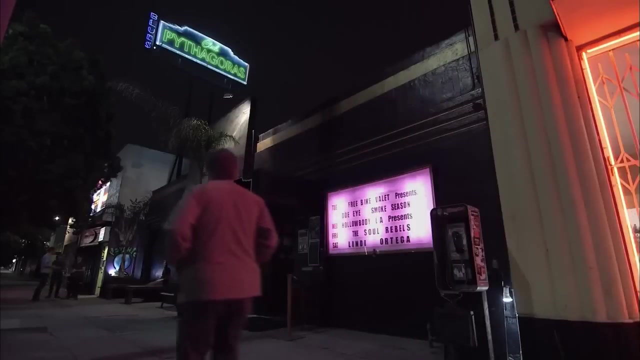 Max Tegmark's matrix-like view that mathematics doesn't just describe reality but is its essence may sound radical, But it has deep roots in history Going back to ancient Greece, to the time of the philosopher and mystic Pythagoras. 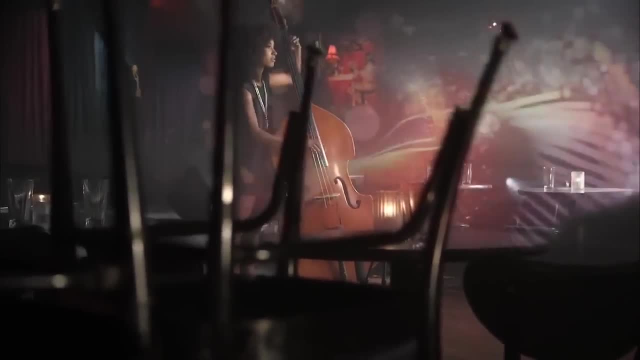 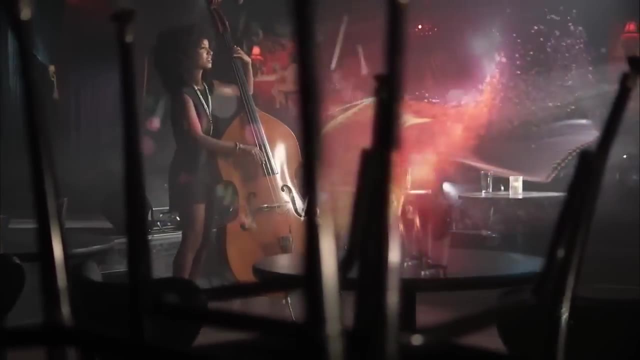 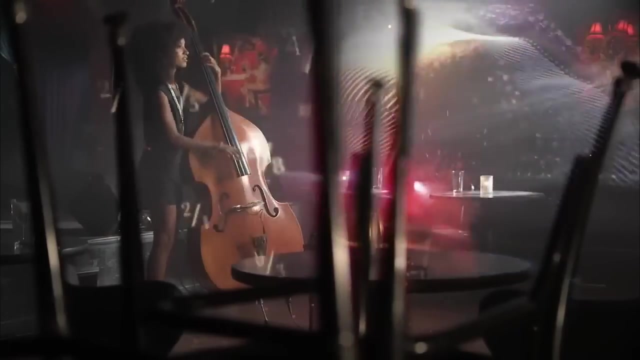 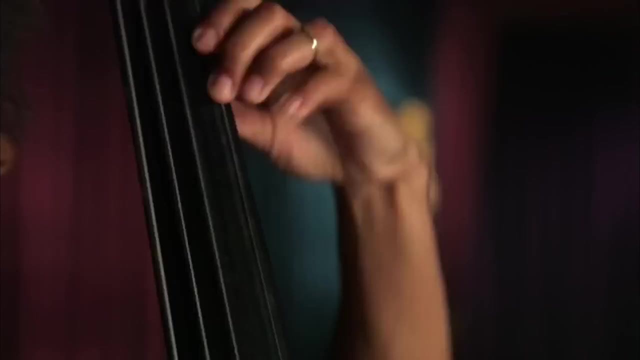 Stories say he explored the affinity between mathematics and music, a relationship that was so strong it resonates to this day in the work of Esperanza Spalding, an acclaimed jazz musician who studied music theory and sees its parallel in mathematics. I love the experience of math. 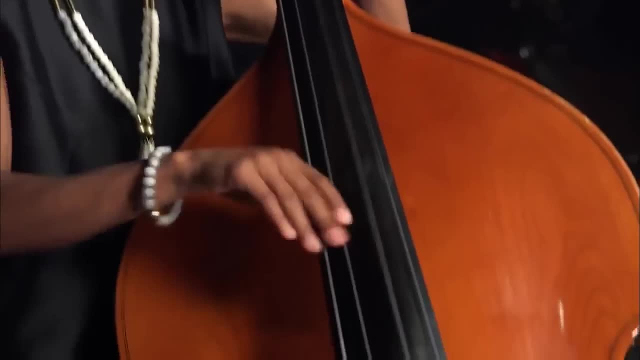 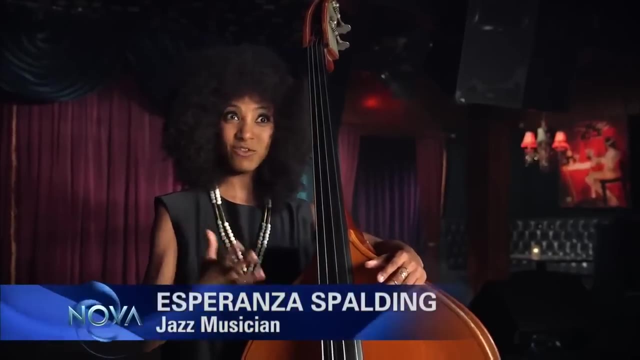 The part that I enjoy about math I get to experience through music too. At the beginning you're studying all the little equations, but you get to have this very visceral relationship with the product of those equations, which is sound and music and harmony and distance. 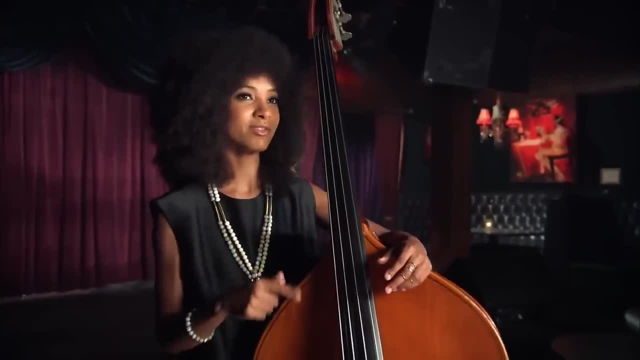 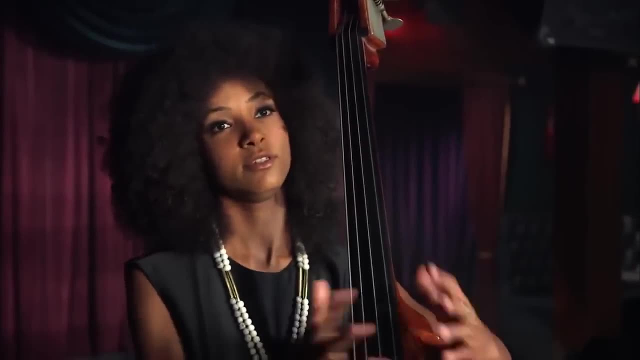 and all that good stuff. So I'm much better at music than at math, but I love math with a passion. They're both just as much work. They both you have to study it off Your head off, Study your head off. 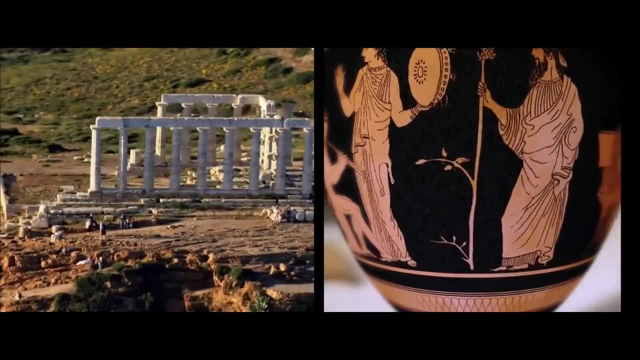 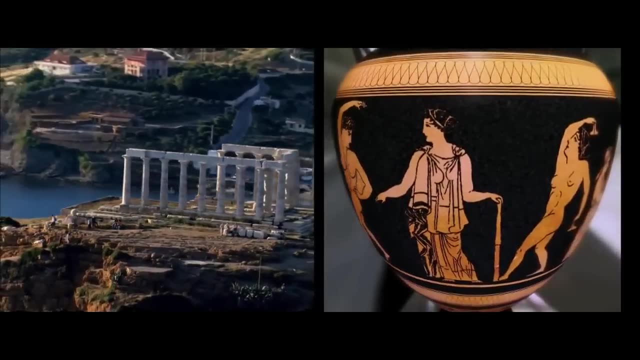 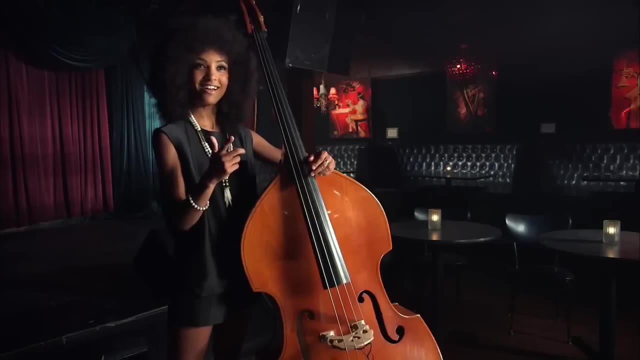 The ancient Greeks found three relationships between notes especially pleasing. Now we call them an octave, a fifth and a fourth. An octave is easy to remember because it's the first two notes of somewhere over the rainbow. La la, That's an octave somewhere. 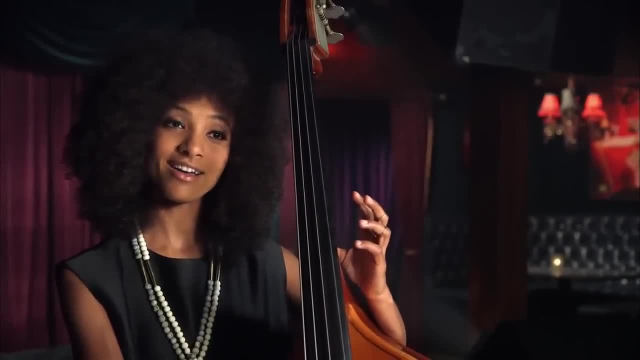 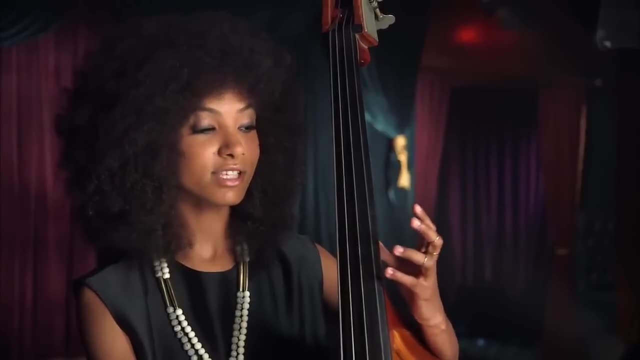 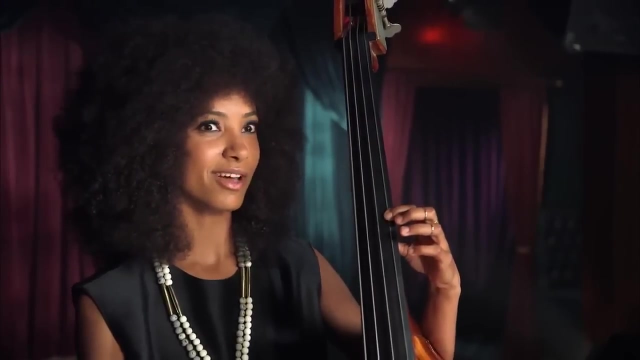 A fifth sounds like this: La la, Or the first two notes of twinkle, twinkle little star. And a fourth sounds like la la. You can think of it as the first two notes of here comes the bride In the sixth century BCE. 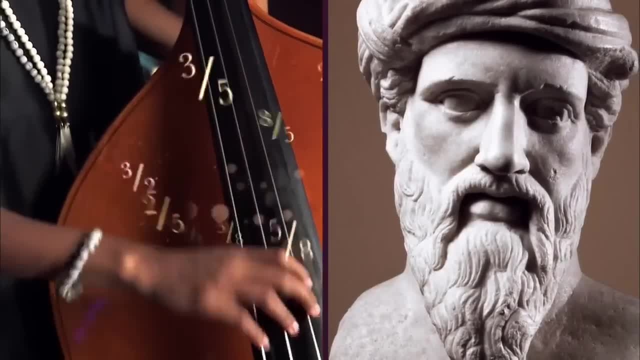 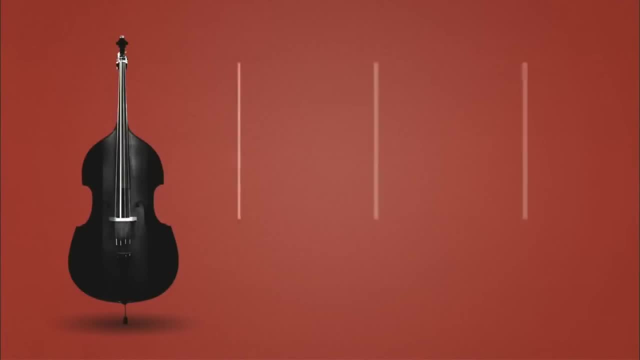 the Greek philosopher Pythagoras is said to have discovered that those beautiful musical relationships were also beautiful mathematical relationships. by measuring the lengths of the vibrating strings. In an octave, the string lengths create a ratio of two to one. In a fifth, the ratio is three to two. 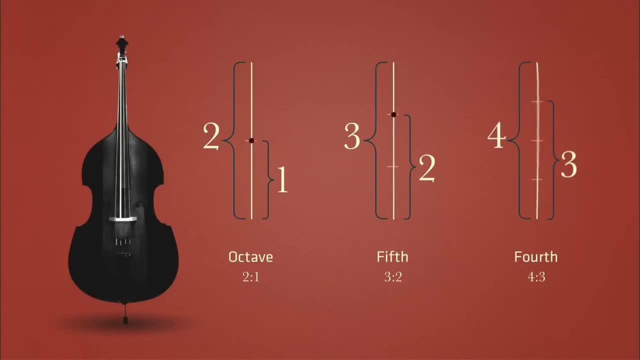 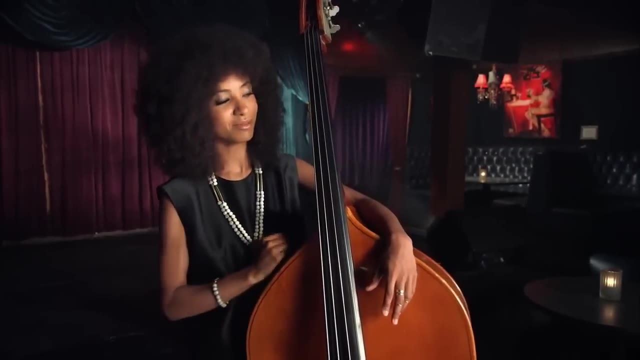 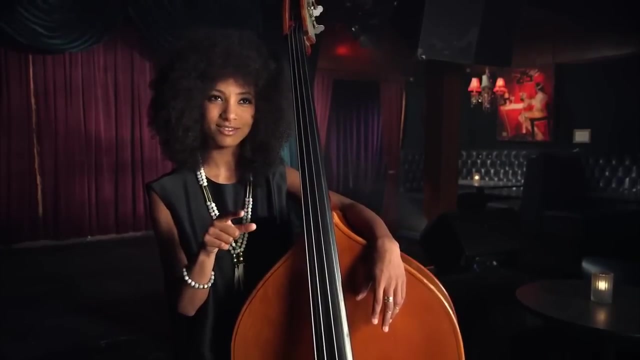 And in a fourth- it is four to three- Seeing a common pattern throughout sound. that could be a big eye-opener of saying, well, if this exists in sound and if it's true universally through all sounds, this ratio could exist universally. 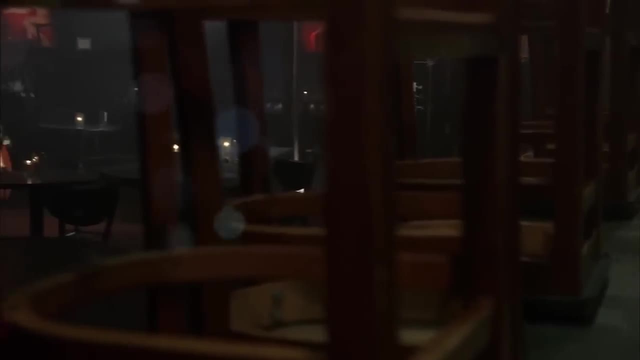 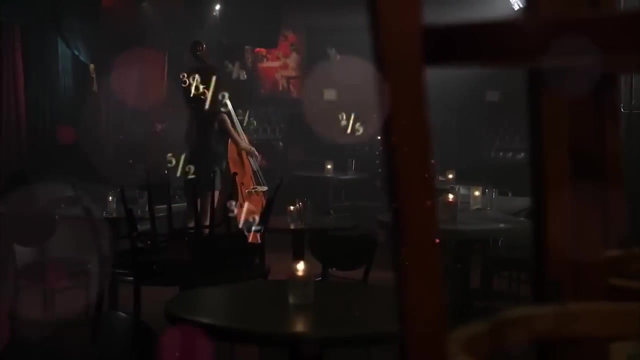 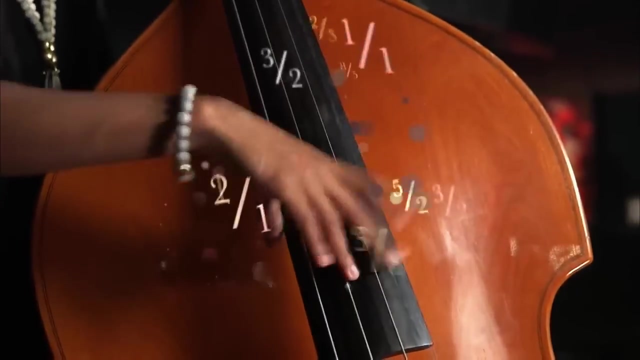 everywhere. right, And doesn't it? Pythagoreans worship the idea of numbers. The fact that simple ratios produced harmonious sounds was proof of a hidden order in the natural world, And that order was made of numbers. a profound insight that mathematicians and scientists 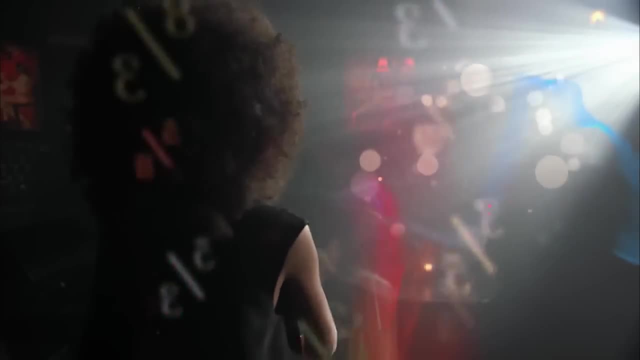 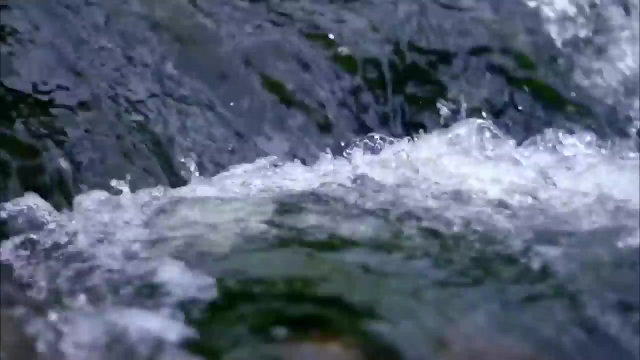 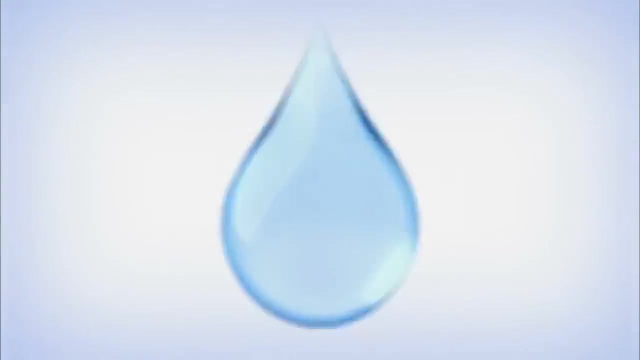 continue to explore to this day. In fact, there are plenty of other physical phenomena that follow simple ratios, From the two to one ratio of hydrogen atoms to oxygen atoms in water, to the number of times the moon orbits the Earth compared to its own rotation. 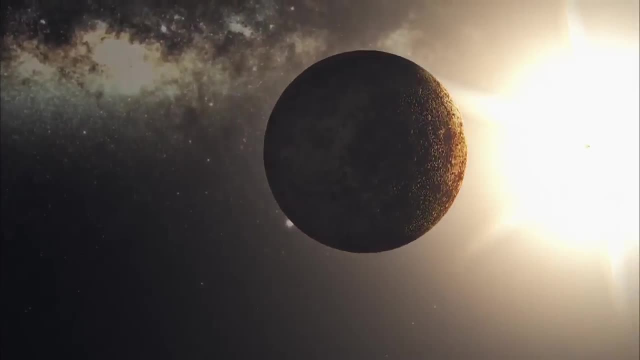 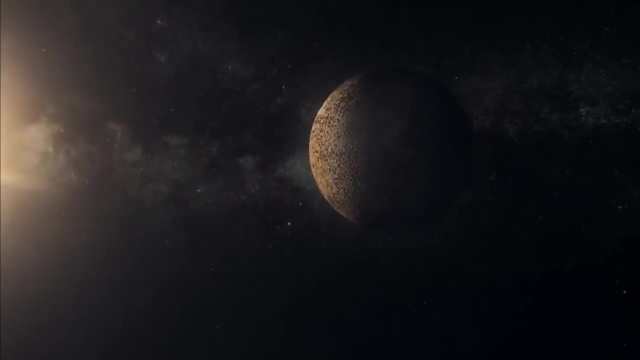 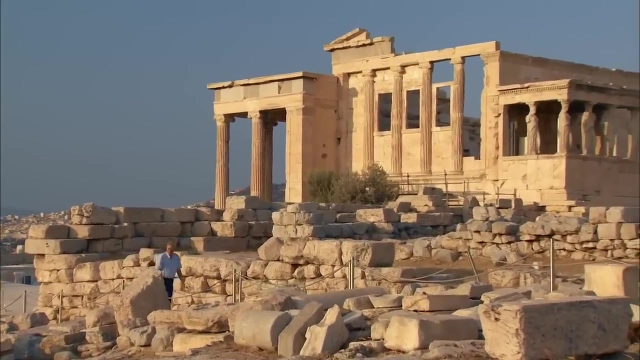 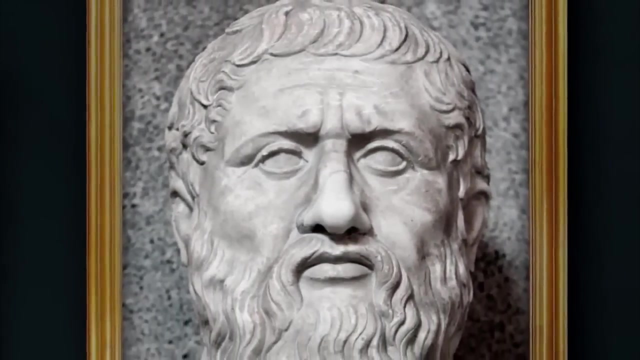 one to one, Or that Mercury rotates exactly three times, when it orbits the sun twice. a three to two ratio In ancient Greece, Pythagoras and his followers had a profound effect on another Greek philosopher, Plato, whose ideas also resonate to this day. 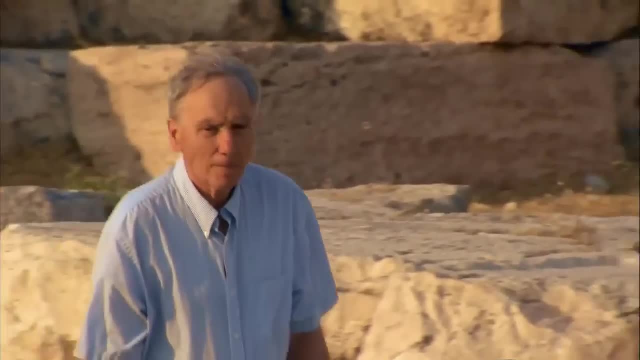 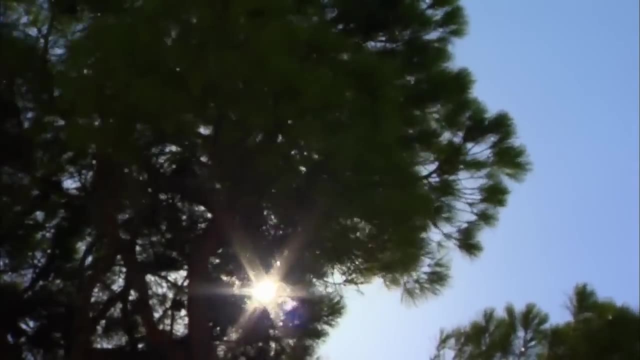 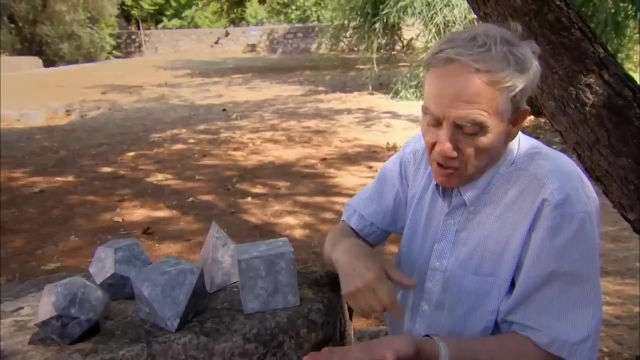 especially among mathematicians. Plato believed that geometry and mathematics exist in their own ideal world. So when we draw a circle on a piece of paper, this is not the real circle. The real circle is in that world and this is just an approximation. 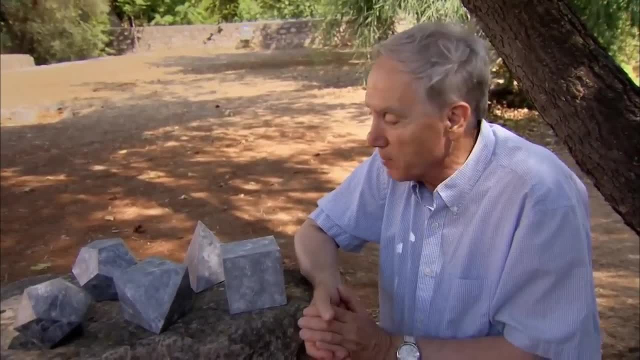 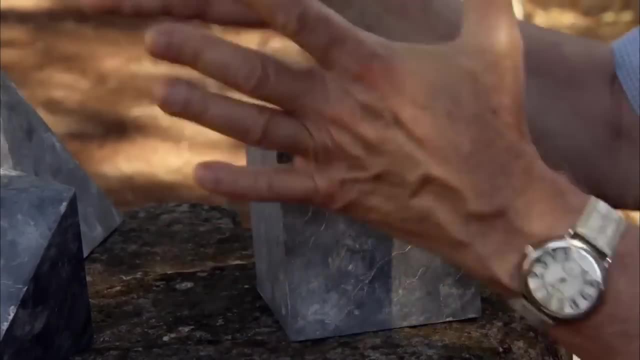 of that real circle, The same with all other shapes, And Plato liked very much these five solids, the platonic solids we call them today, And he assigned each one of them to one of the elements that formed the world as he saw it. 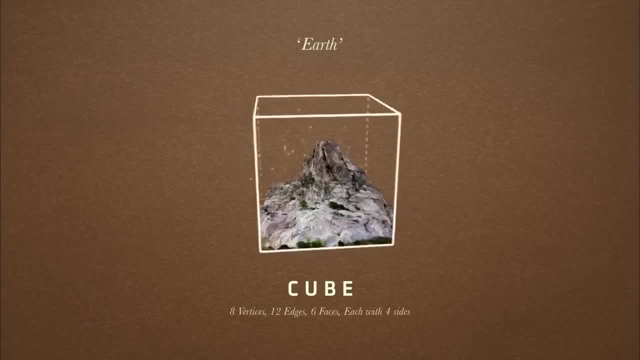 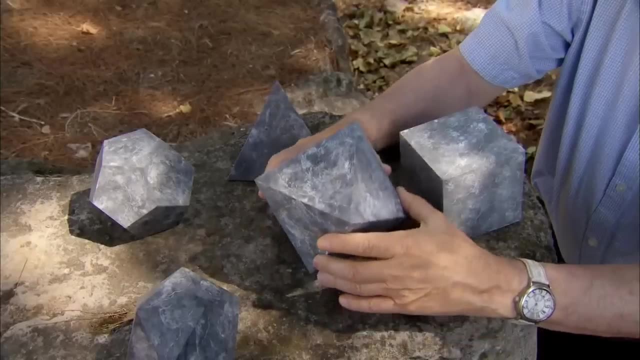 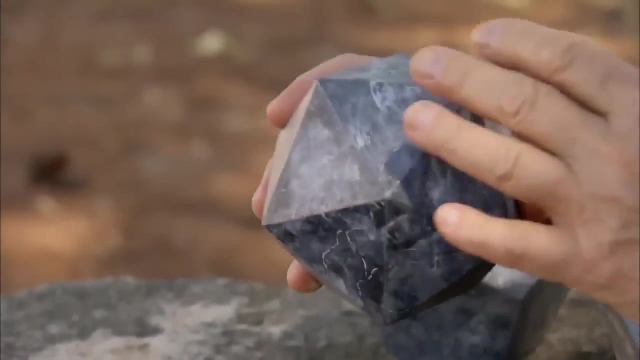 The stable cube was Earth, The tetrahedron with its pointy corners was fire, The mobile-looking octahedron, Plato, thought of as air And the 20-sided icosahedron was water, And finally the dodecahedron. 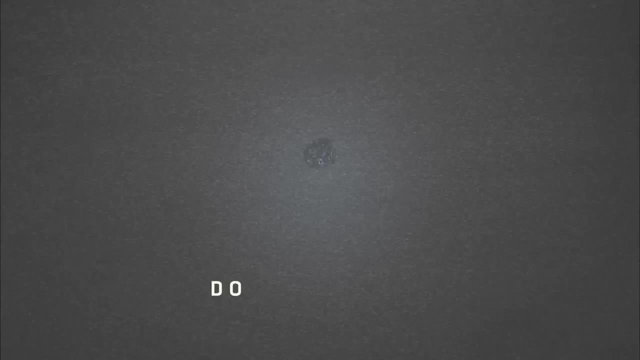 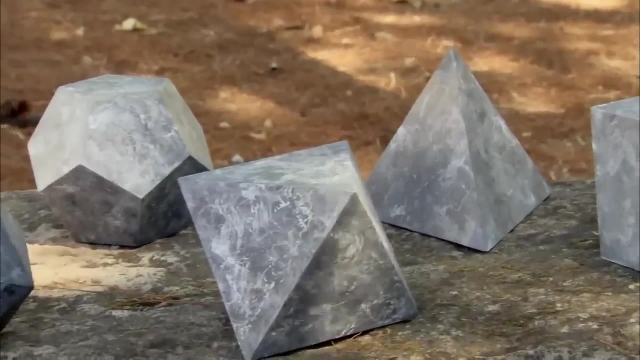 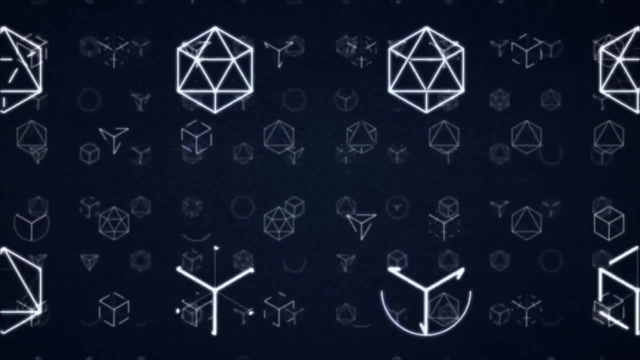 this was the thing that signified: the cosmos as a whole. So Plato's mathematical forms were the ideal version of the world around us, and they existed in their own realm. And, however bizarre that may sound, that mathematics exists in its own world. 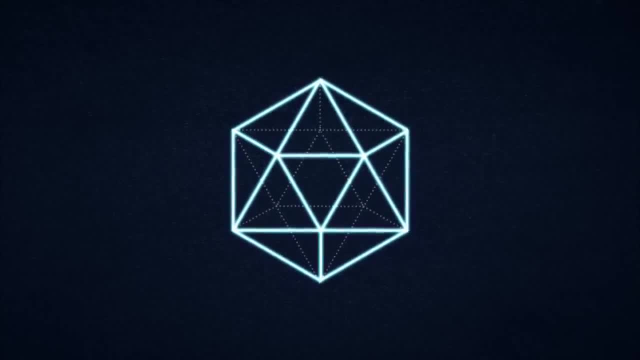 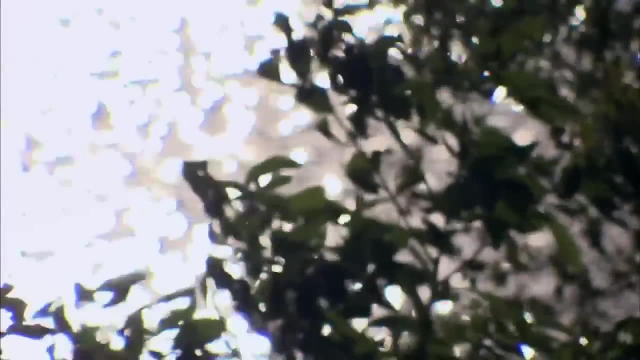 shaping the world. we see, It's an idea that, to this day, many mathematicians and scientists can relate to, The sense they have when they're doing math: that they're just uncovering something that's already out there. I feel quite strongly that mathematics is discovered. 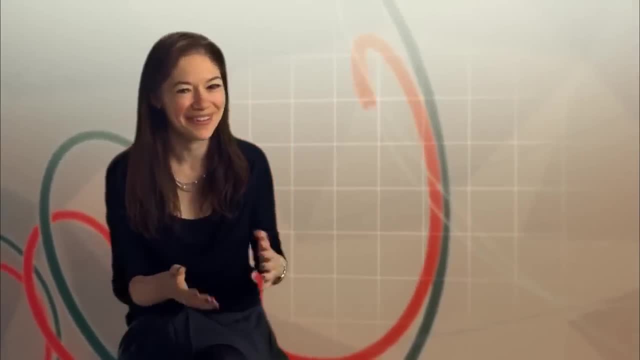 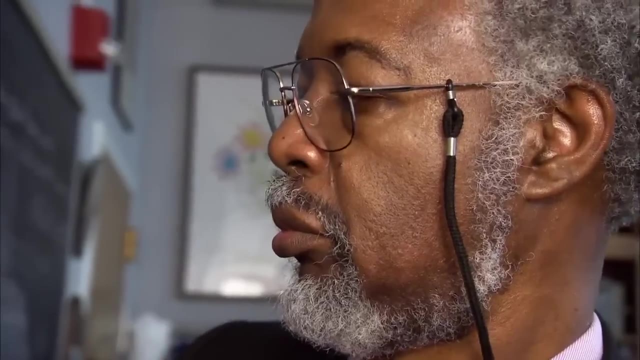 In my work as a mathematician it always feels to me there is a thing out there and I'm kind of trying to find it and understand it and touch it. As someone who actually has had the pleasure of making new mathematics, it feels like there's something there. 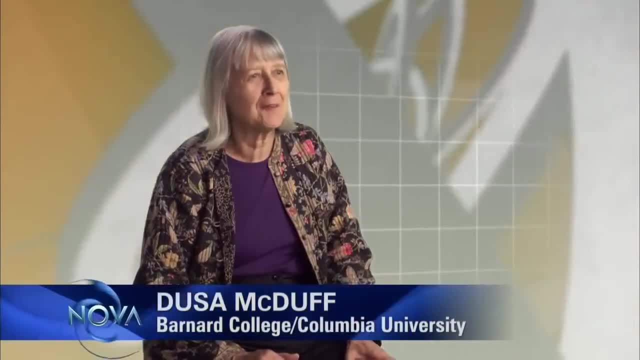 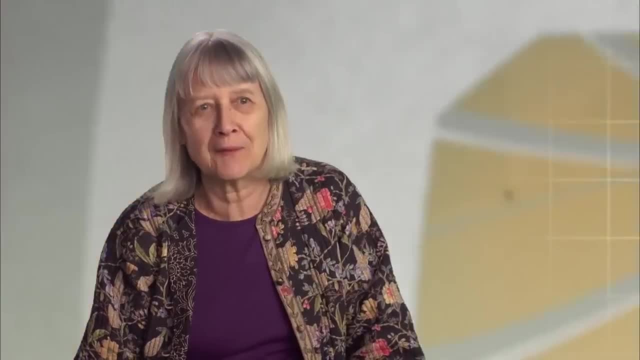 before you get to it. If I have to choose, I think it's more discovered than invented, because I think there's a reality to what we study in mathematics. When we do good mathematics, we're discovering something about the way our minds work. 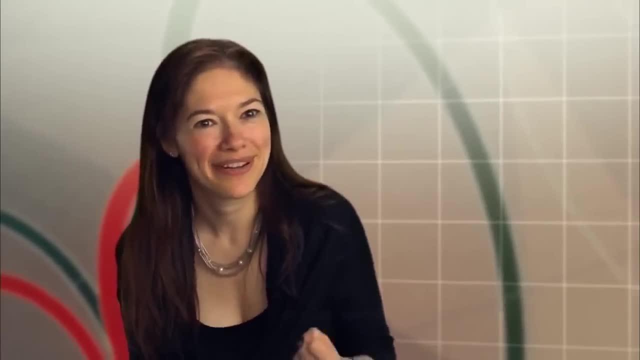 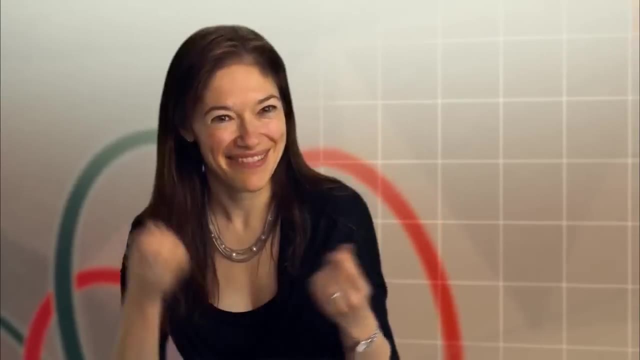 in interaction with the world. Well, I know that because that's what I do. I come to my office, I sit down in front of my whiteboard and I try and understand that thing that's out there. And every now and then, 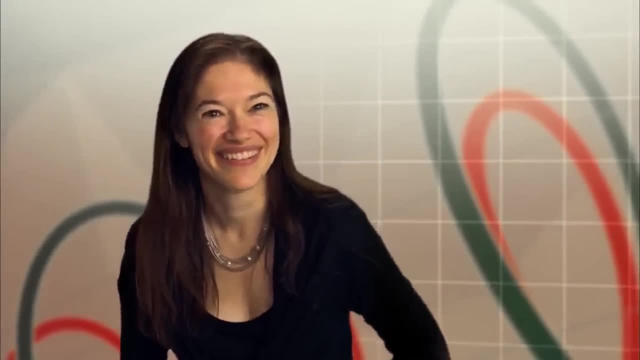 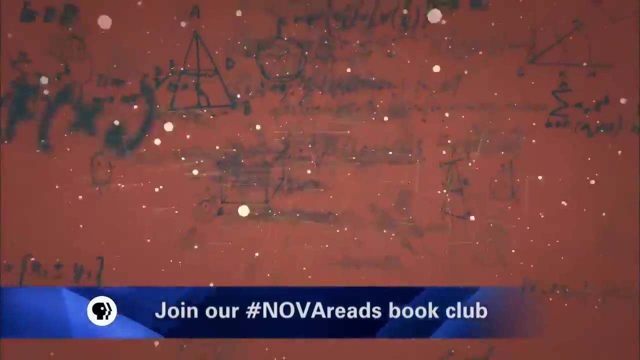 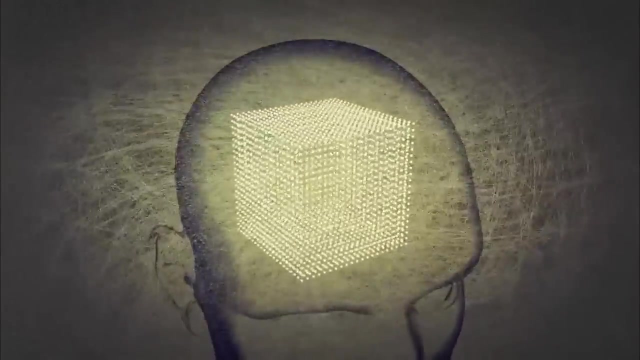 I'm discovering a new bit of it. That's exactly what it feels like To many mathematicians. it feels like math is discovered rather than invented. But is that just a feeling? Could it be that mathematics is purely a product of the human brain? 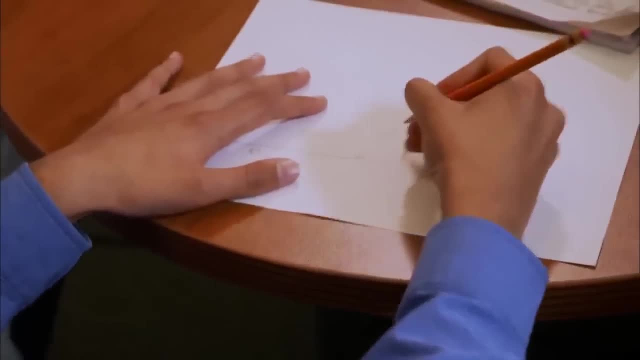 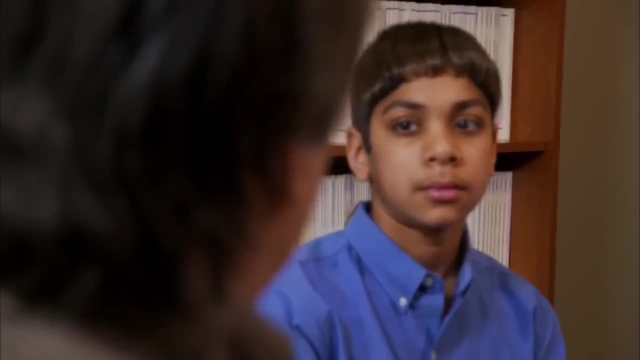 Meet Shyam, a bona fide math whiz. 800 on the SAT math, That's pretty good, And you took it when you were how old? 11. 11. Wow, that's like a perfect score. Where does Shyam's math genius come from? 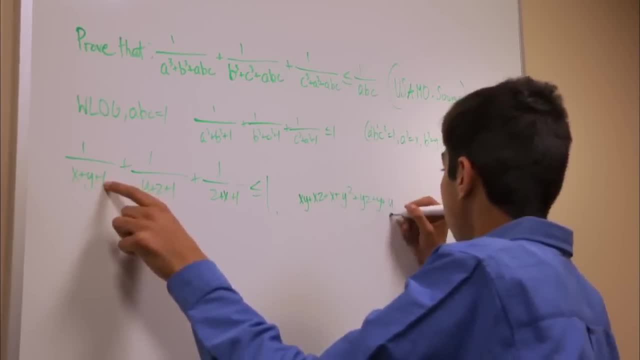 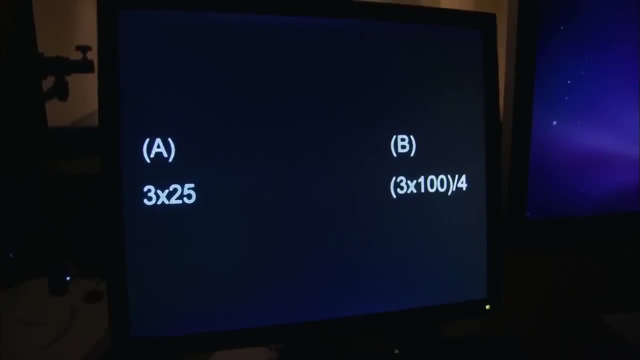 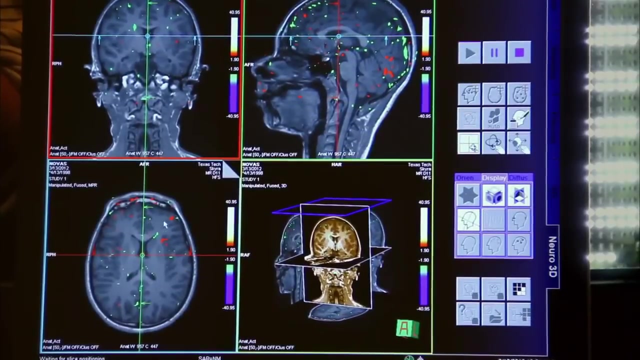 It turns out, we can pinpoint it and it's all in his head. Using fMRI, scientists can scan Shyam's brain as he answers math questions to see which parts of the brain receive more blood, a sign they are hard at work. 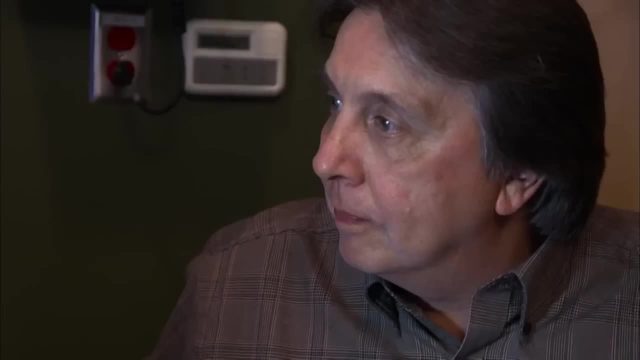 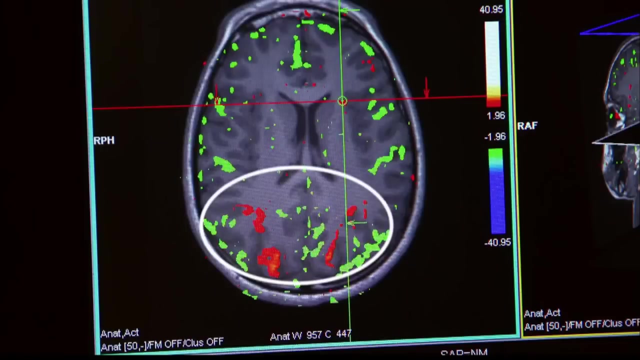 All right, Shyam, we'll start right now. okay, buddy? In images of Shyam's brain, the parietal lobes glow- an especially bright crimson. He is relying on parietal areas to determine these mathematical relationships. 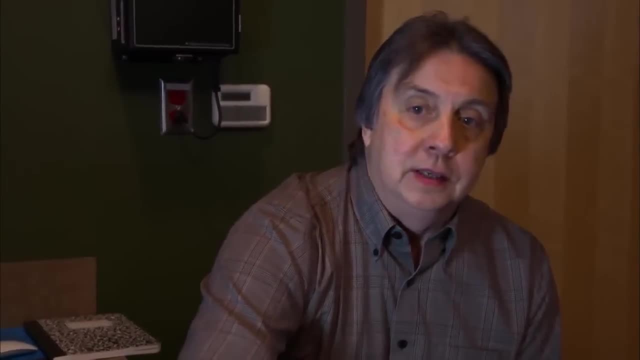 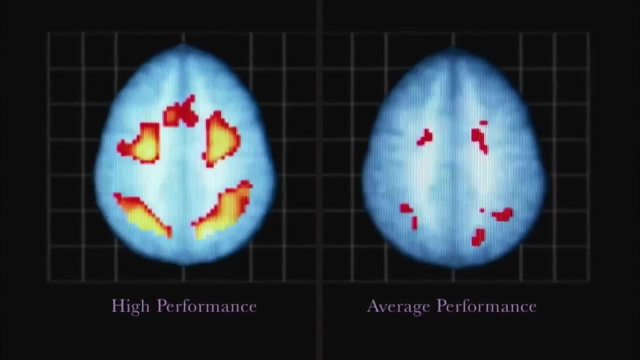 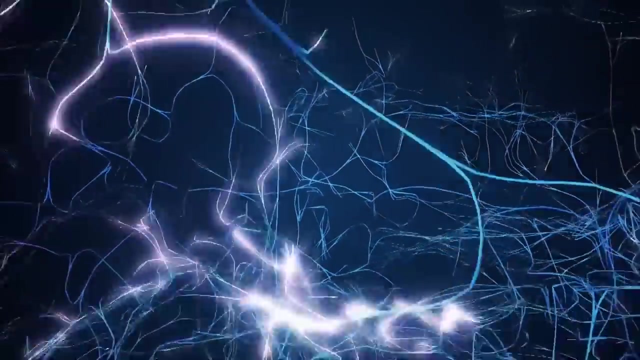 That's characteristic of lots of math-gifted types. In tests similar to Shyam's, kids who exhibit high math performance have five to six times more neuron activation than average kids in these brain regions. But is that the reason that Shyam's brain is so weak? 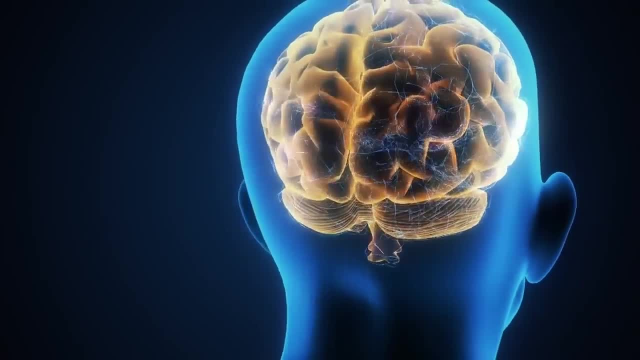 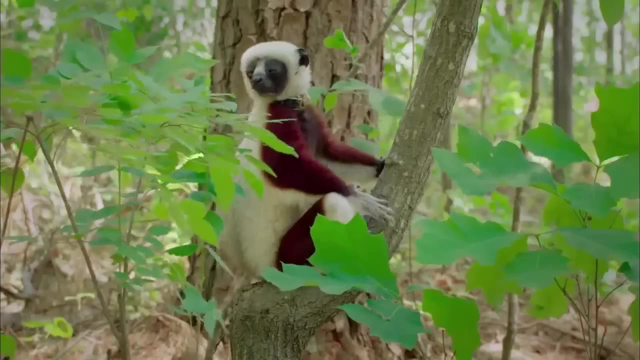 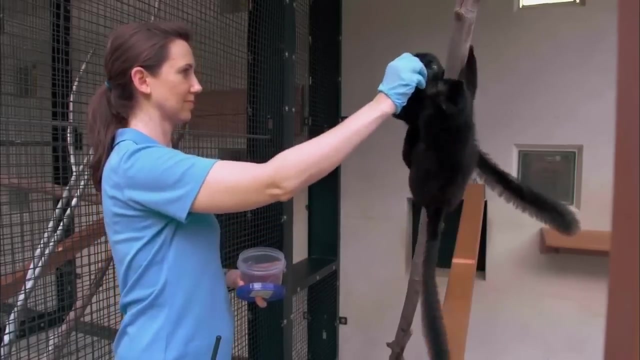 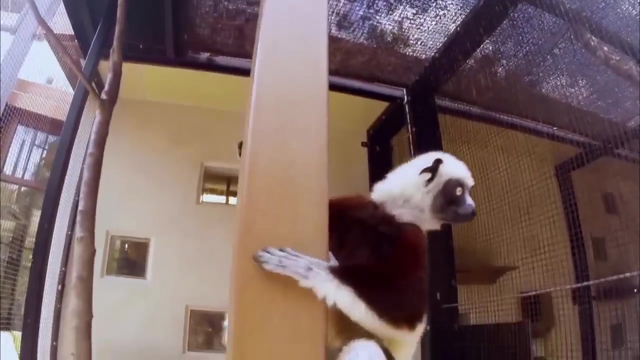 But is that the result of teaching an intense practice, Or are the foundations of math built into our brains? Scientists are looking for the answer here at the Duke University Lemur Center, a 70-acre sanctuary in North Carolina, the largest one for rare and endangered lemurs in the world. 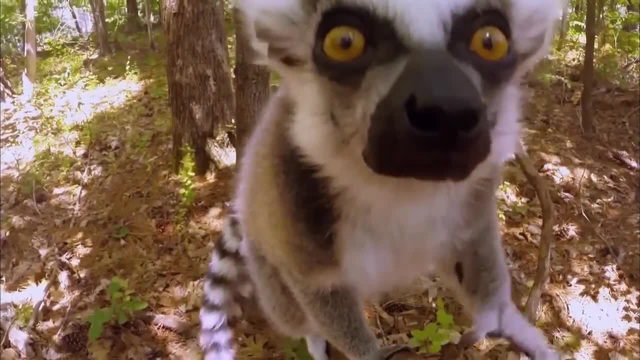 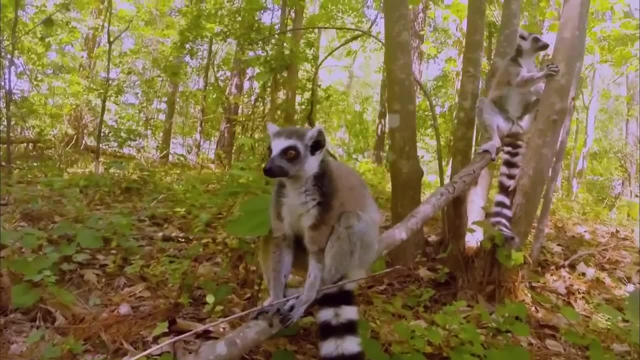 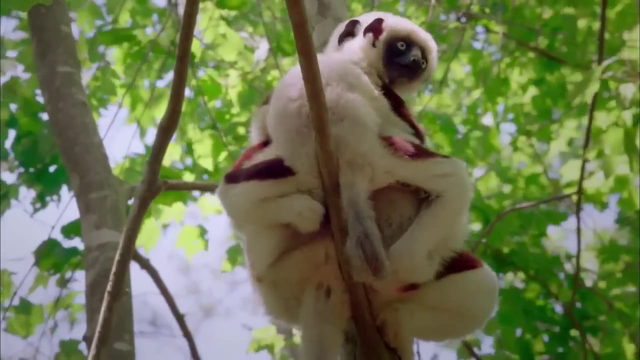 Like all primates, lemurs are related to humans through a common ancestor that lived as many as 65 million years ago. Scientists believe lemurs share many characteristics with those earliest primates, making them a window, though a blurry one, into our ancient past. 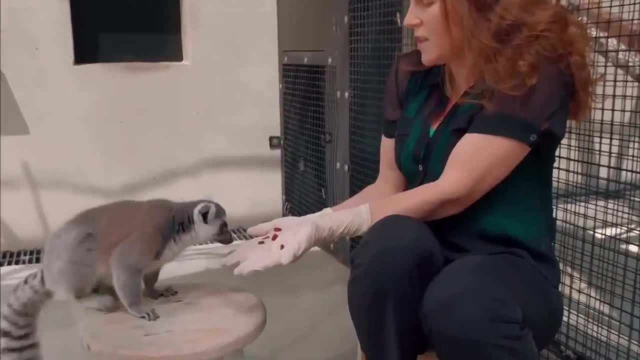 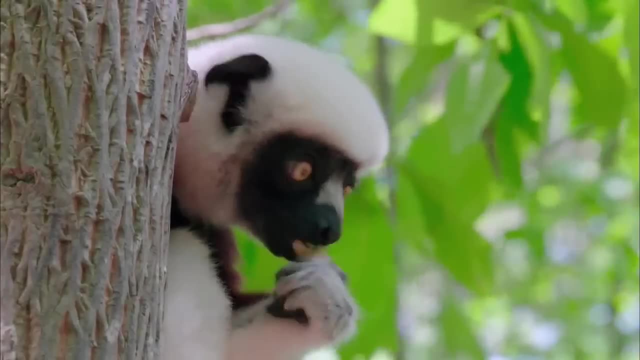 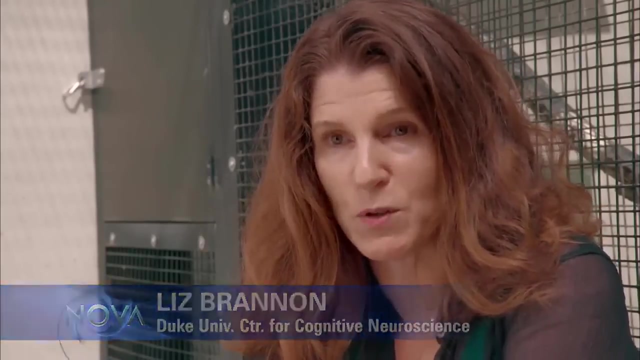 Got a choice here, Terrys, Come on up. Duke professor Liz Brannon investigates how well lemurs like Terrys here can compare quantities. Many different animals choose larger food quantities. So what is Terrys doing? What are all of these different animals doing? 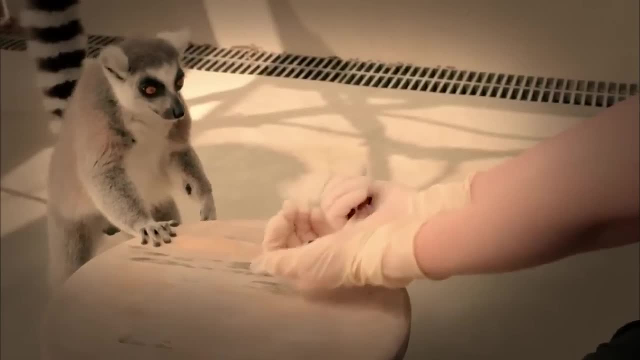 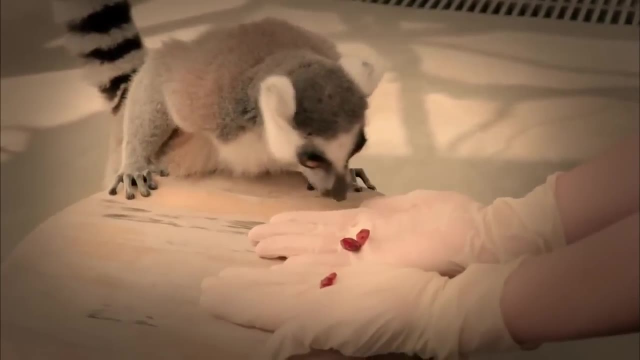 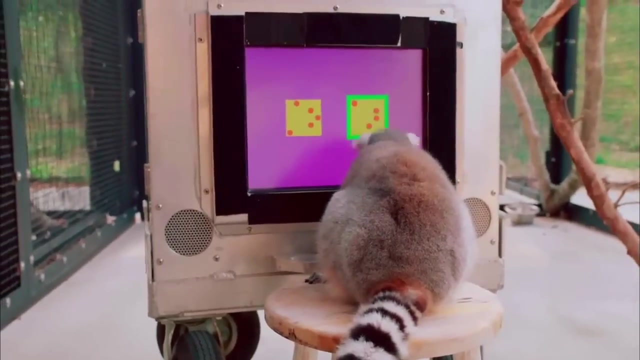 when they compare two quantities. Well, clearly he's not using verbal labels, He's not using symbols. We need to figure out whether they can really use number, pure number, as a cue To test how well Terrys can distinguish quantities. 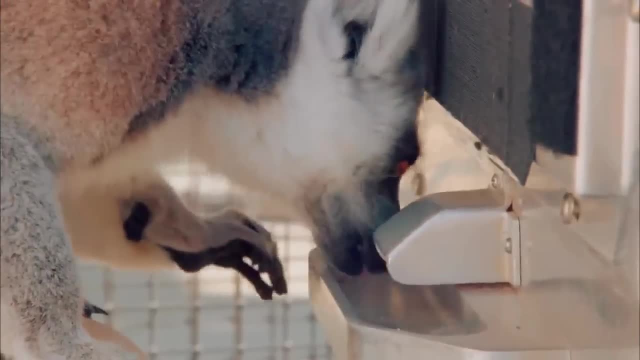 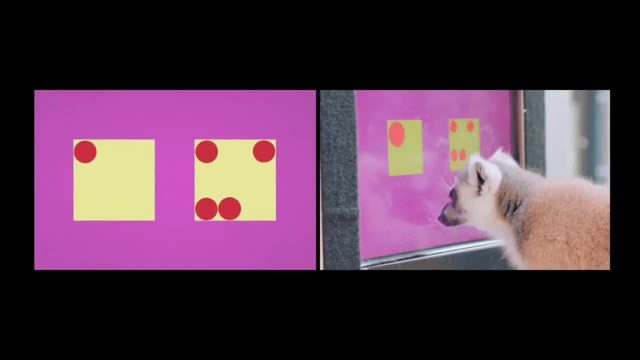 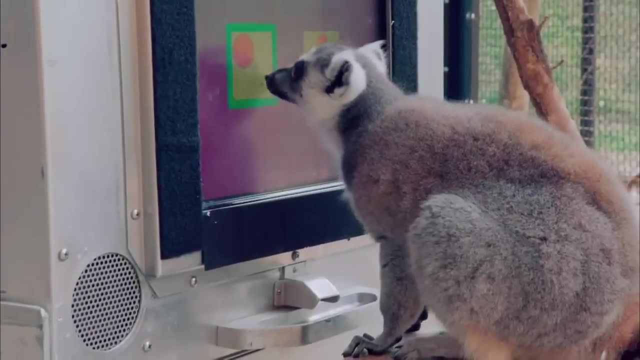 he's been taught a touch-screen computer game. The red square starts around. If he touches it, two squares appear containing different numbers of objects. He's been trained that if he chooses the box with the fewest number, he'll get a reward. 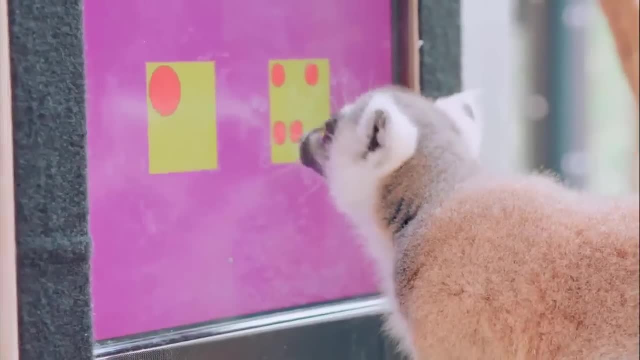 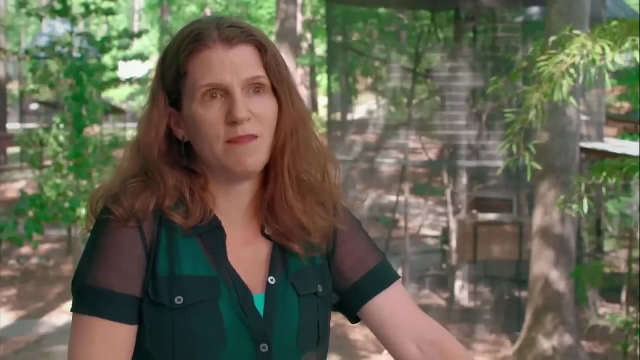 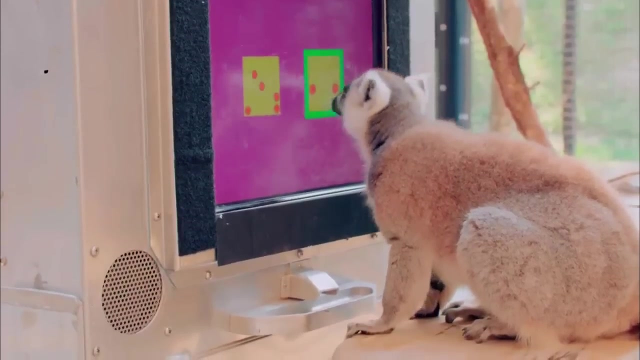 a sugar pellet? A wrong answer. We have to do a lot to ensure that they're really attending to number and not something else, To make sure the test animal is reacting to the number of objects and not some other cue. Liz varies the object's size. 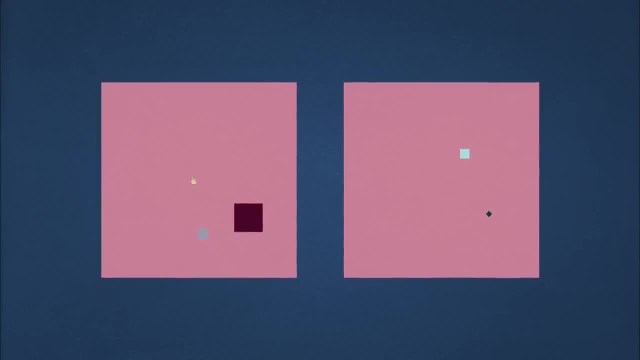 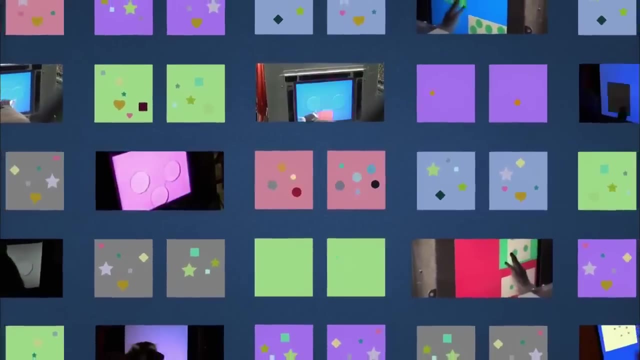 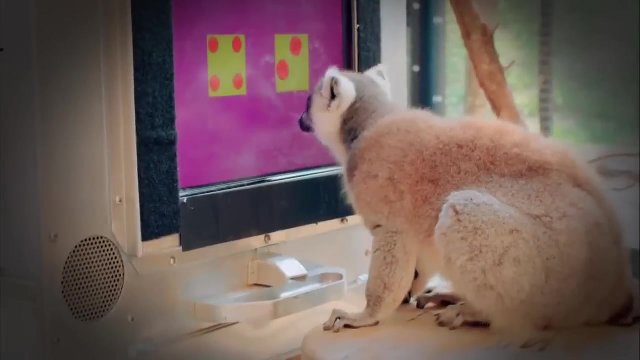 color and shape. She has conducted thousands of trials and shown that lemurs and rhesus monkeys can learn to pick the right answer. Terrys obviously doesn't have language and he doesn't have any symbols for number. So is he counting? 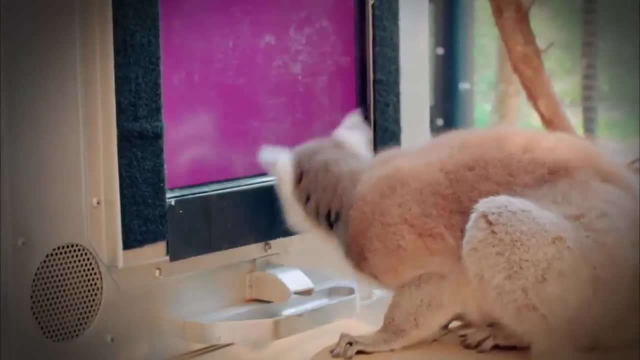 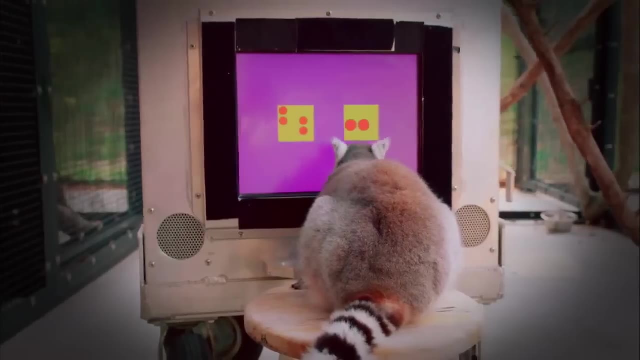 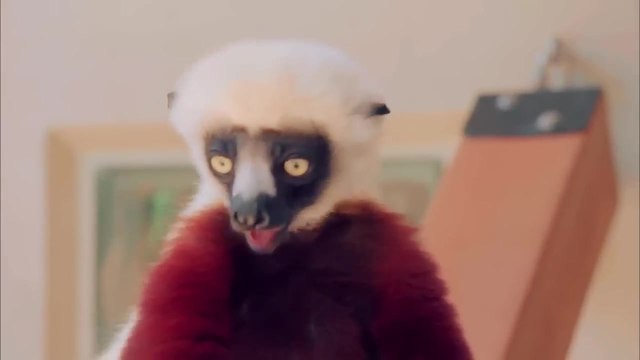 Is he doing what a human child does when they recite the numbers one, two, three, No, And yet what he seems to be attending to is the very abstract essence of what a number is. Lemurs and rhesus monkeys aren't alone. 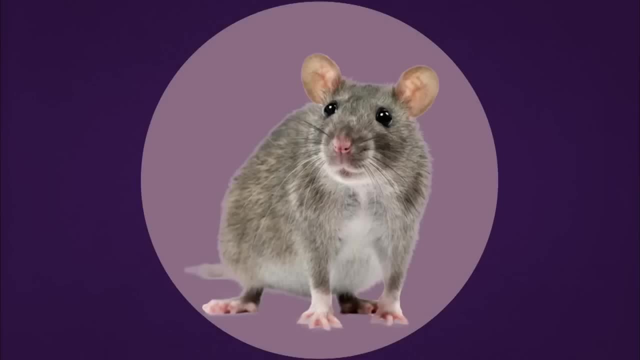 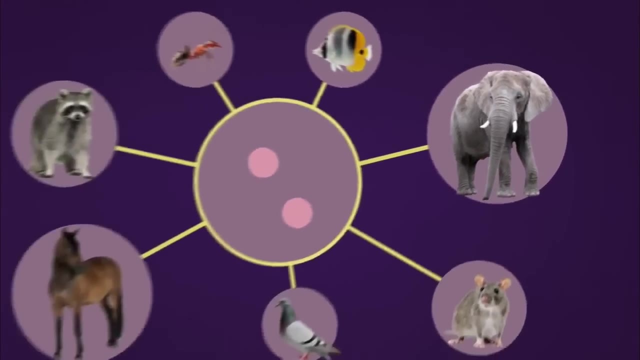 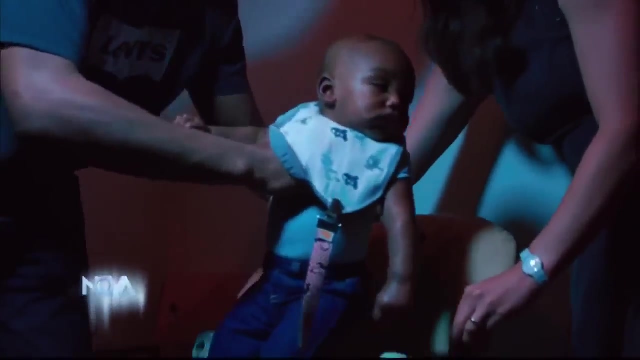 in having this primitive number sense. Rats, pigeons, fish, raccoons, insects, horses and elephants all show sensitivity to quantity, And so do human infants. They're gonna be filming him At her lab on the Duke campus. 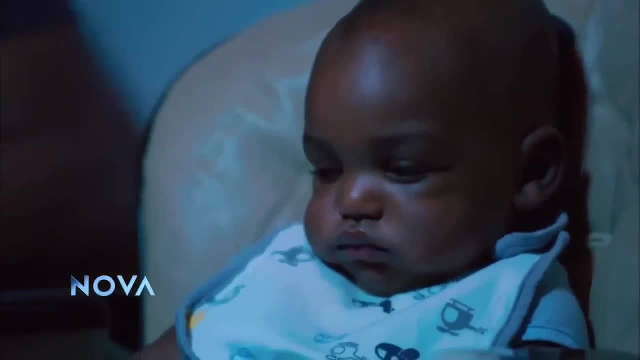 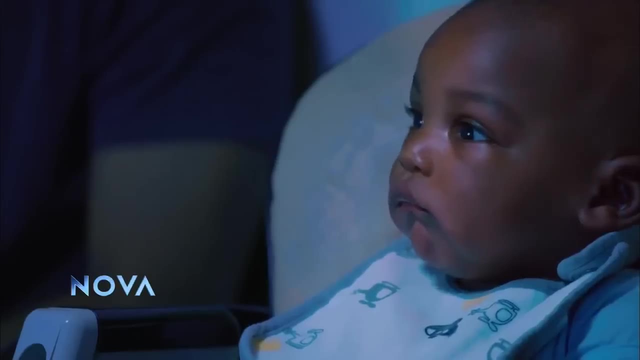 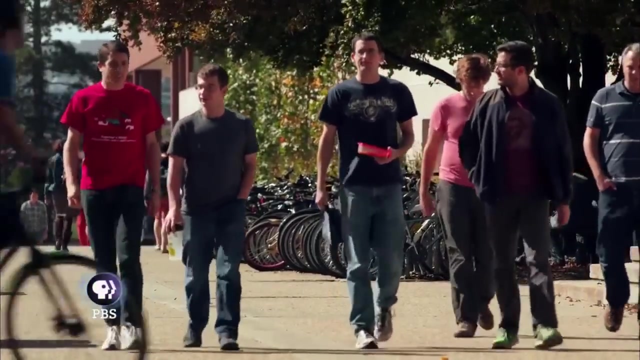 Liz has tested babies that were only six months old. They'll look longer at a screen with a changing number of objects, as long as the change is obvious enough to capture their attention. Liz has also tested college students, asking them not to count. 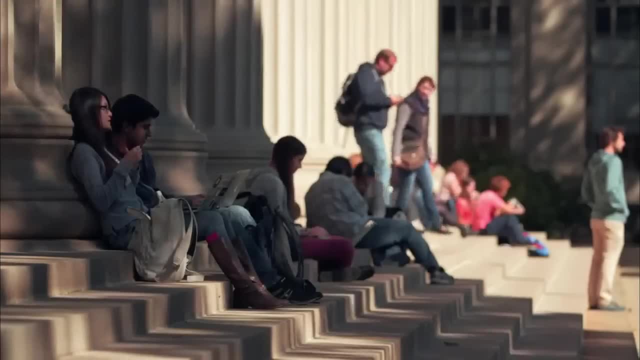 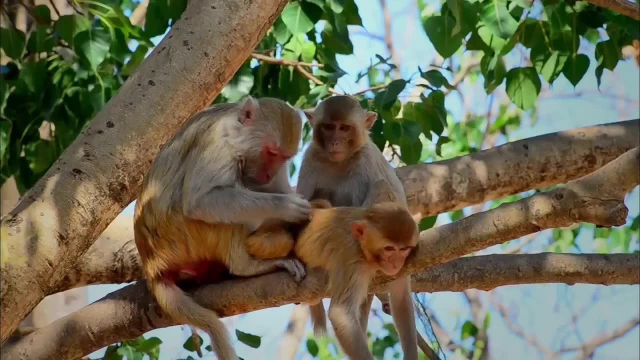 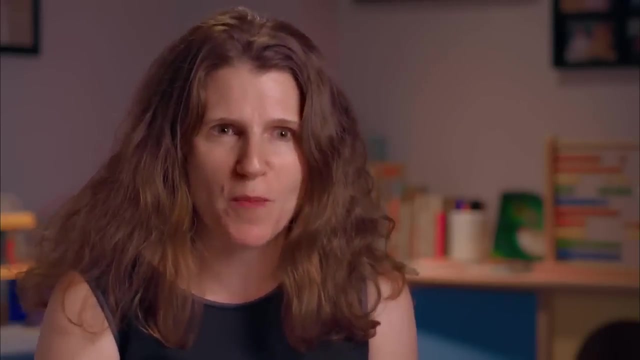 but to respond as quickly as they could to a touchscreen test comparing quantities. The results About the same as lemurs and rhesus monkeys. In fact, there are humans who aren't as good as our monkeys and others that are far better. 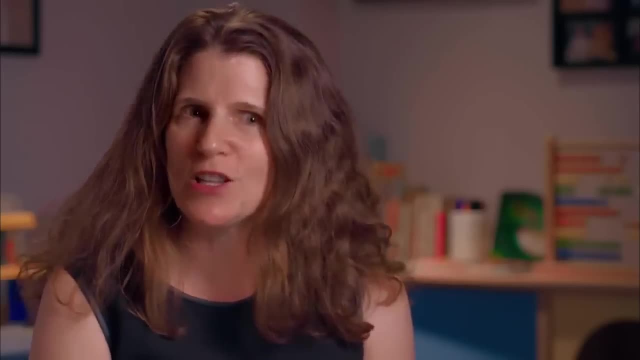 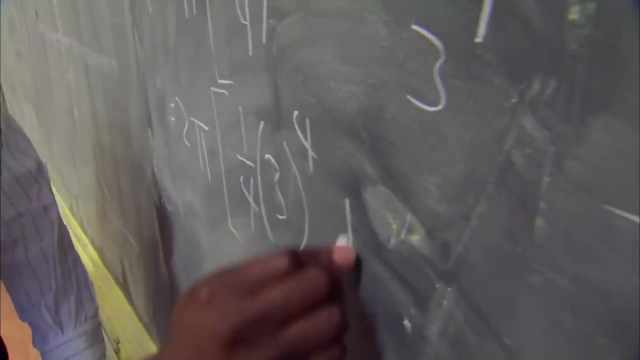 So there's a lot of variability in human performance, but in general it looks very similar to a monkey. Number five Substitute in the three, you raise that to the four, Even without any mathematical education, even without learning any number words or symbols. 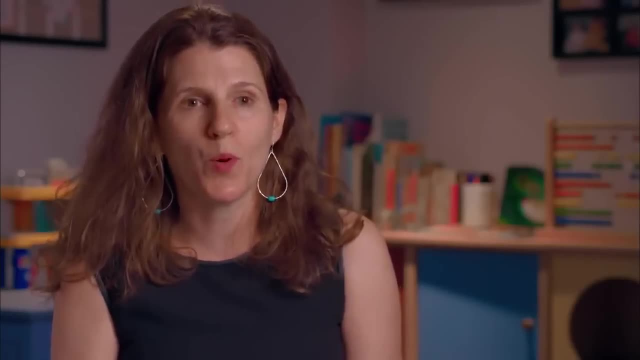 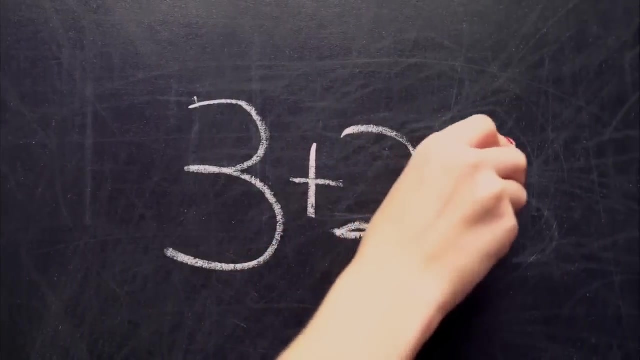 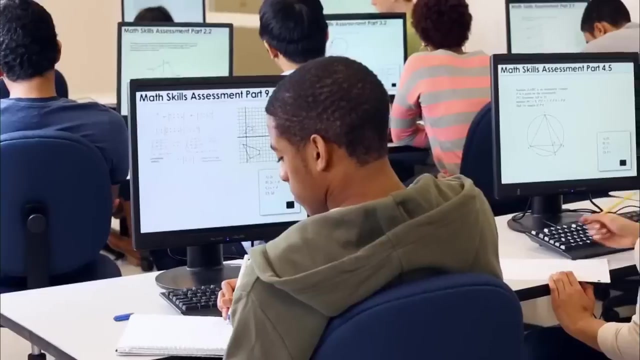 we would still have, all of us as humans, a primitive number sense. That fundamental ability to perceive number seems to be a very important foundation, and without it it's very questionable as to whether we could ever appreciate symbolic mathematics, The building blocks of mathematics. 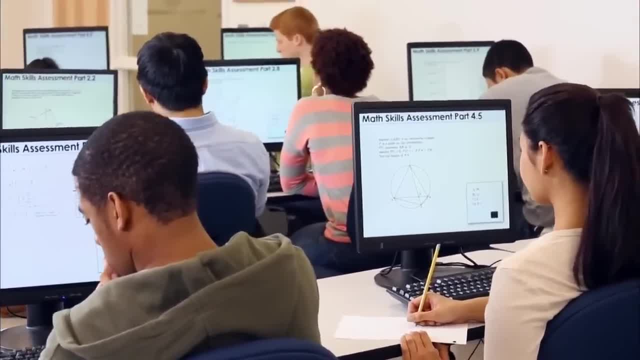 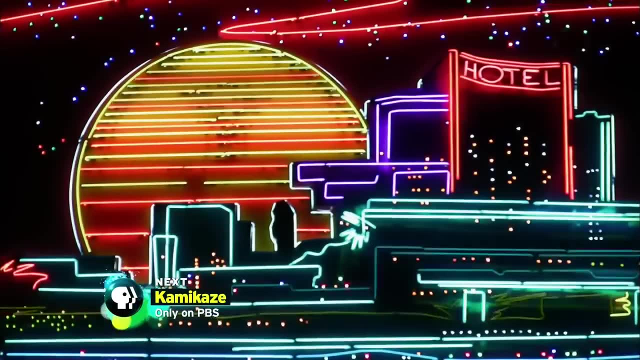 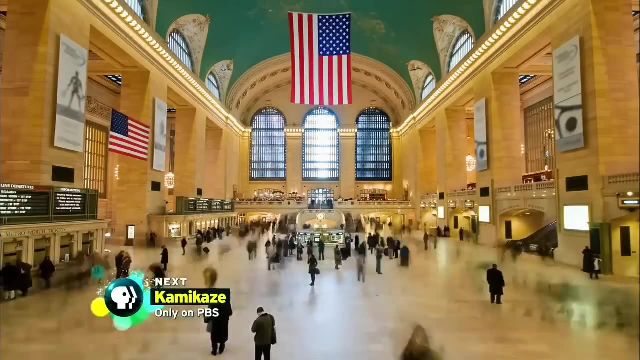 may be pre-programmed into our brains, part of the basic toolkit for survival, like our ability to recognize patterns and shapes, or our sense of time. From that point of view, on this foundation we've erected one of the greatest inventions of human culture. 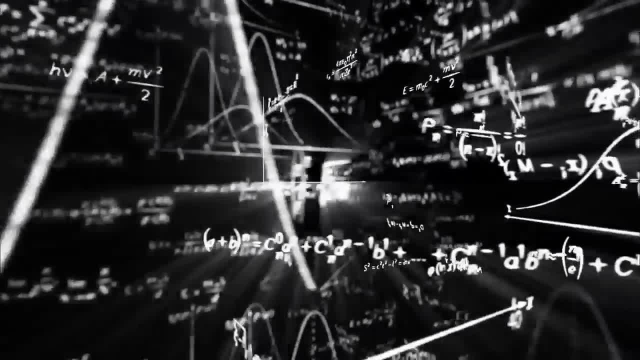 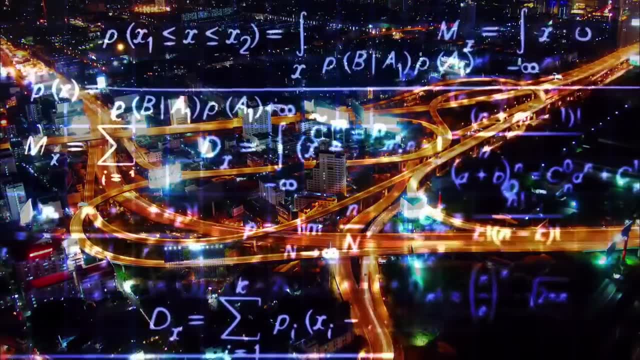 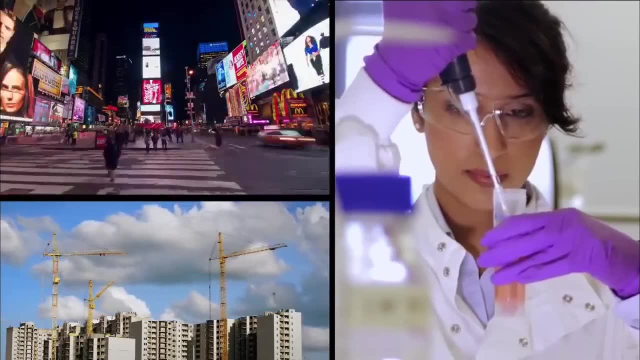 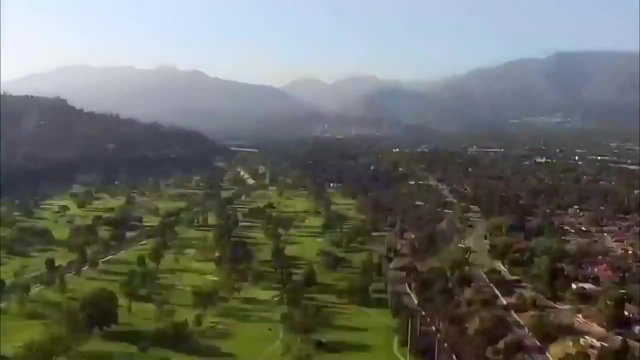 Mathematics, But the mystery remains. If it is all in our heads, why has math been so effective? Through science, technology and engineering, it's transformed the planet, even allowing us to go into the beyond, As in the work here. 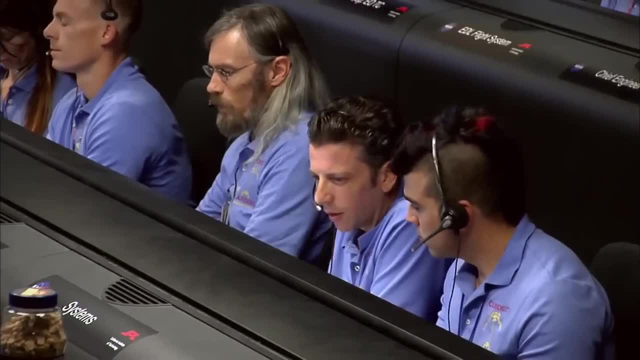 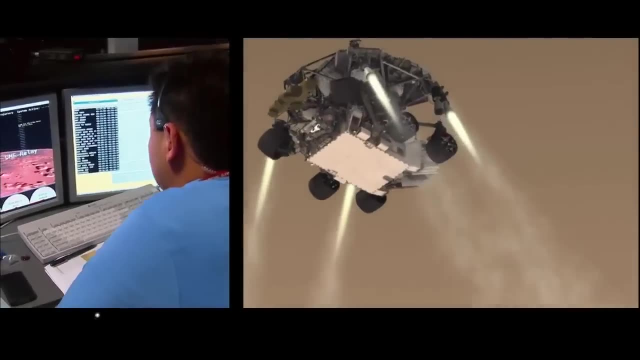 at NASA's Jet Propulsion Laboratory in Pasadena, California, Roger Copy mission, Coming up on entry In 2012.. Sky green has started. they landed a car-sized rocket standing at about 0.75 meters per second, as expected. 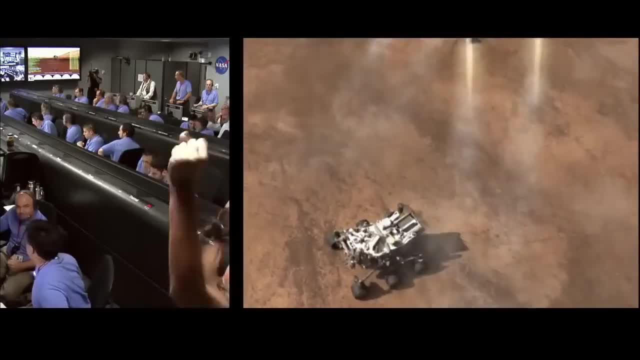 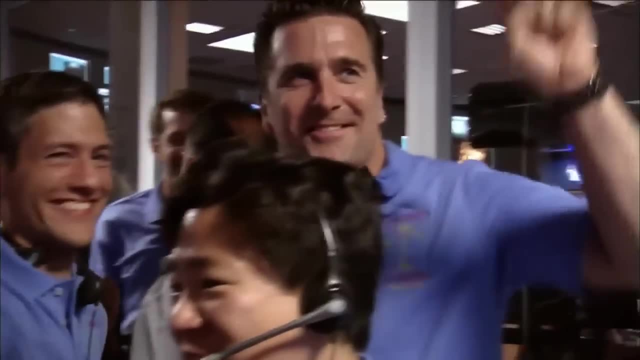 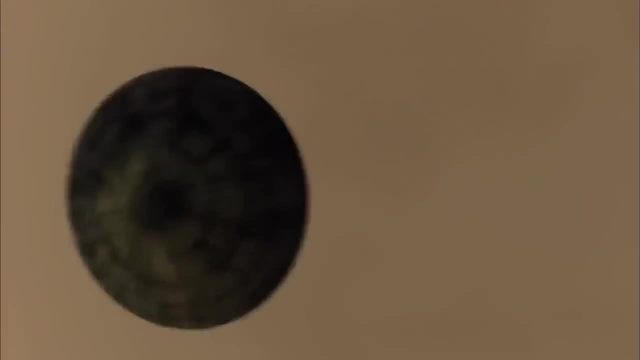 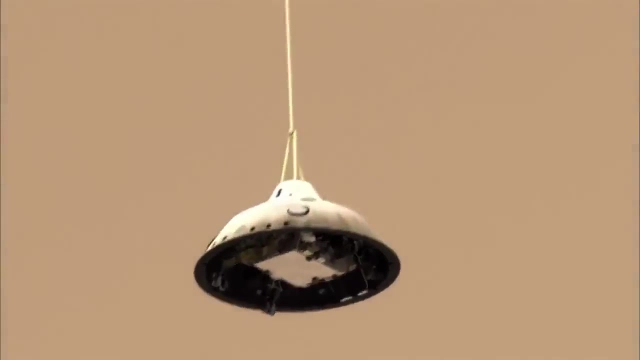 on Mars: Touchdown confirmed Received. Adam Stelzner was the lead engineer on the team that designed the landing system. Their work depended on a groundbreaking discovery from the Renaissance that turned mathematics into the language of science: The law of falling bodies. 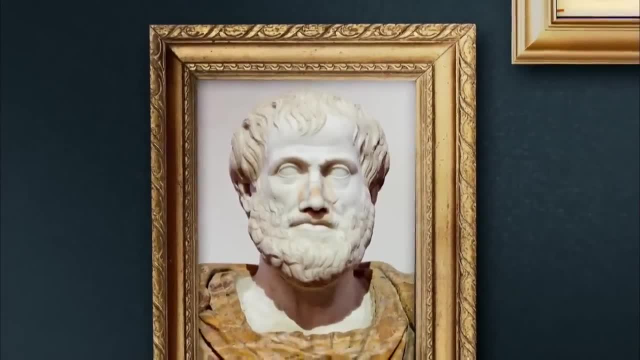 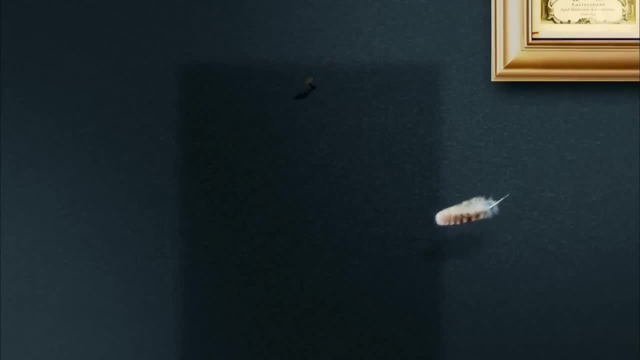 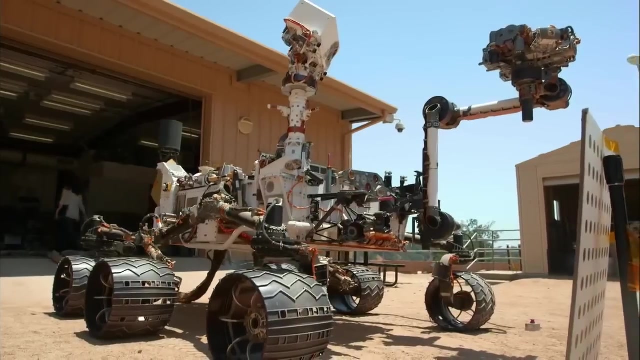 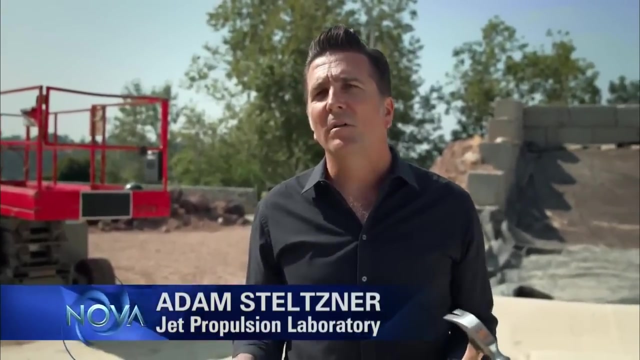 The ancient Greek philosopher, Aristotle, taught that heavier objects fall faster than lighter ones, An idea that on the surface makes sense, Even this surface, the Mars yard where they test the rovers at JPL. So Aristotle reasoned that the rate at which things would fall, 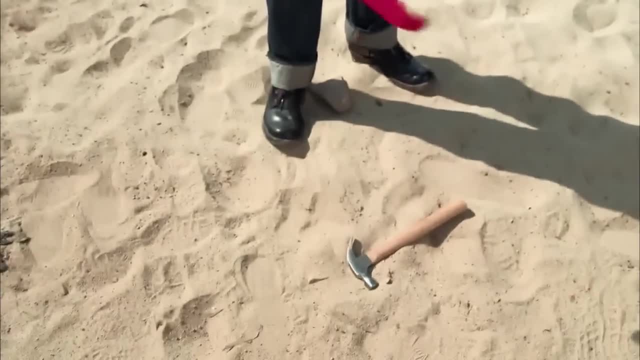 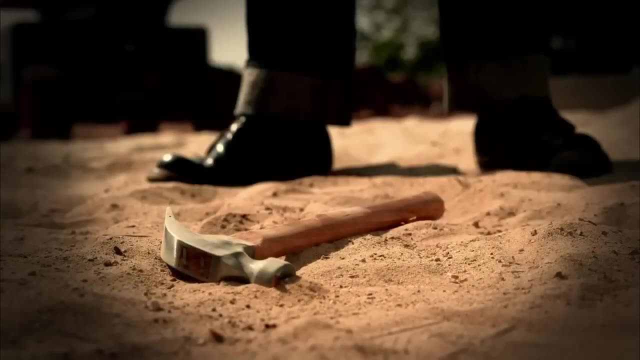 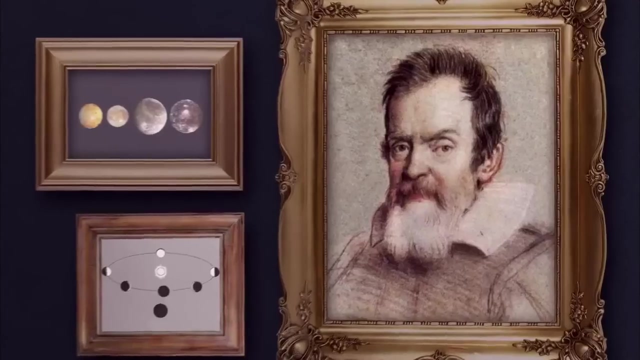 was proportional to their weight, Which seems reasonable, In fact so reasonable, the view held for nearly 2,000 years Until challenged in the late 1500s, by Italian mathematician Galileo Galilei. Legend has it that Galileo dropped. 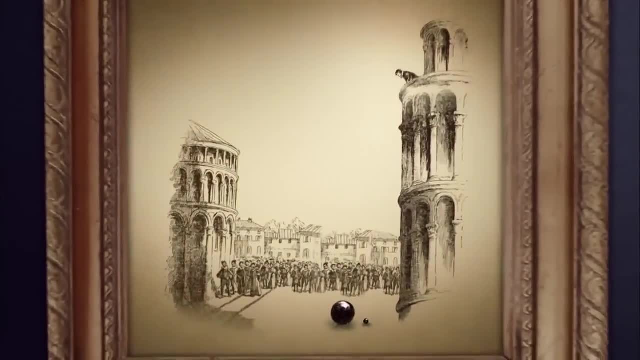 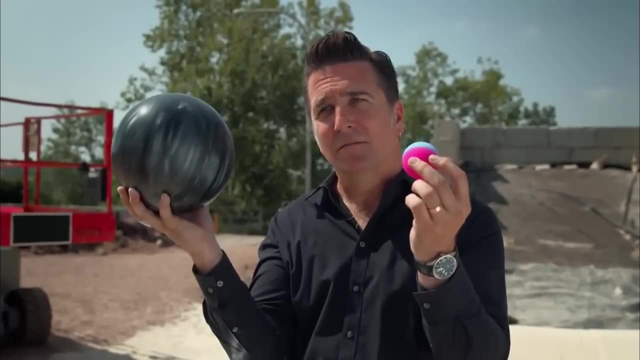 two different weight cannonballs from the leaning tower of Pisa. Well, we're not in Pisa, We don't have cannonballs, But we do have a bowling ball and a bouncy ball. Let's weigh them First. we weigh the bowling ball. 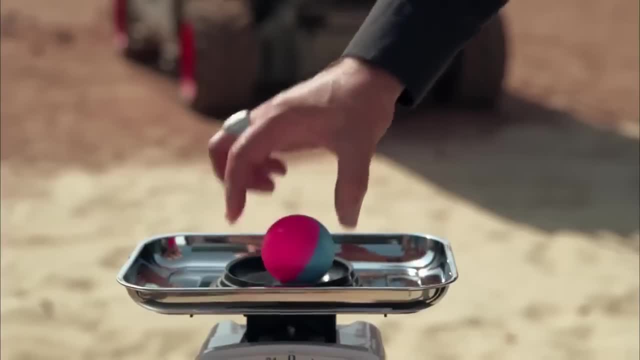 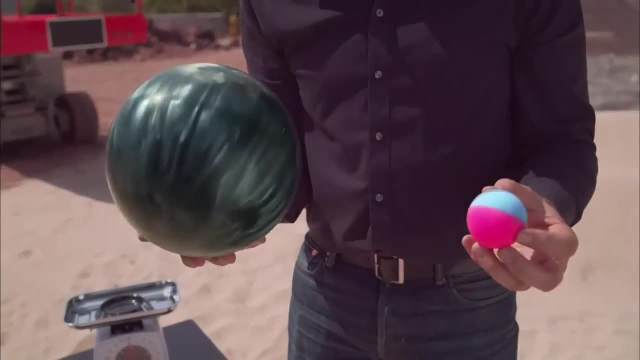 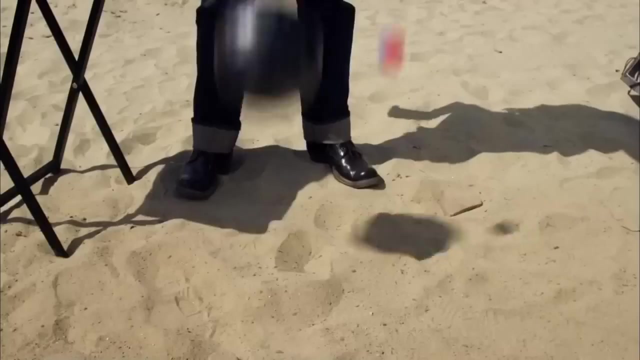 It weighs 15 pounds, And the bouncy ball? it weighs hardly anything. Let's drop them. According to Aristotle, the bowling ball should fall over 15 times faster than the bouncy ball. Well, they seem to fall at the same rate. 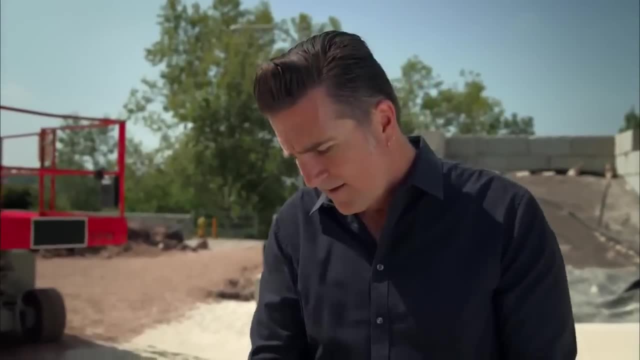 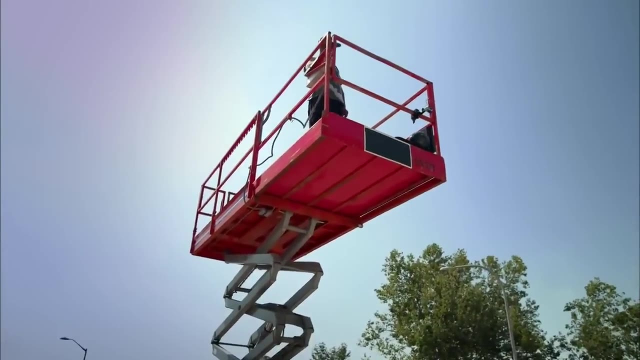 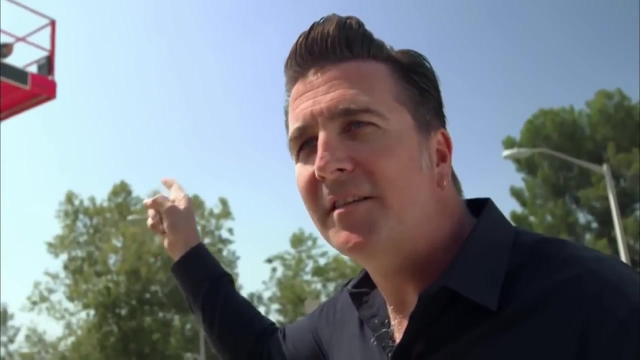 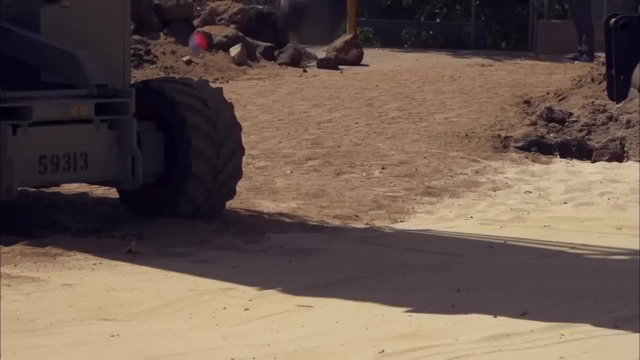 This isn't that high, though. Maybe we should drop them from higher. So Ed is 20 feet in the air up there. Let's see if the balls fall at the same rate. Ready Three, two, one drop. Galileo was right. 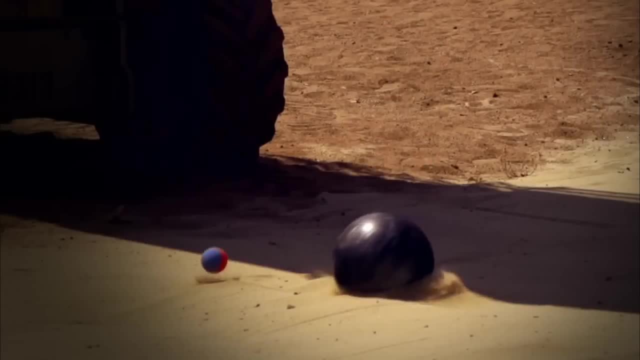 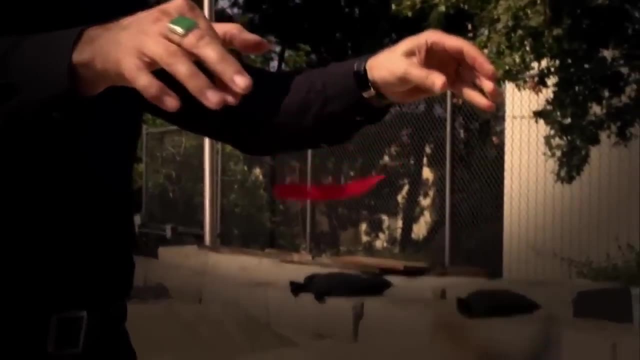 Aristotle, you lose. Dropping feathers and hammers is misleading, thanks to air resistance. Well, in my left hand I have a feather, In my right hand a hammer. A fact demonstrated on the moon, where there is no air. 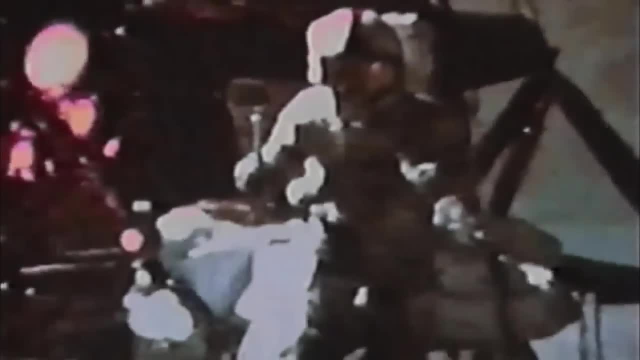 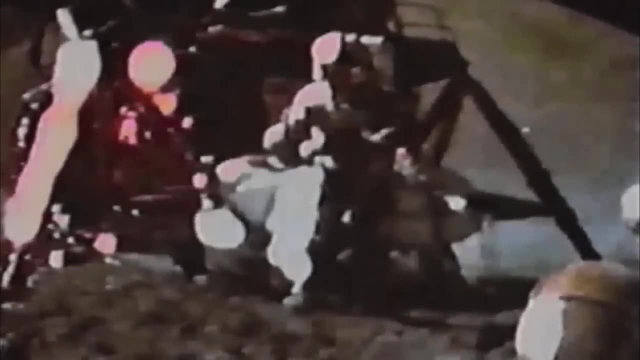 in 1971,, during the Great Depression, was that there was no air in the air, And that's why we're here today, And that's why we're here today, And that's why we're here today In 1971,, during the Apollo 15 mission. 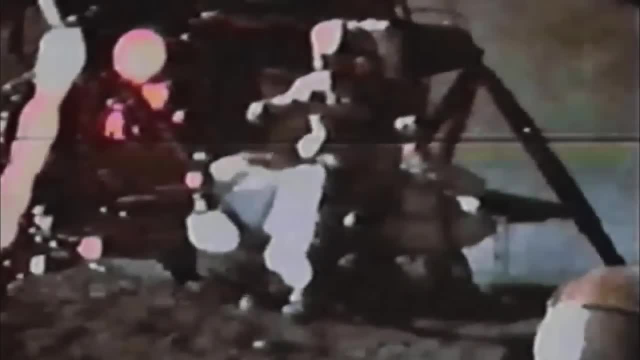 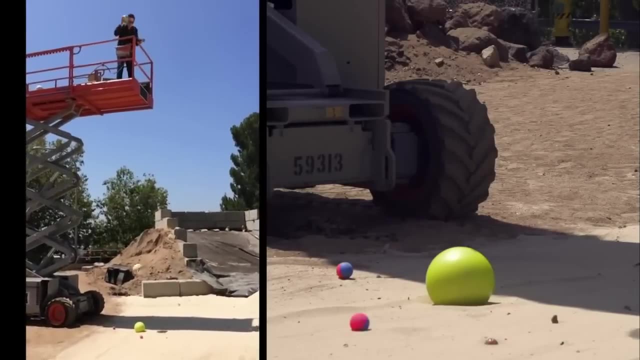 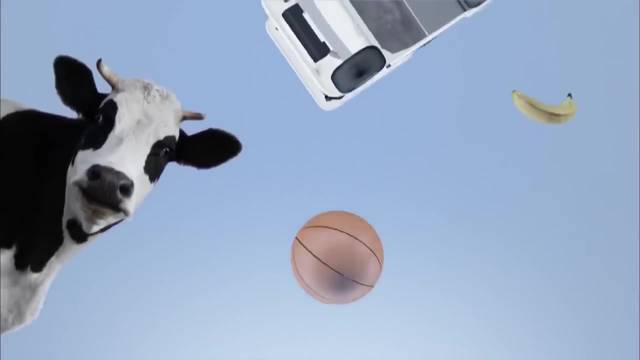 And I'll drop the two of them here. How about that? Mr Galileo was correct. Little balls, Soccer balls, So, while counterintuitive Vegetables? If you take the air out of the equation, everything falls at the same rate. 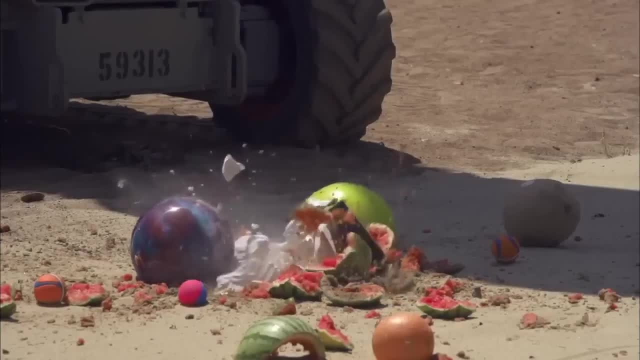 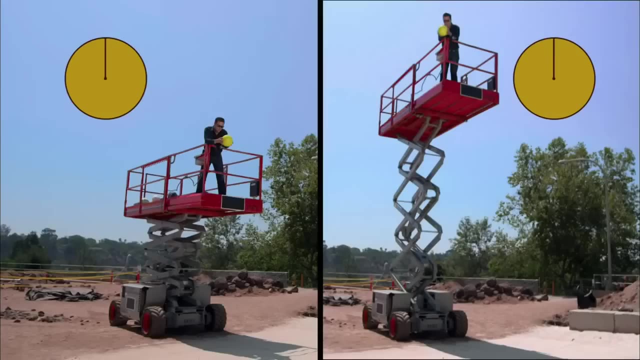 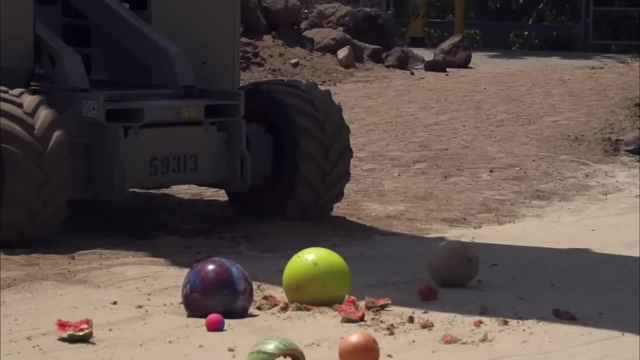 Even Aristotle. But what really interested Galileo was that an object dropped at one height didn't take twice as long to drop from twice as high. It accelerated. But how do you measure that Everything is happening so fast? Galileo came up with 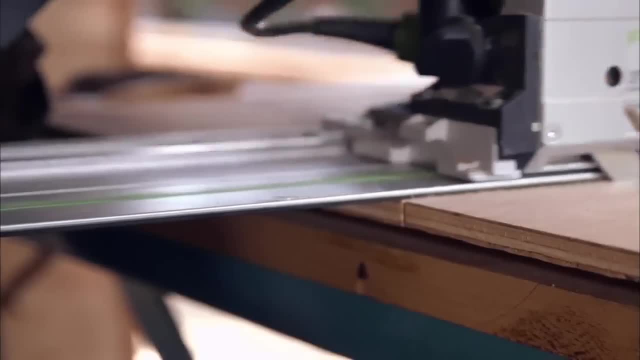 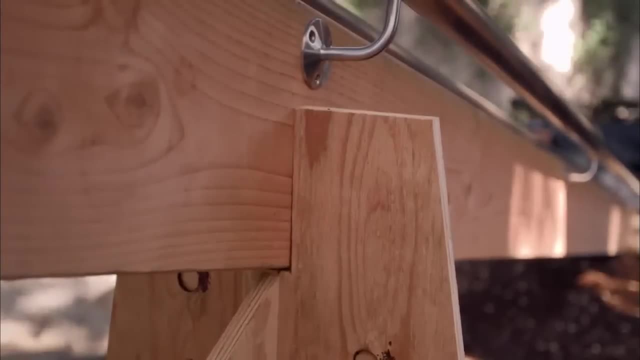 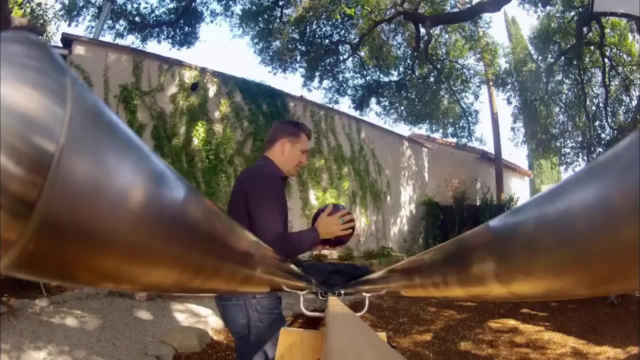 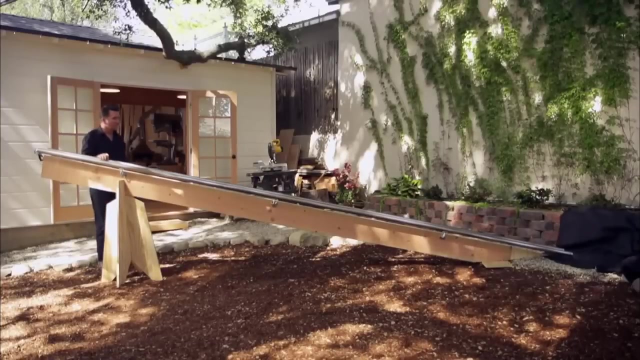 an ingenious solution. He built a ramp, An inclined plane To slow the falling motion down so he could measure it. So we're going to use this ramp to find the relationship between distance and time. For time I'll use an arbitrary unit. 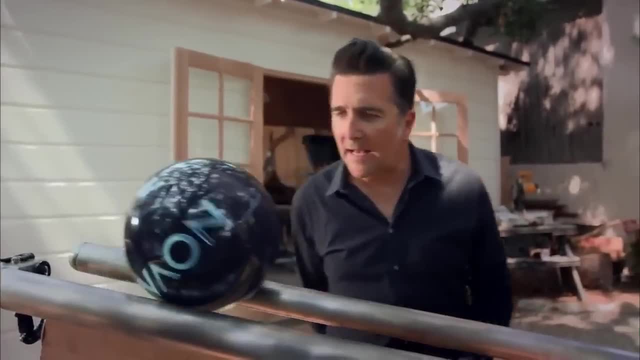 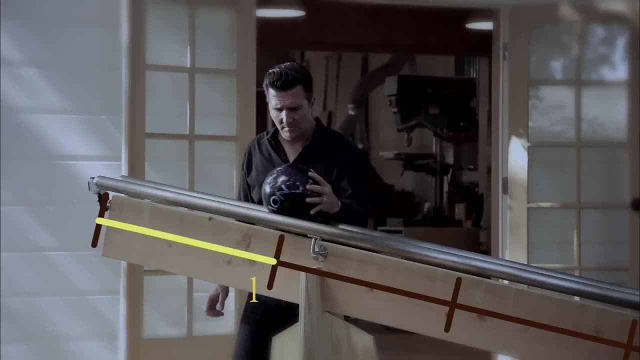 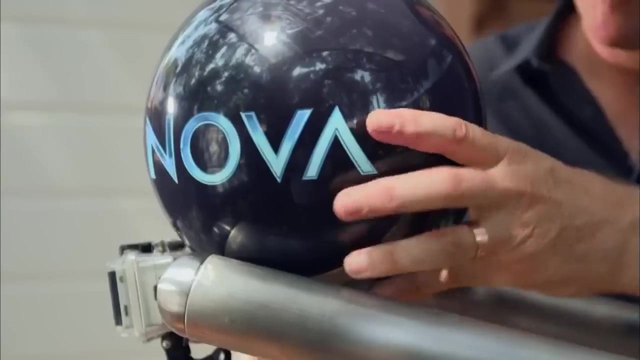 A Galileo. One Galileo, The length of the ramp that the ball rolls during one Galileo becomes one unit of distance. So we've gone one unit of distance in one unit of time. Now let's try it for a two count. 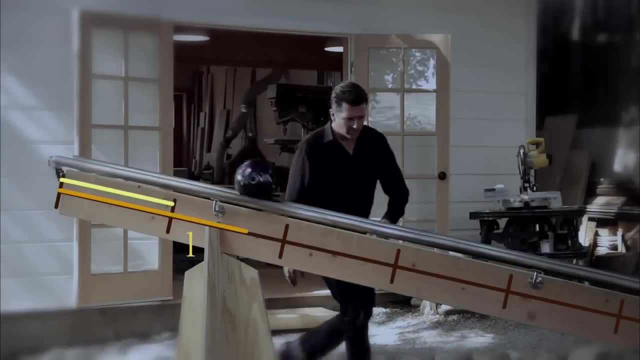 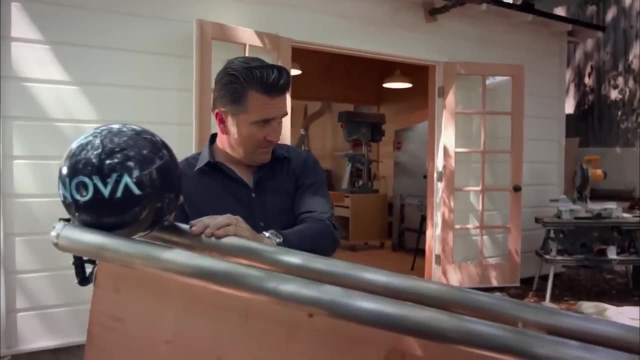 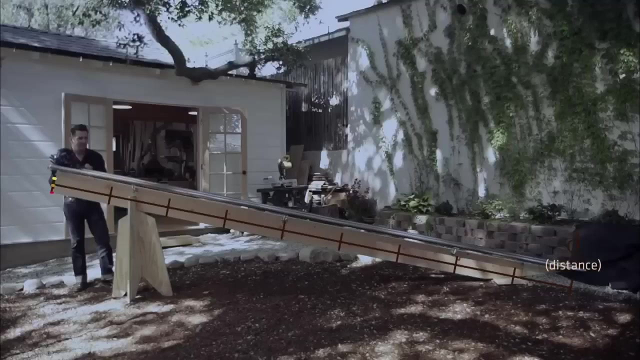 One Galileo, Two Galileo In two units of time. the ball has rolled four units of distance. Now let's see how far it goes in three Galileos: One Galileo, Two Galileo, Three Galileo In three units of time. 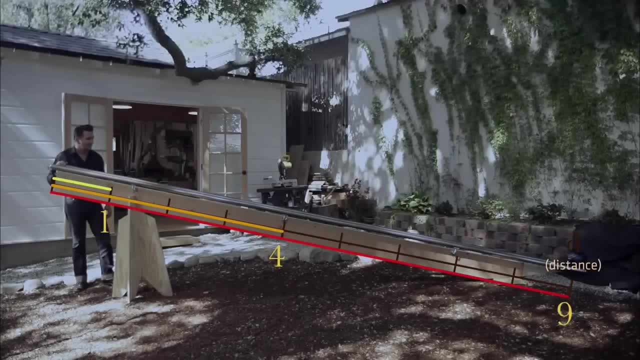 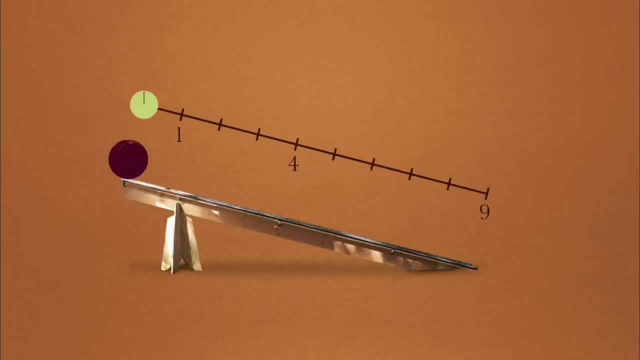 the ball has gone nine units of distance. So there it is. There's a mathematical relationship here between time and distance. Galileo's inspired use of a ramp had shown. falling objects follow mathematical laws. The distance the ball traveled is directly proportional to the square of the time. 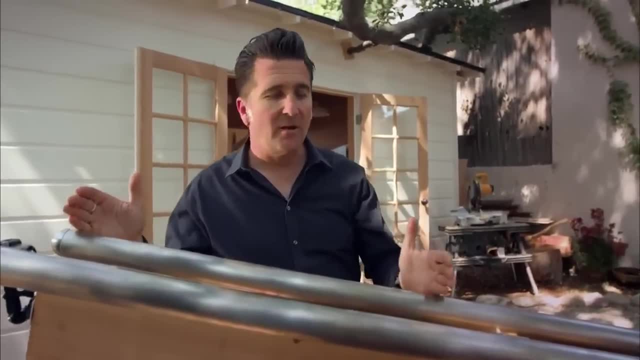 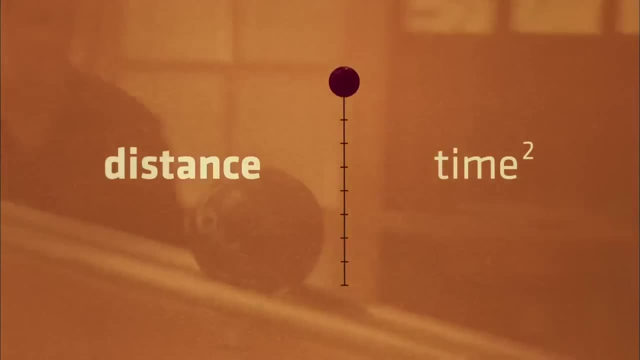 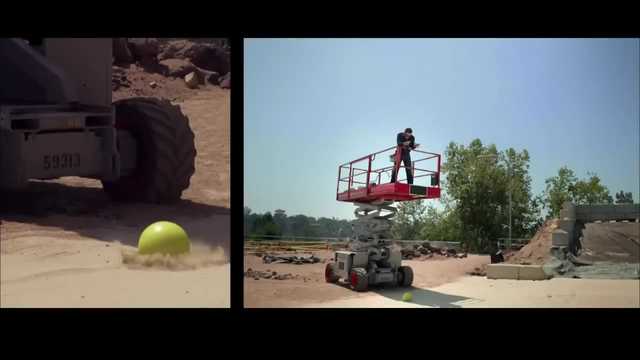 That mathematical relationship that Galileo observed is a mathematical expression of the physics of our universe. Galileo's centuries-old mathematical observation about falling objects remains just as valid today. It's the same mathematical expression that we can use to understand how objects might fall here on Earth. 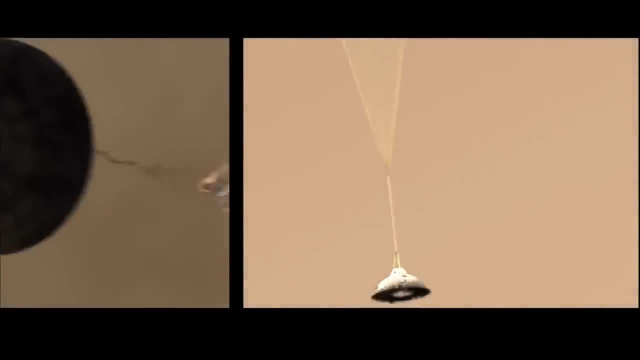 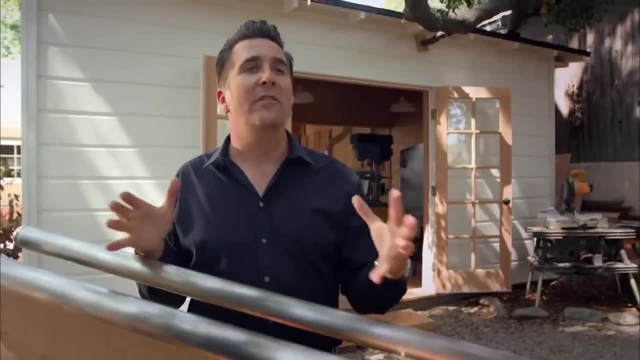 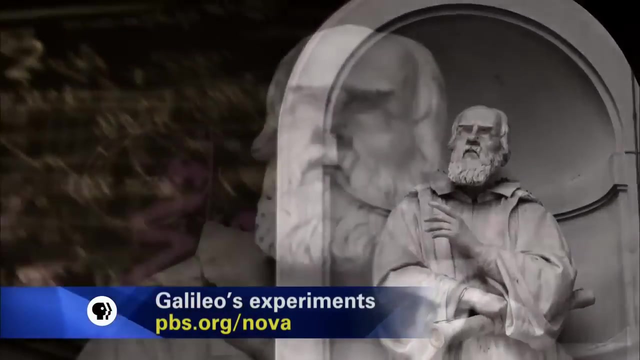 roll down a ramp. It's even a relationship that we used to land the Curiosity rover on the surface of Mars. That's the power of mathematics. Galileo's insight was profound: Mathematics could be used as a tool to uncover and discover the hidden rules of our world. 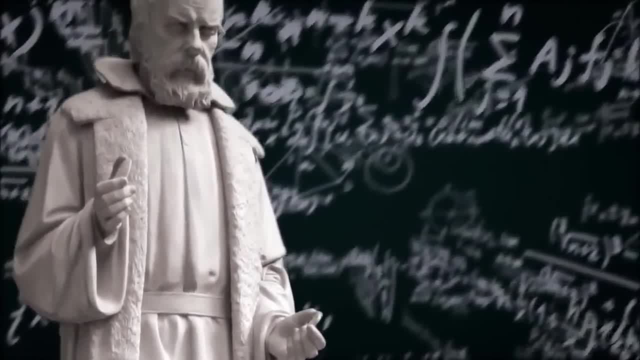 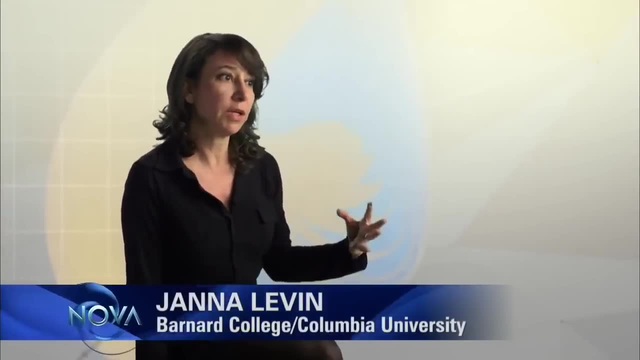 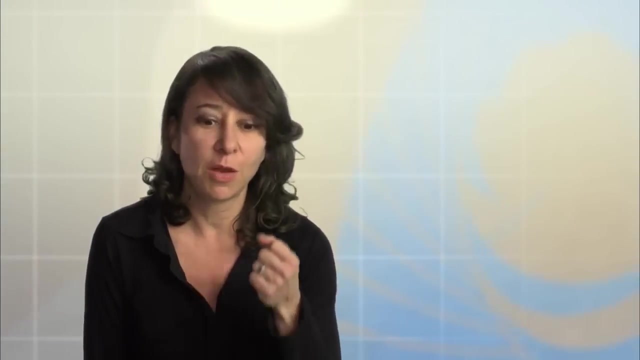 He later wrote, the universe is written in the language of mathematics. Math is really the language in which we understand the universe. We don't know why it's the case that the laws of physics and the universe follows mathematical models, but it does seem to be the case. 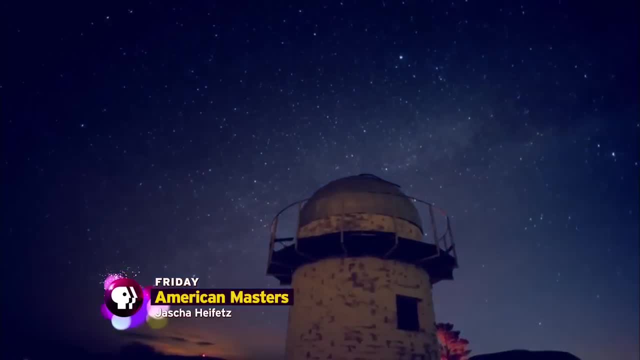 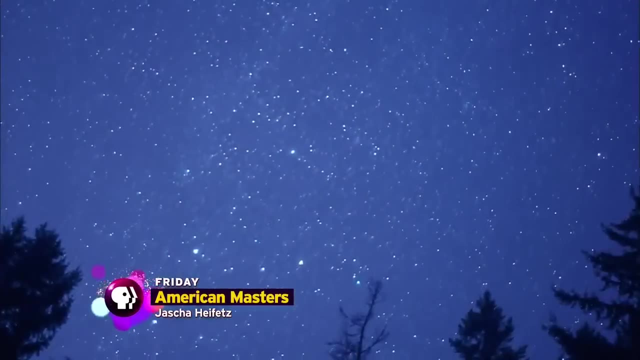 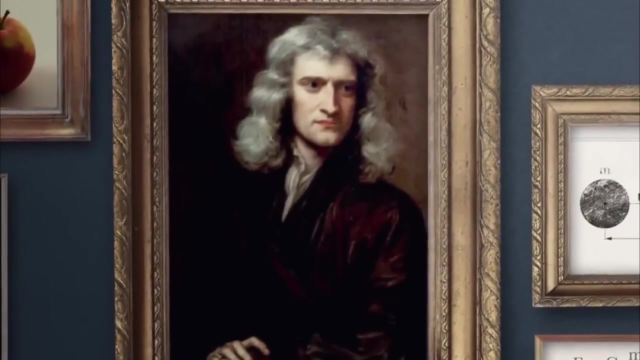 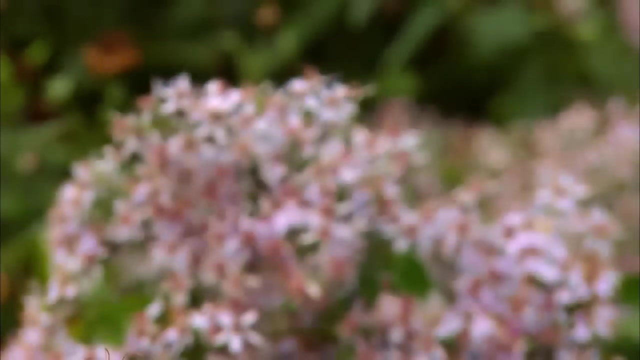 While Galileo turned mathematical equations into laws of science, it was another man, born the same year Galileo died, who took that to new heights that crossed the heavens. His name was Isaac Newton. He worked here at Trinity College in Cambridge, England. Newton cultivated the reputation. 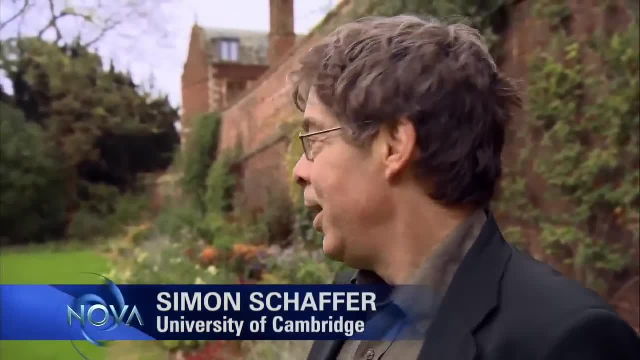 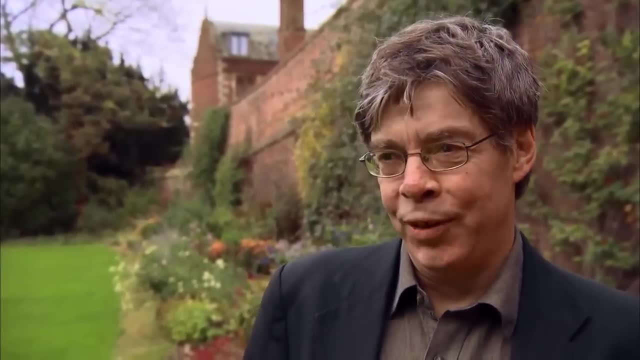 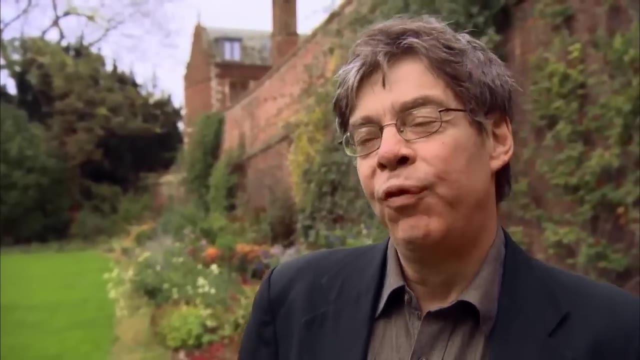 of being a solitary genius, and here in the Bowling Green of Trinity College it was said that he would walk meditatively up and down the paths, absentmindedly, drawing mathematical diagrams in the gravel, and the fellows were instructed, or so it was said. 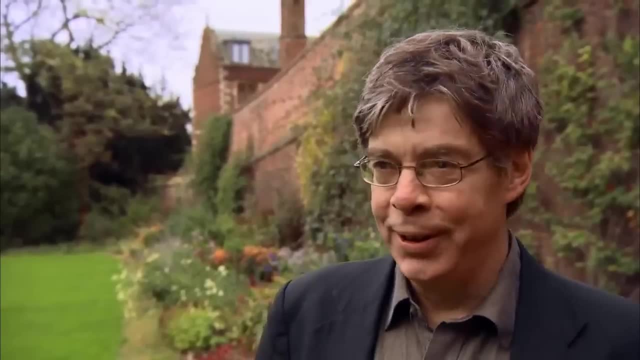 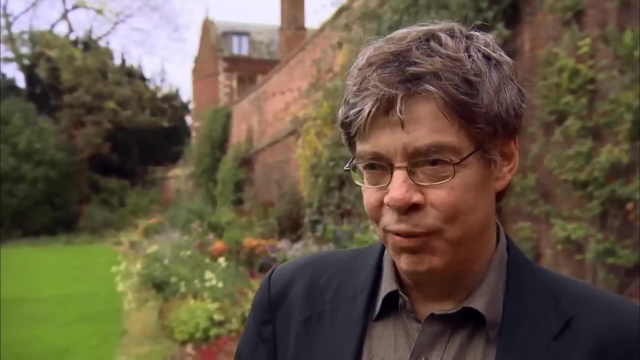 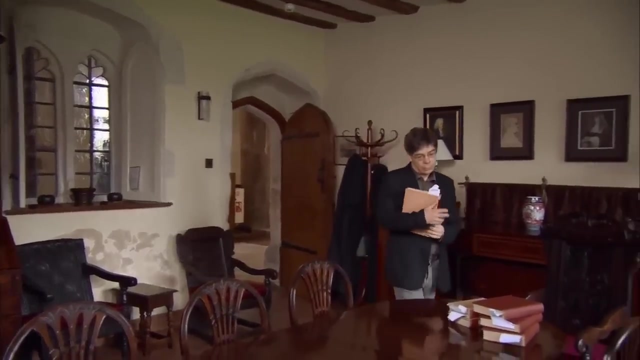 not to disturb him, not to clear up the gravel after he'd passed, in case they inadvertently wiped out some major scientific or mathematical discovery. In 1687, Newton published a book that would become a landmark in the history of science. Today it is known simply. 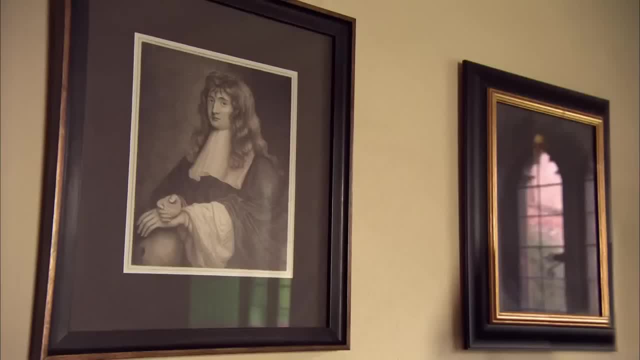 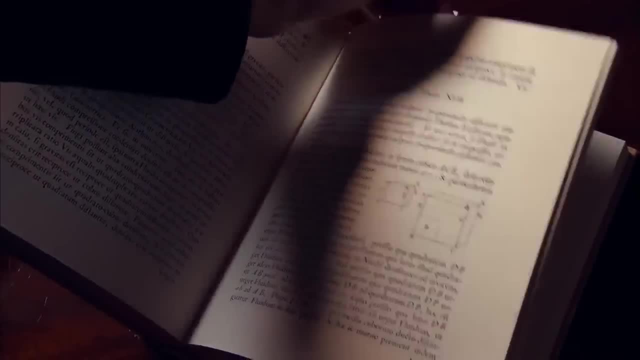 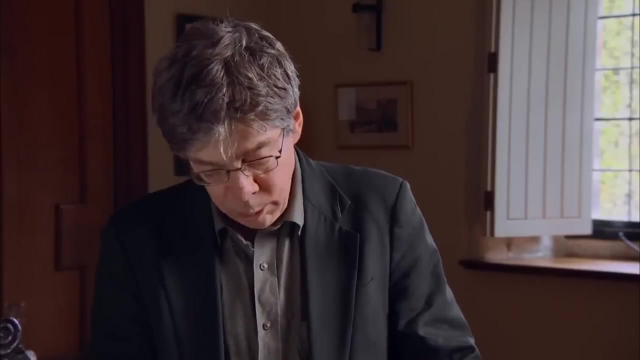 as the Principia In it. Newton gathered observations from around the world and used mathematics to explain them, For instance that of a comet seen widely in the fall of 1680.. He gathers data worldwide in order to construct the comet's path. 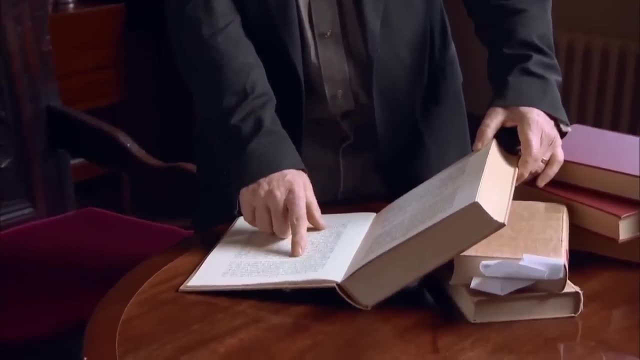 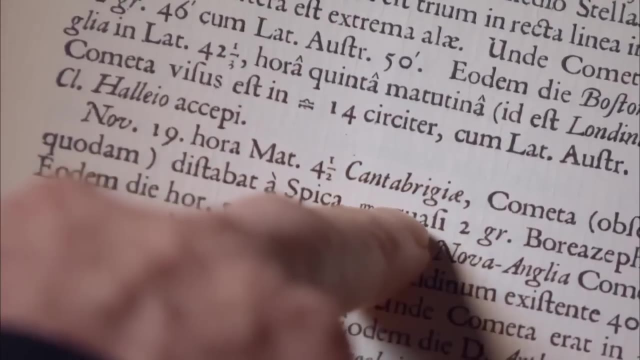 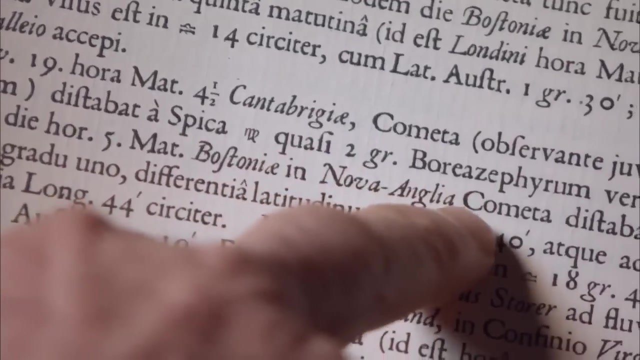 So for November the 19th he begins with an observation made in Cambridge, in England, at 4.30 am by a certain young person, and then at 5 in the morning at Boston in New England. So what Newton does is to accumulate numbers. 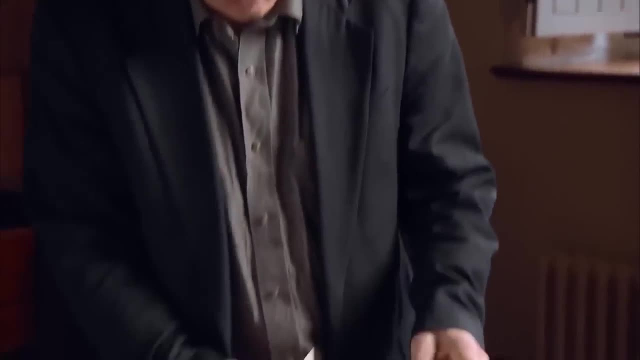 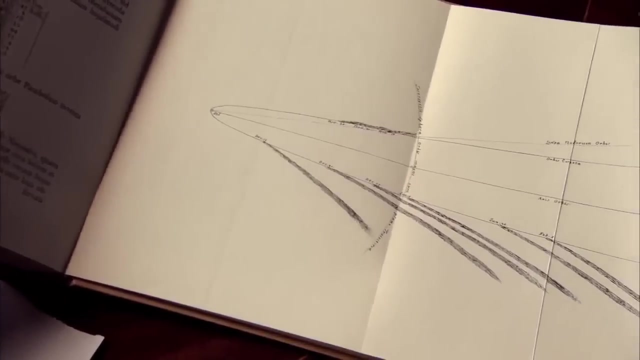 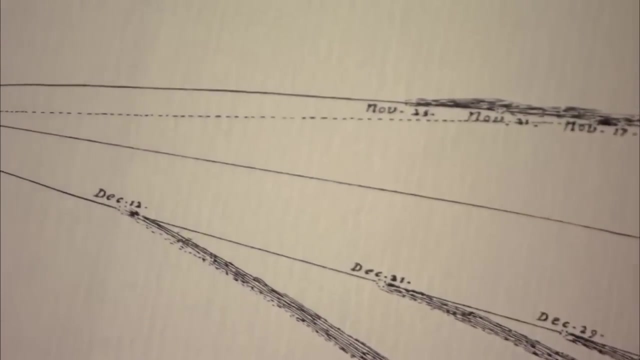 made by observers spread right across the globe in order to construct an unprecedentedly accurate calculation of how this great comet moved through the sky. Newton's groundbreaking insight was that the force that sent the comet hurtling around the Sun was the same force that brought cannonballs. 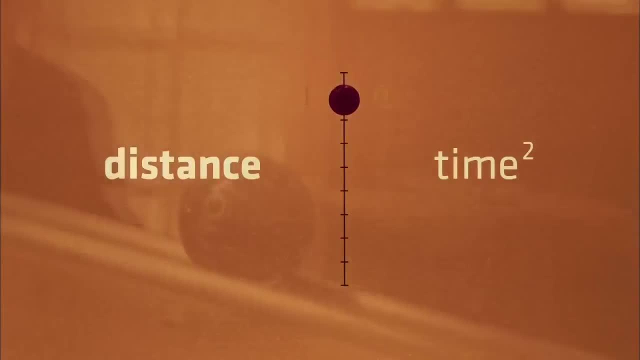 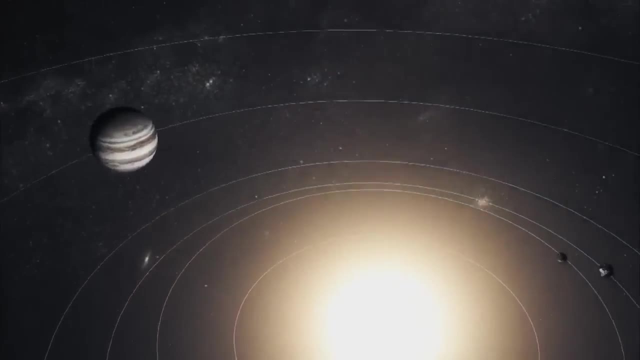 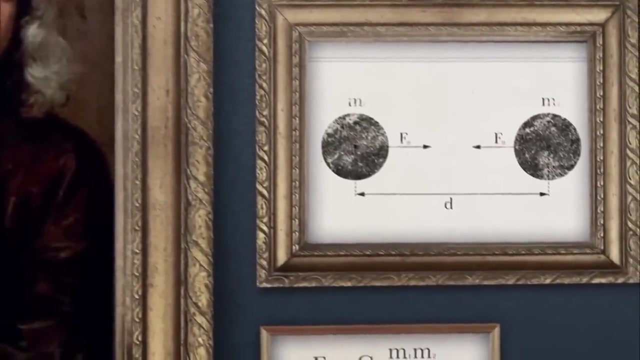 back to Earth. It was the force behind Galileo's law of falling bodies, And it even held the planets in their orbits. He called the force gravity and described it precisely in a surprisingly simple equation that explains how two masses attract each other. 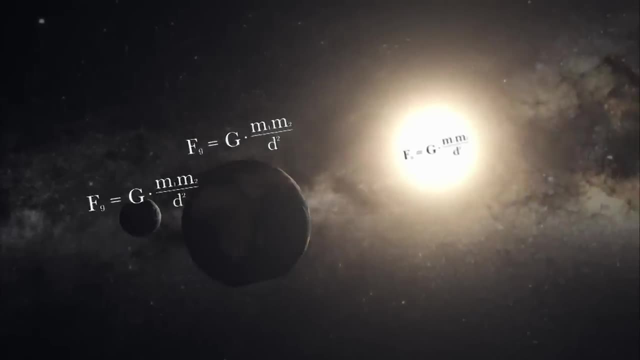 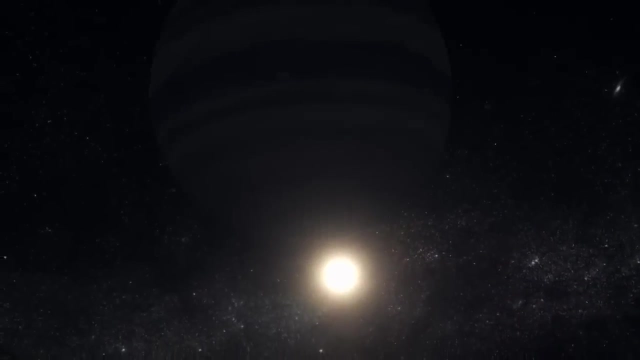 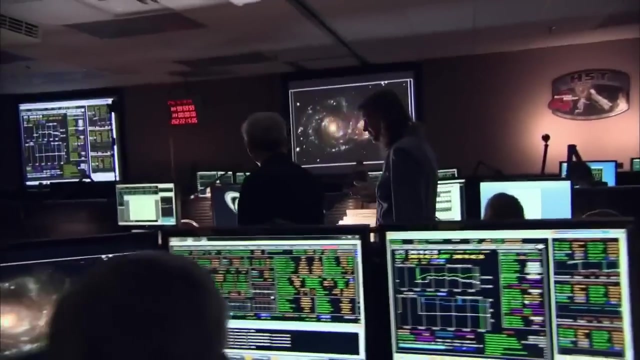 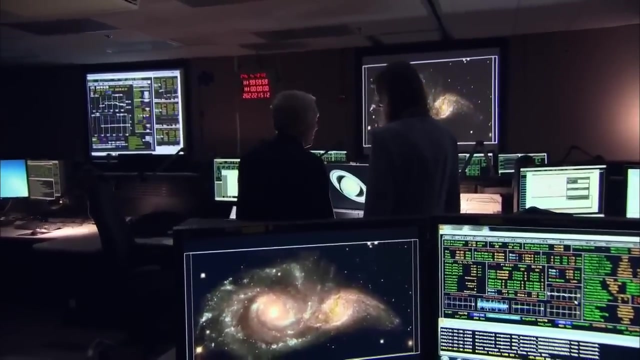 whether here on Earth or in the heavens above. What's so impressive and so dramatic is that a single mathematical law would allow you to move throughout the universe. Today, we can even witness it at work beyond the Milky Way. This is a picture of two galaxies. 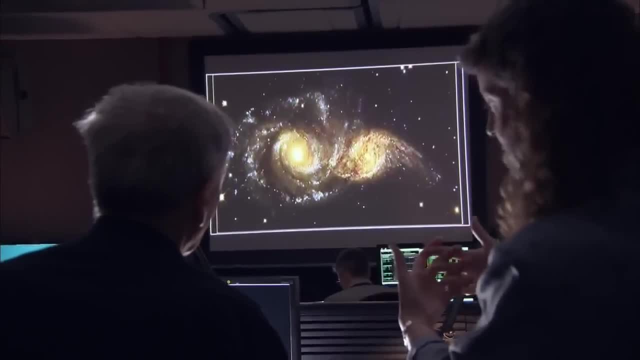 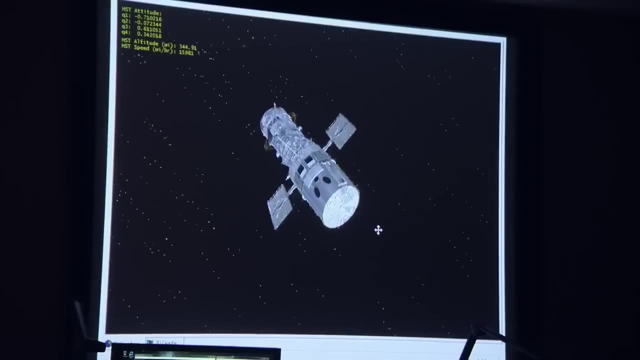 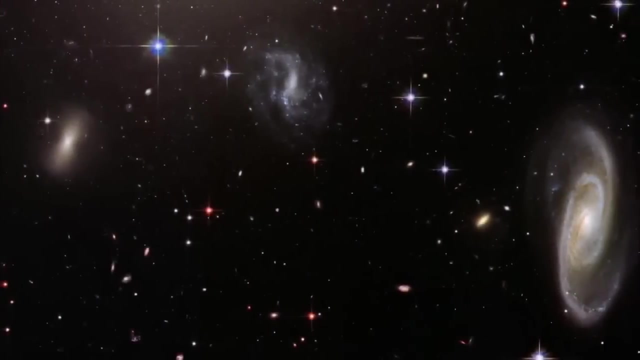 that are actually being drawn together in a merger. This is how galaxies build themselves, Right? Mario Livio is on the team working with the images from the Hubble Space Telescope. For decades, scientists have used Hubble to gaze far beyond our solar system. 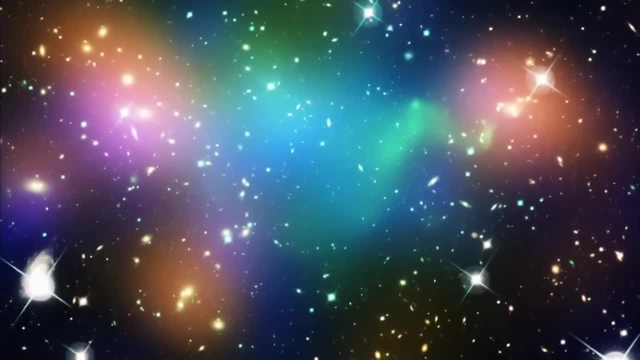 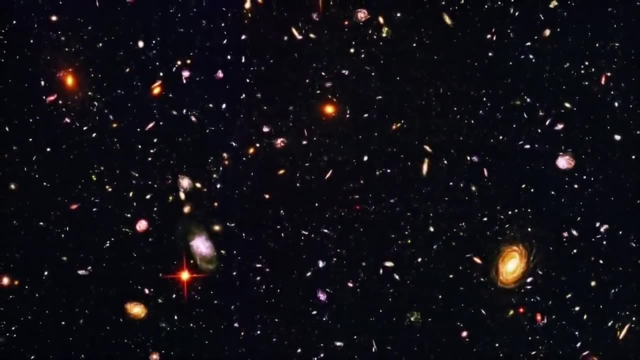 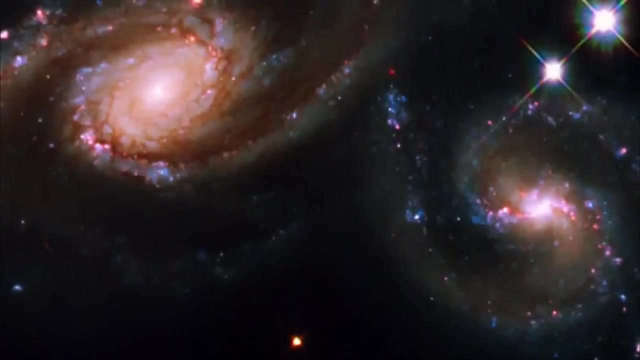 even beyond the stars of our galaxy. It's shown us distant gas clouds of nebulae and vast numbers of galaxies wheeling in the heavens billions of light years away. And what those images show is that throughout the visible universe as far as the telescope can see, 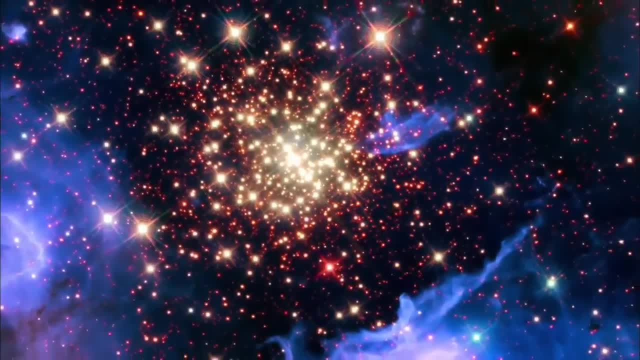 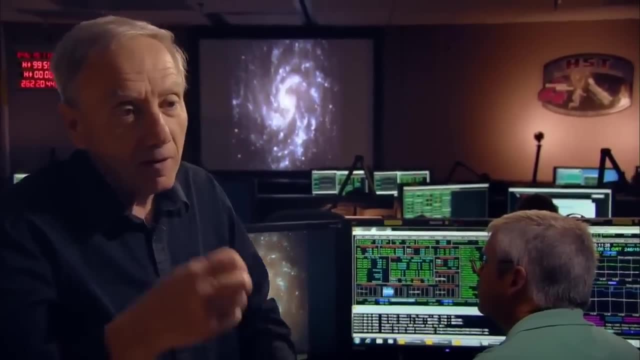 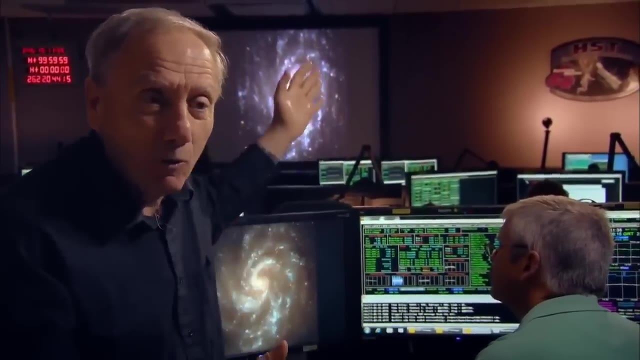 the law of gravity still applies. You know, Newton wrote these laws of gravity and of motion based on things happening on Earth and the planets and the solar system and so on. But these same laws, these very same laws, apply to all these distant galaxies. 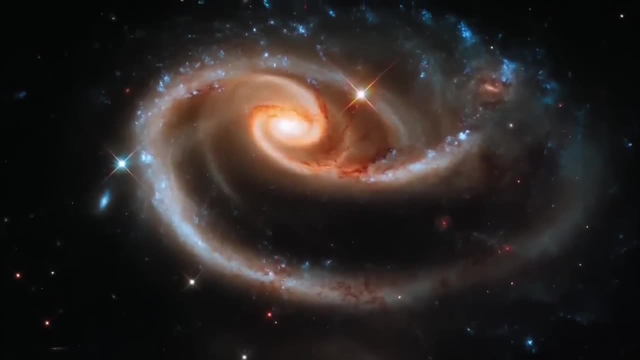 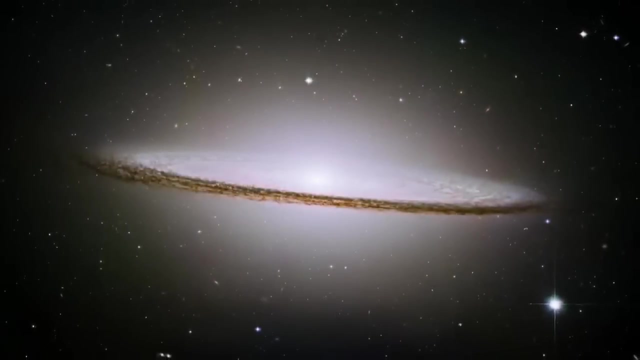 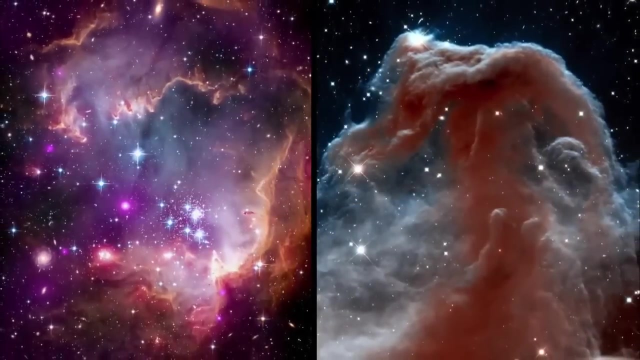 and you know, shape them and everything about them- how they form, how they move- is controlled by those same mathematical laws. Some of the world's greatest minds have been amazed by the way that math permeates the universe- Albert Einstein. 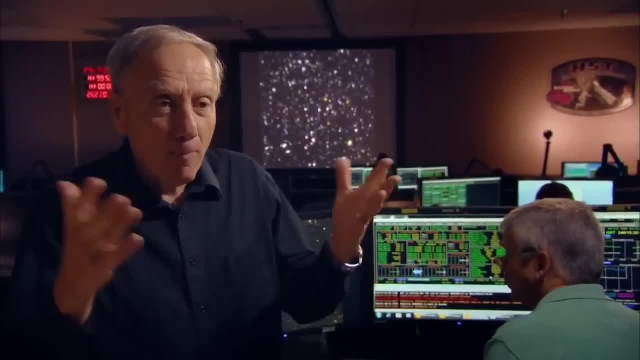 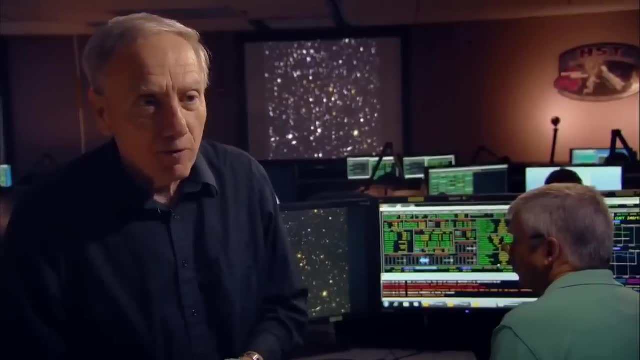 he wondered. he said: how is it possible that mathematics, which is, he thought, a product of human thought, does so well in explaining the universe as we see it? And Nobel laureate in physics Eugene Wigner coined this phrase. 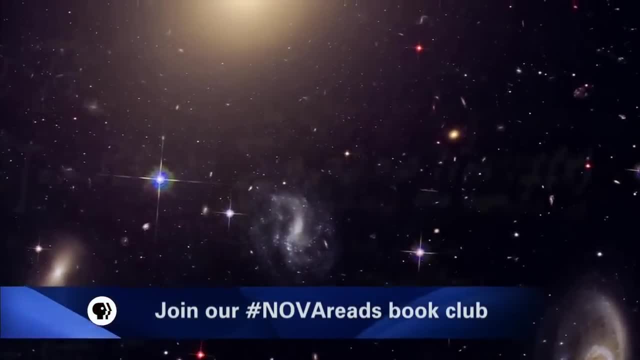 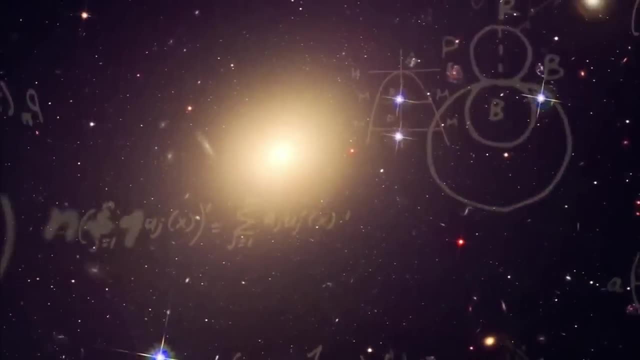 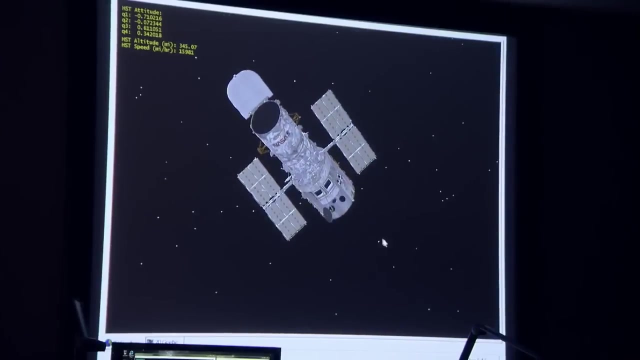 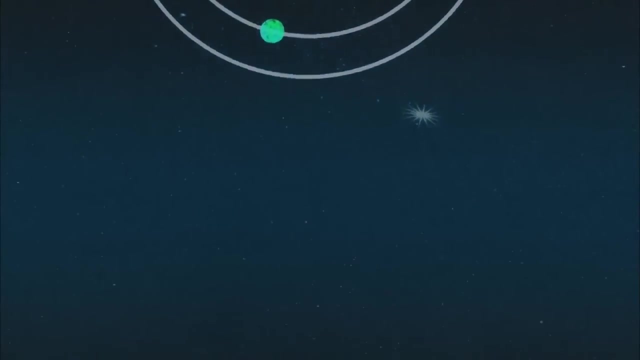 the unreasonable effectiveness of mathematics. He said that the fact that mathematics can really describe the universe so well, in particular physical laws, is a gift that we neither understand nor deserve. In physics, examples of that unreasonable effectiveness abound. When, nearly 200 years ago, 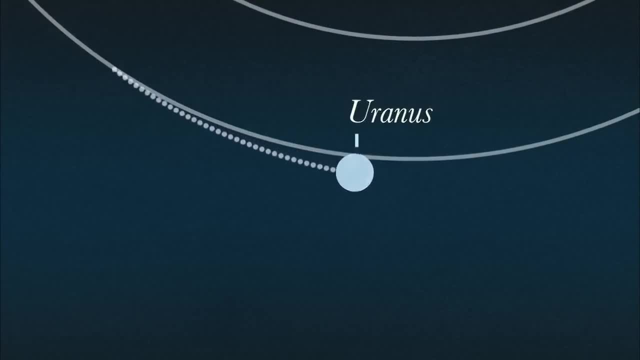 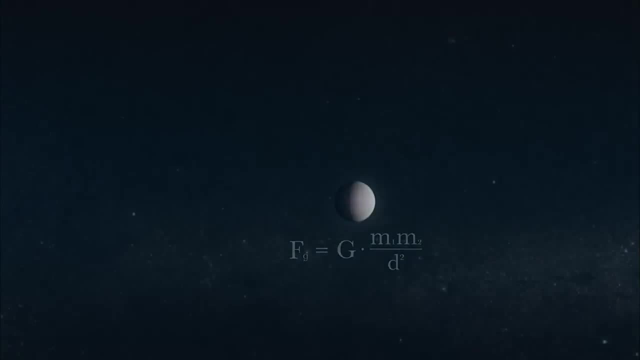 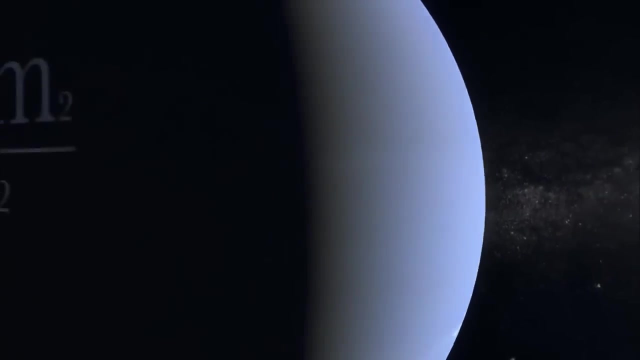 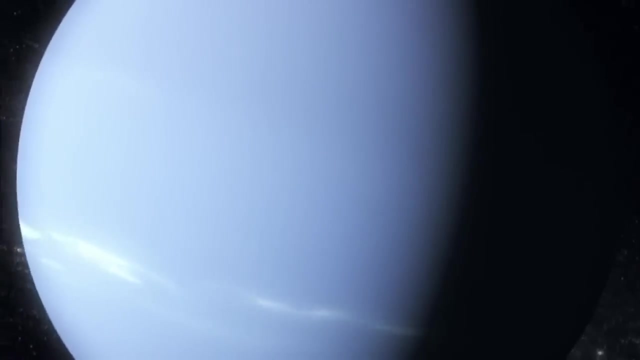 the planet Uranus was seen to go off track, scientists trusted the math and calculated it was being pulled by another unseen planet, And so they discovered Neptune. Mathematics had accurately predicted a previously unknown planet. If you formulate a question properly, mathematics gives you the answer. 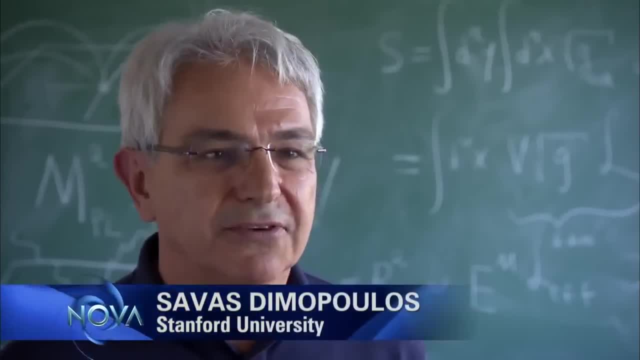 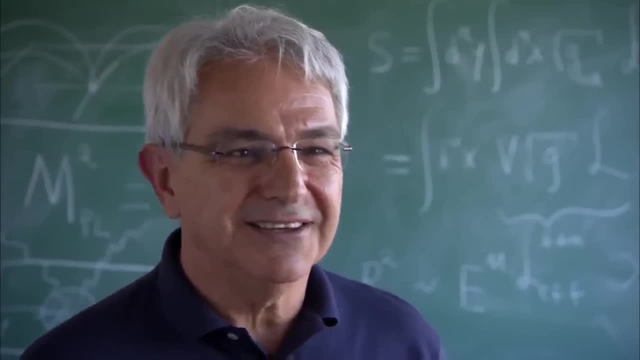 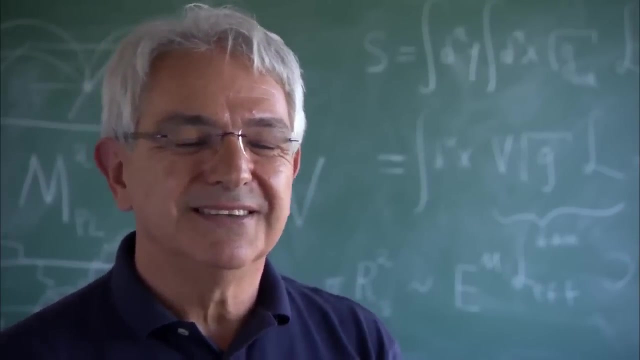 It's like having a servant that is far more capable than you are. so you tell it: do this, and if you say it nicely, then it will do it and it will carry you all the way to the truth, to the final answer. 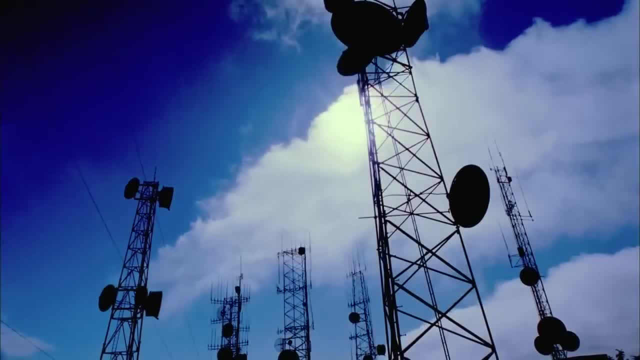 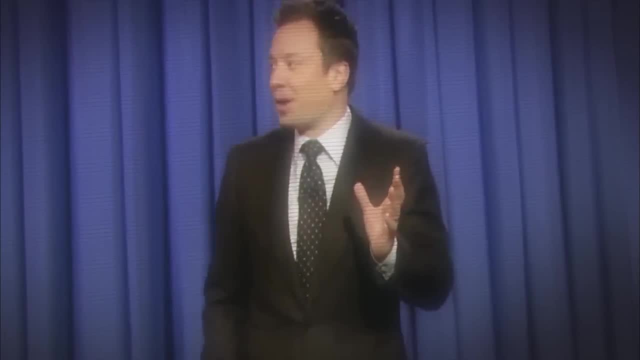 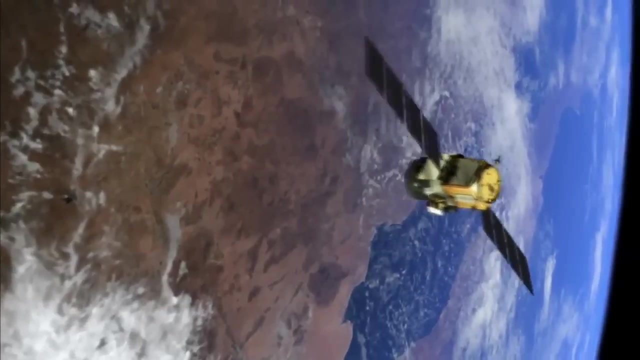 WDVH 89.7. Evidence of the amazing predictive power of mathematics can be found all around us. I heard it took five Elvises to pull them apart. Television, radio, your cell phone satellites, the baby monitor, Wi-Fi. 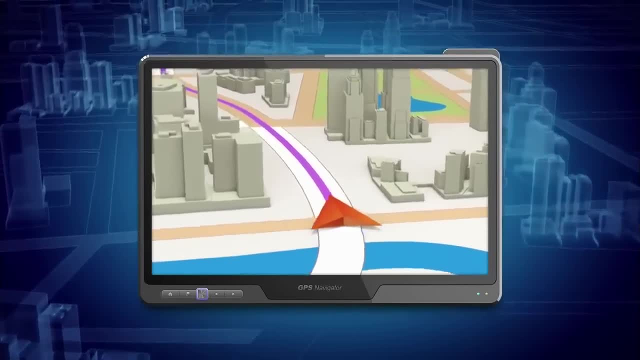 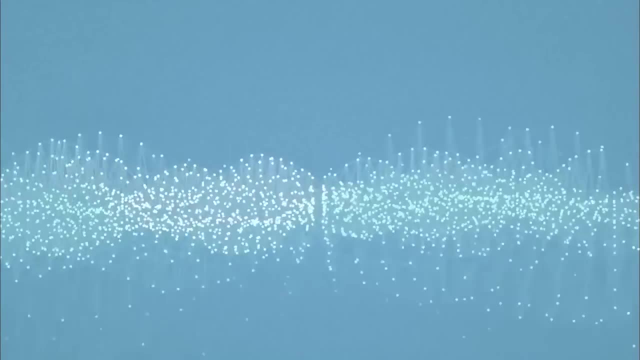 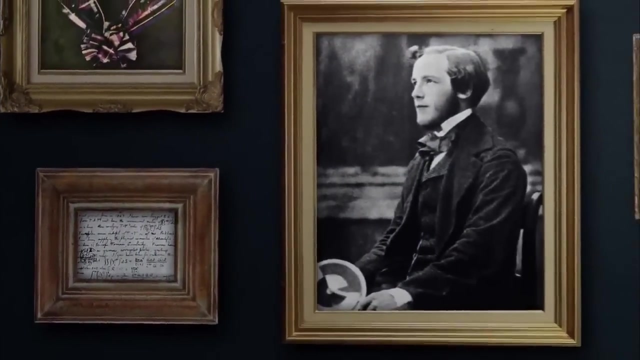 your garage door opener, GPS and, yes, even maybe your TV's remote. All of these use invisible waves of energy to communicate and no one even knew they existed until the work of James Maxwell, a Scottish mathematical physicist, In the 1860s. 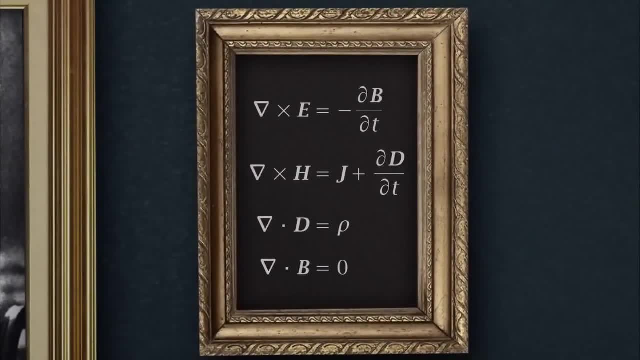 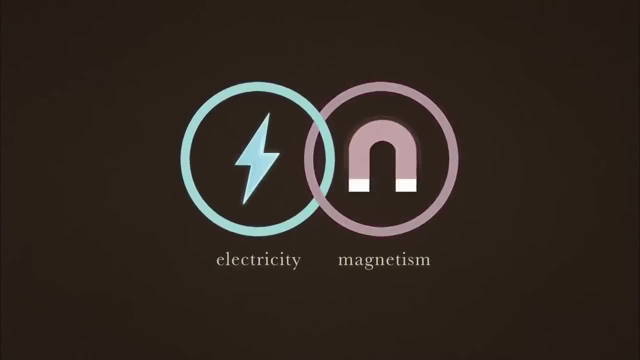 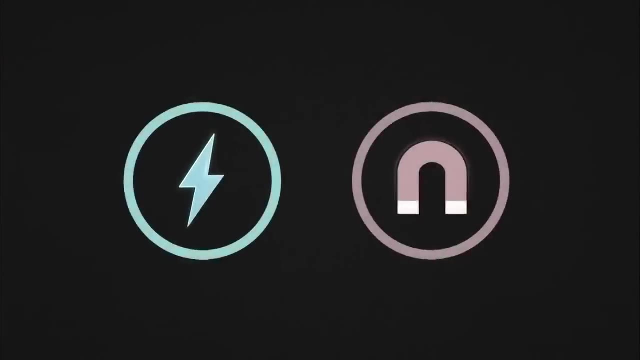 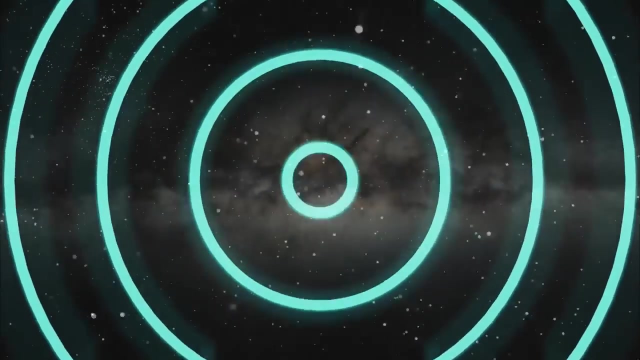 he published a set of equations that explained how electricity and magnetism were related, how each could generate the other. The equations also made a startling prediction: Together, electricity and magnetism could produce waves of energy that would travel through space at the speed of light. 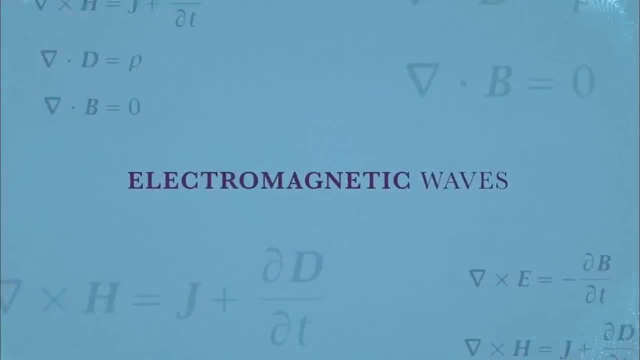 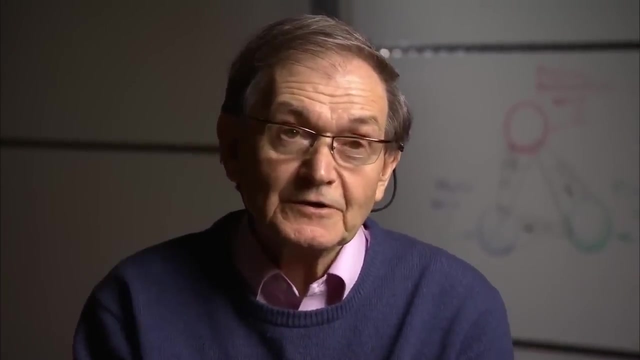 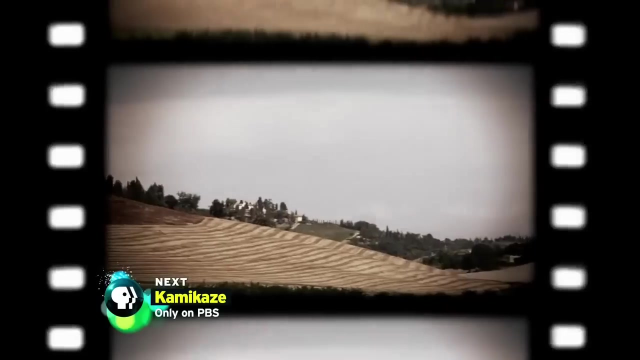 Electromagnetic waves. Maxwell's theory gave us these radio waves, X-rays, these things which were simply not known about at all. So the theory had a scope which was extraordinary. Almost immediately, people set out to find the waves predicted by Maxwell's equations. 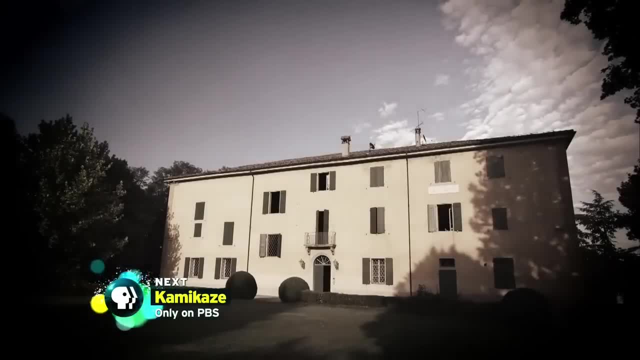 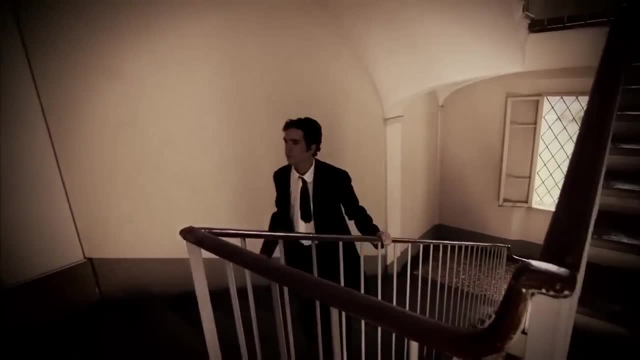 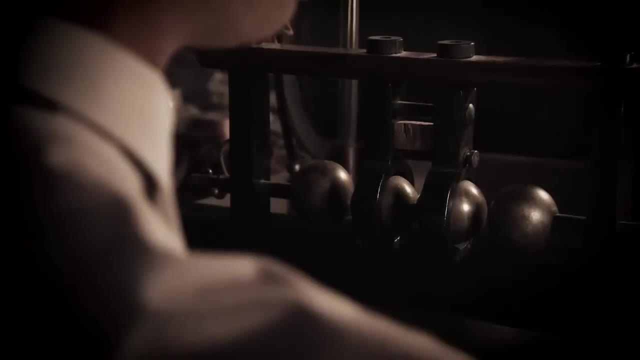 What must have seemed the least promising attempt to harness them is made here in northern Italy, in the attic of a family home, by 20-year-old Guglielmo Marconi. His process starts with a series of sparks, The burst of electricity. 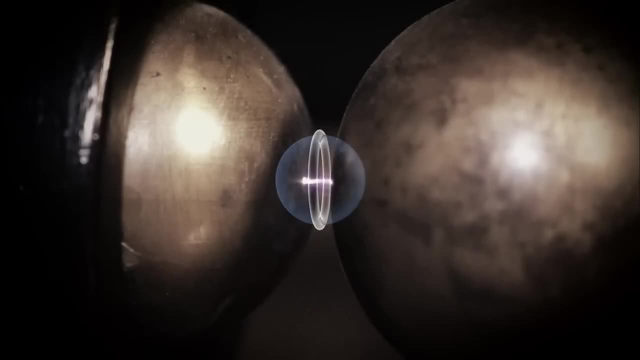 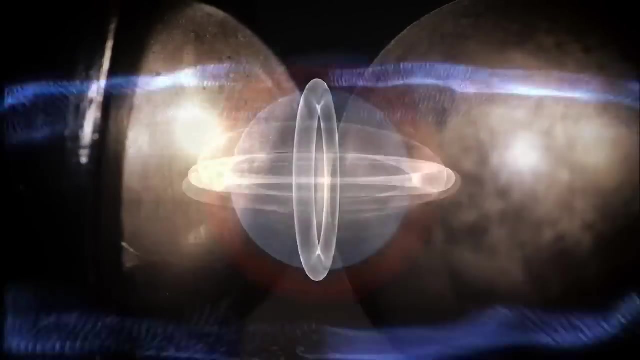 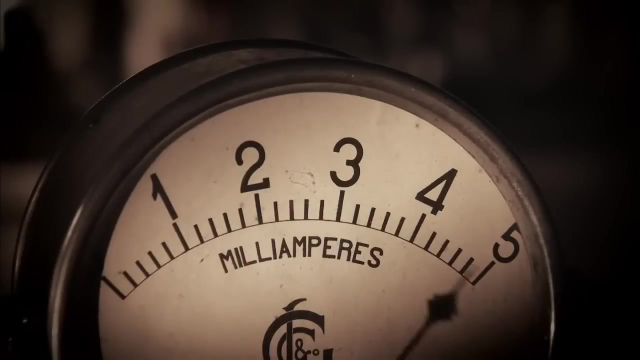 creates a momentary magnetic field, which in turn generates a momentary electric field, which creates another magnetic field, The energy cycles between the two propagating an electromagnetic wave. Marconi gets his system to work inside, but then he scales up. 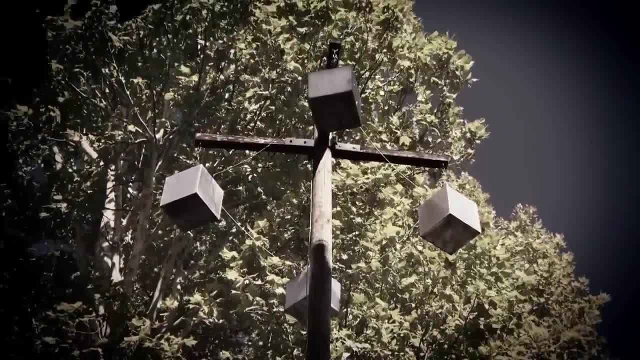 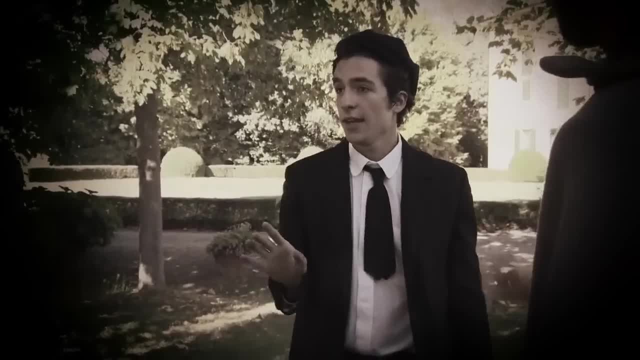 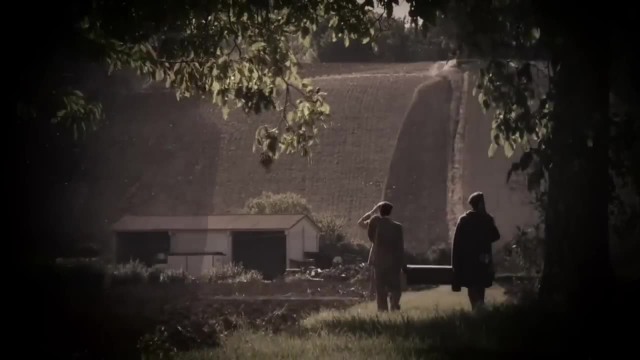 Over a few weeks he builds a big antenna beside the house to amplify the waves coming from his spark generator. Then he asks his brother and an assistant to carry a receiver across the estate to the far side of a nearby hill. They also have a shotgun. 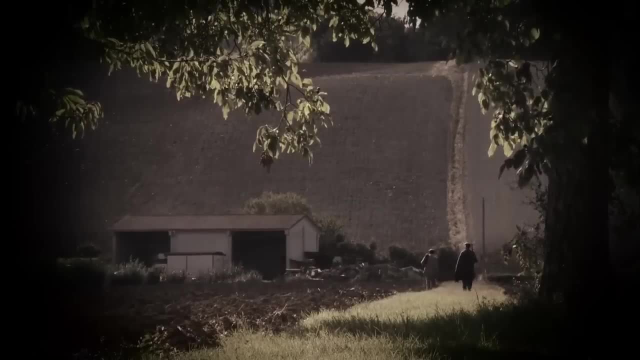 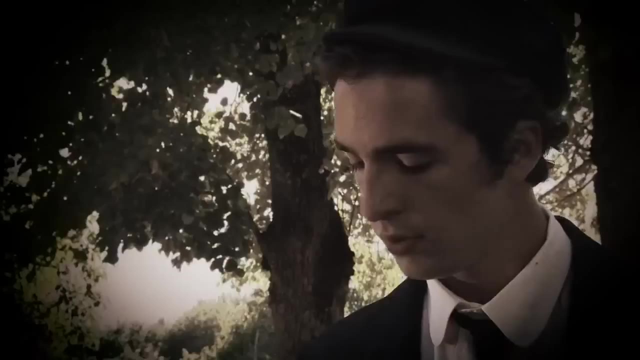 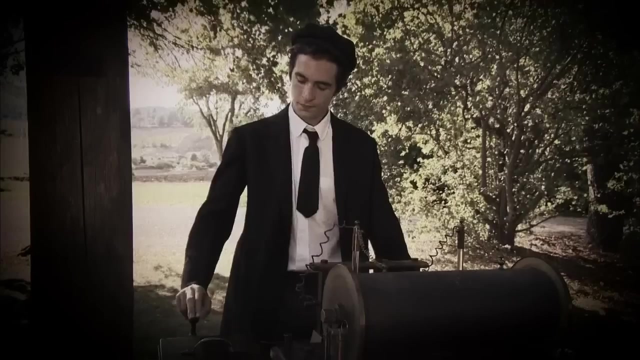 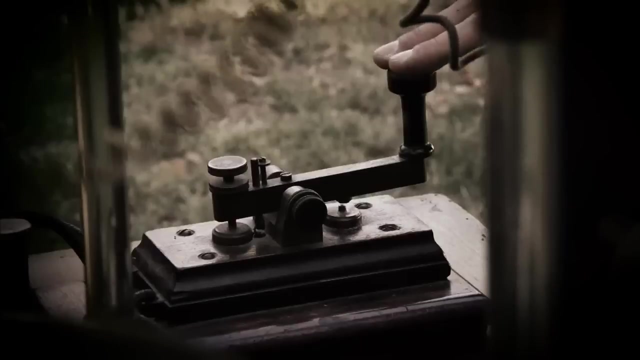 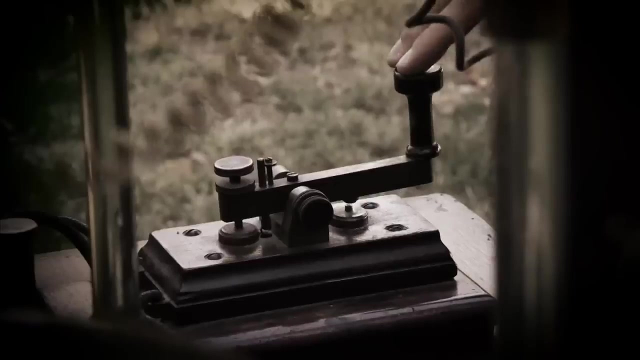 which they will fire if they manage to pick up the signal. And it works. The signal has been detected even though the receiver is now hidden behind a hill At over a mile. it is the farthest transmission to date, In fewer than 10 years. 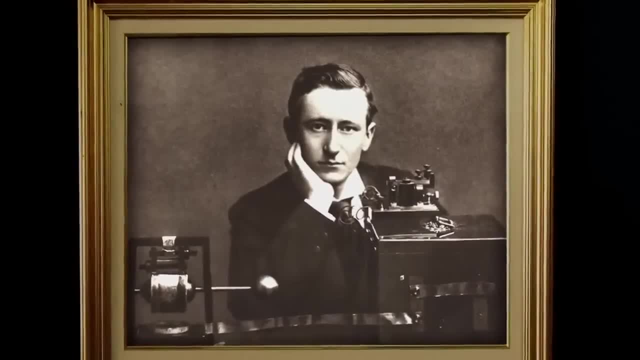 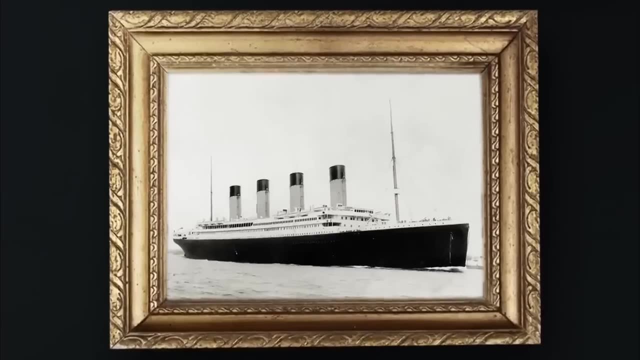 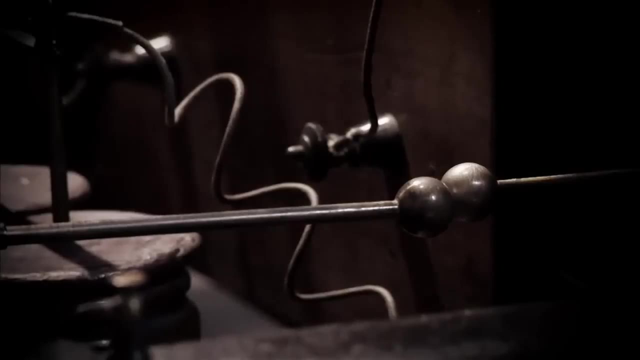 Marconi will be sending radio signals across the Atlantic. In fact, when the Titanic sinks in 1912, he'll be personally credited with saving many lives because his onboard equipment allowed the distress signal to be transmitted, Thanks to the predictions of Maxwell's equations. 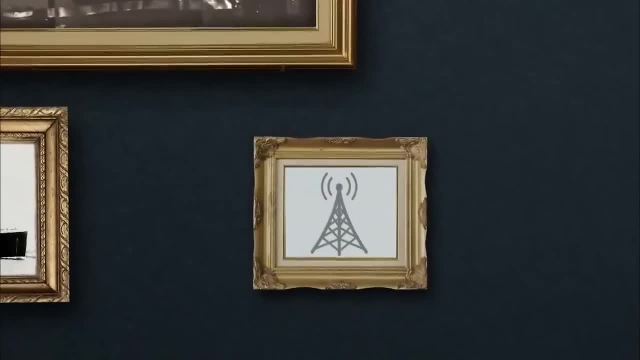 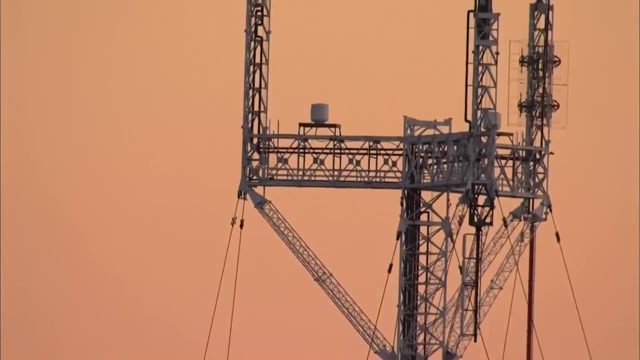 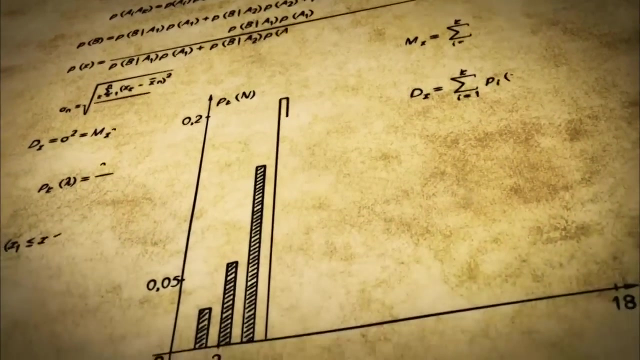 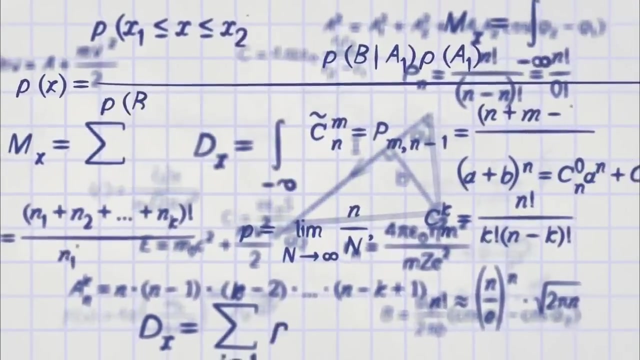 Marconi could harness a hidden part of our world, ushering in the era of wireless communication. Since Maxwell and Marconi, evidence of the predictive power of mathematics has only grown, especially in the world of physics. A hundred years ago, we barely knew atoms existed. 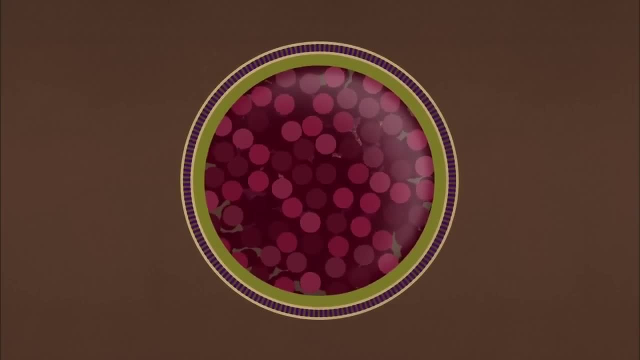 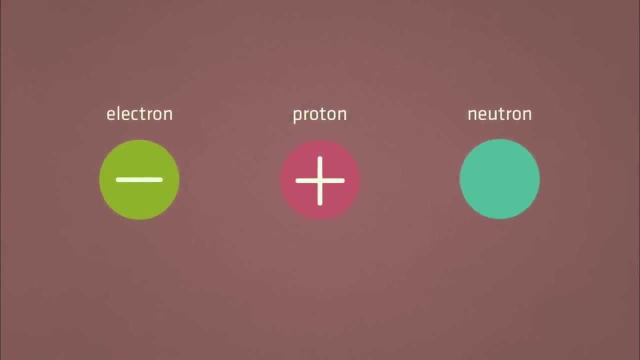 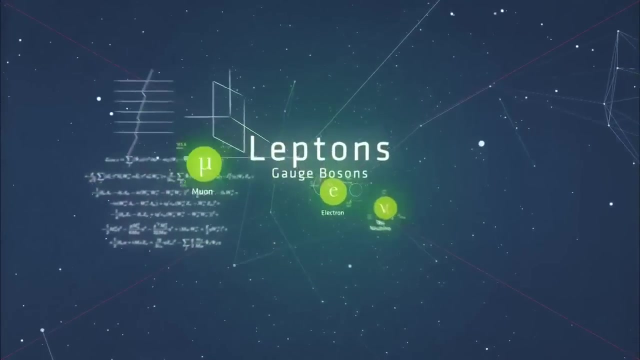 It took experiments to reveal their components: the electron, the proton and the neutron. But when physicists wanted to go deeper, mathematics began to lead the way. Ultrasound and quantum mechanics began to lead the way, Ultimately revealing a zoo of elementary particles. 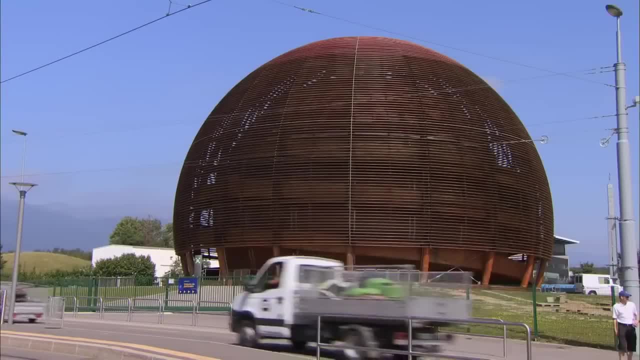 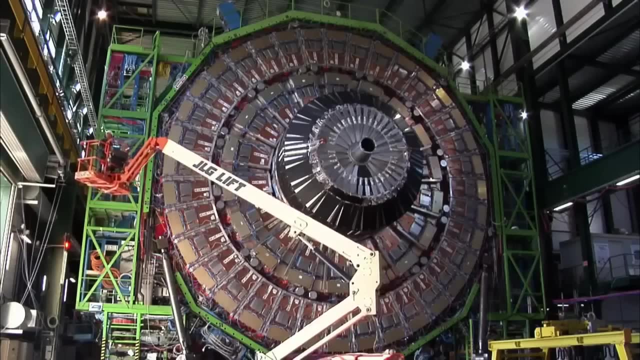 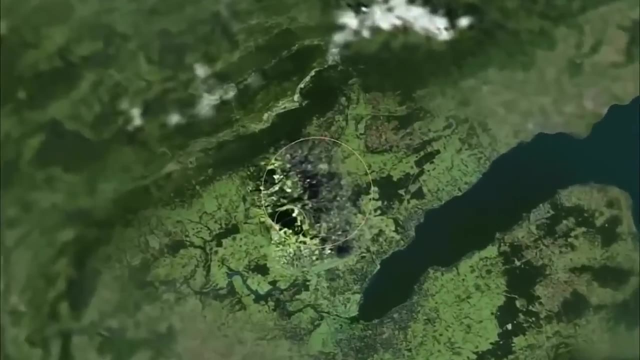 Discoveries that continue to this day here at CERN, the European Organization for Nuclear Research in Geneva, Switzerland. These days they're most famous for their Large Hadron Collider, a circular particle accelerator about 17 miles around, built deep underground. 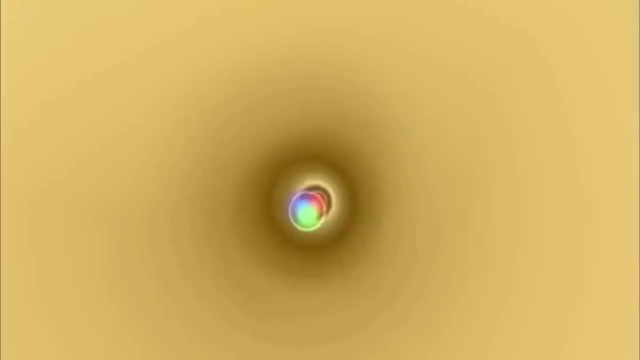 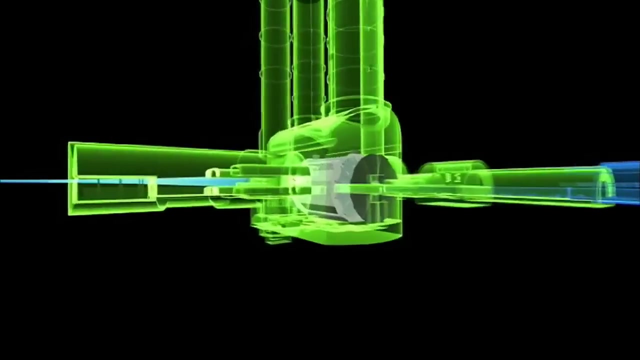 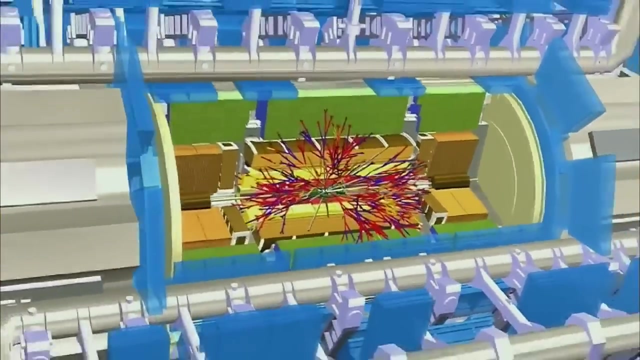 This $10 billion project, decades in the making, had a well-publicized goal: the search for one of the most fundamental building blocks of the universe: A subatomic particle mathematically predicted to exist nearly 50 years earlier by Robert Braut. 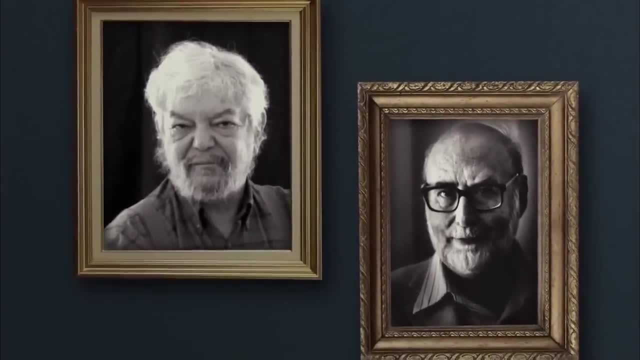 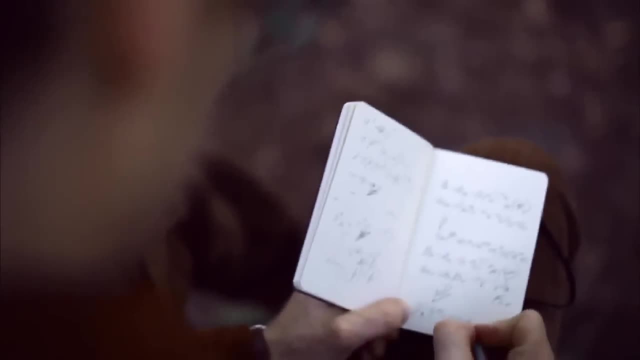 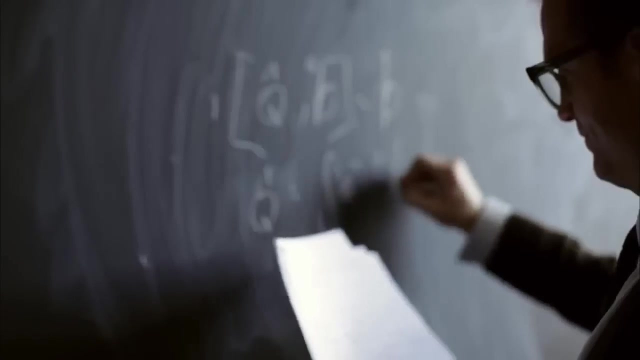 and Francois Englert working in Belgium, and Peter Higgs in Scotland. Peter Higgs sat down with the most advanced physics equations we had and calculated and calculated and made this audacious prediction that if we built the most sophisticated machines humans have ever built and used it to smash particles, 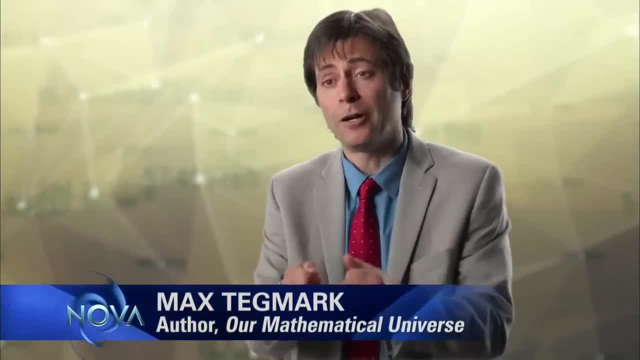 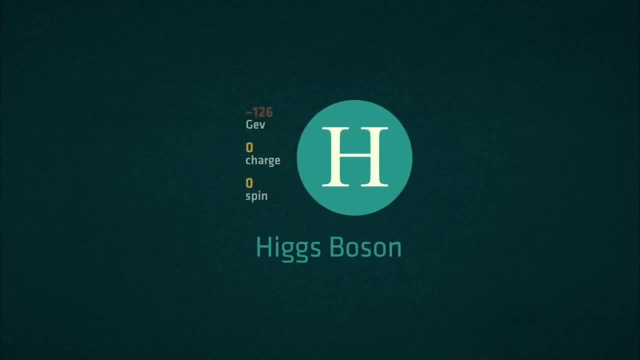 together near the speed of light in a certain way that we would there discover a new particle. and if this math was really accurate, The discovery of the Higgs particle would be proof of the Higgs field, a cosmic molasses. that gives the stuff. 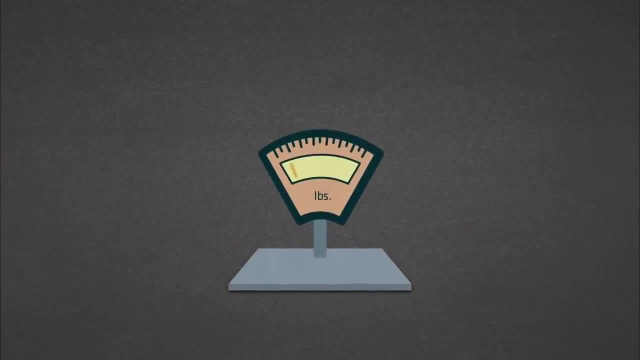 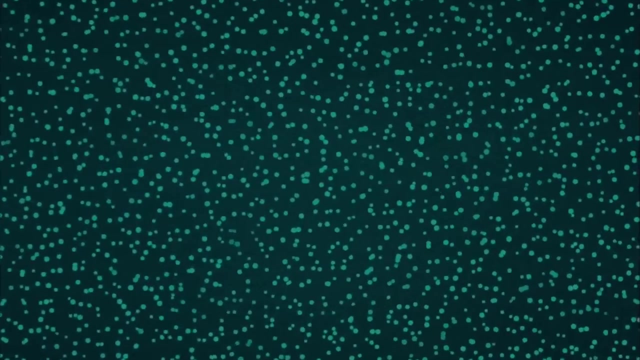 of our world mass, What we usually experience as weight. Without mass, everything would travel at the speed of light and would never combine to form atoms. That makes the Higgs field such a fundamental part of physics that the Higgs particle gained the nickname. 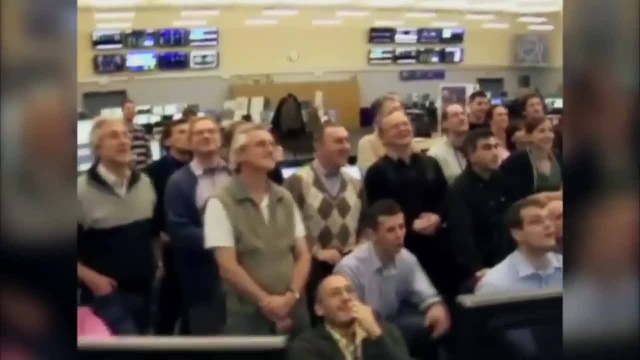 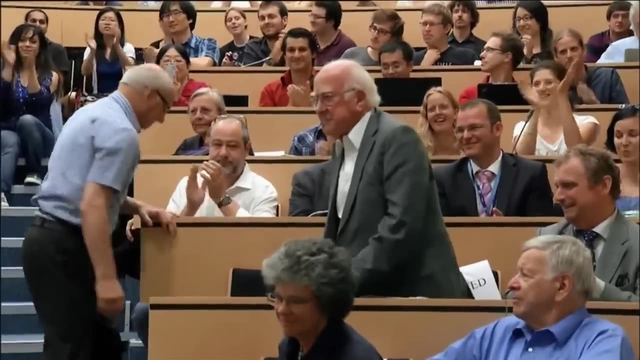 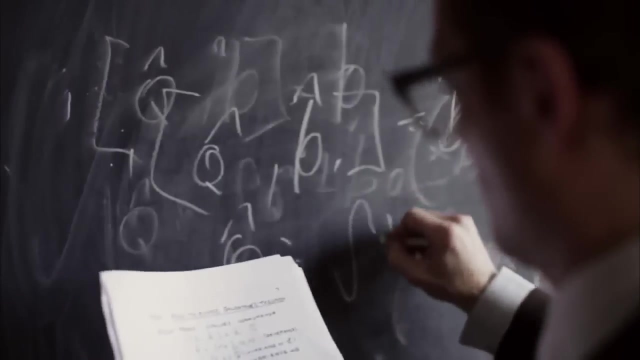 the God particle. In 2012,, experiments at CERN confirmed the existence of the Higgs particle in the atmosphere, making the work of Peter Higgs and his colleagues decades earlier one of the greatest predictions ever made. Well, we built it and it worked. 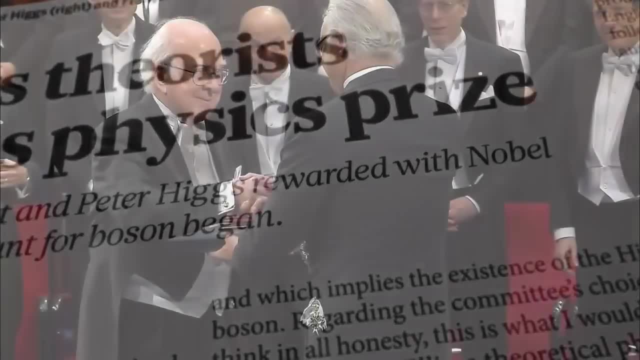 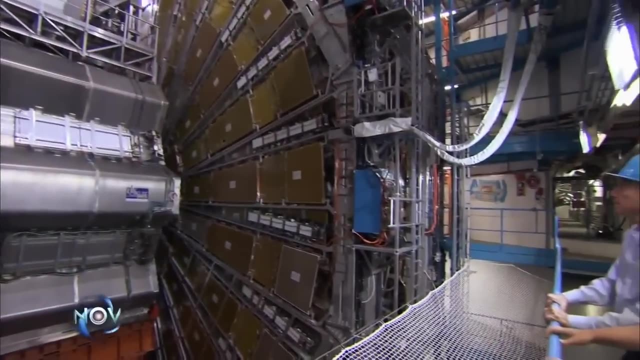 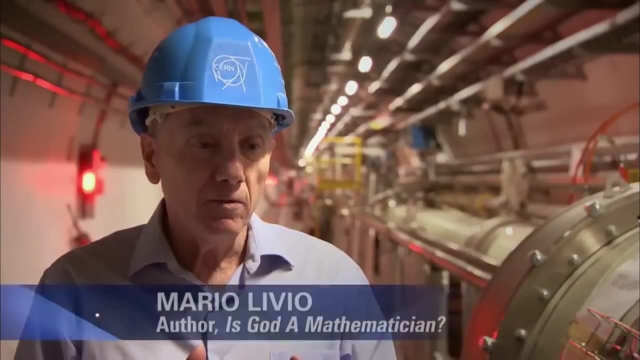 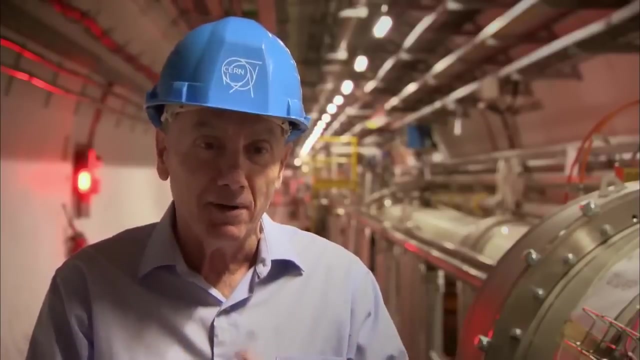 and he got a free trip to Stockholm. Here you have mathematical theories which make very difficult predictions about the possible existence of some fundamental particles of nature And, believe it or not, they make these huge experiments and they actually discover the particles that have been predicted. 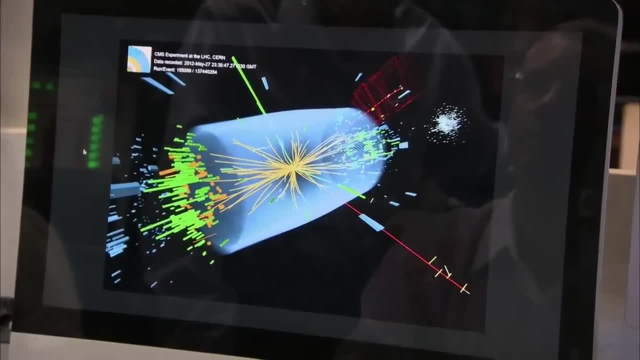 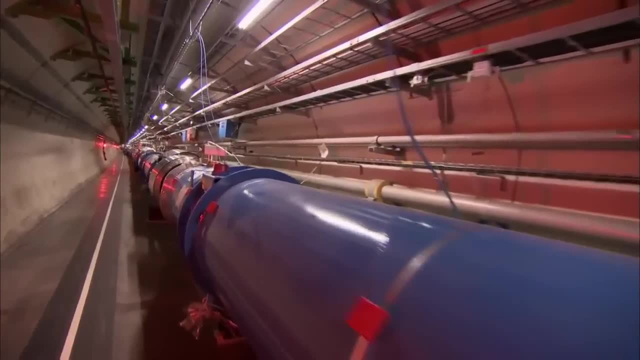 mathematically. I mean, this is just amazing to me. Why does this work? How can mathematics be so powerful? Is mathematics the only way to do this? Well, the only way to do this is to use the power of the Higgs particle. 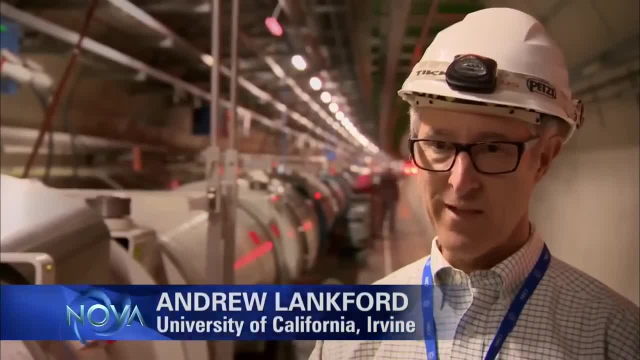 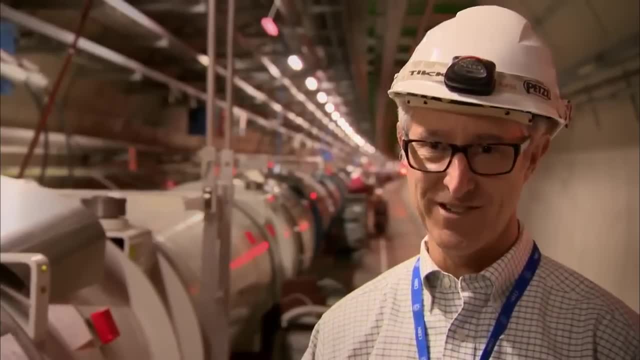 The Higgs particle is the most powerful particle in the universe. Is mathematics you know, a truth of nature, or does it have something to do with the way we, as humans, perceive nature? I mean, to me this is just a fascinating puzzle. 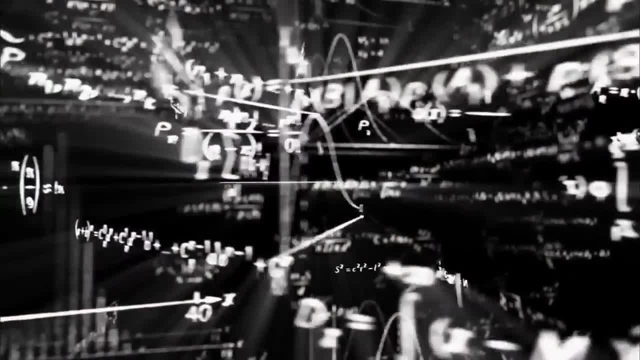 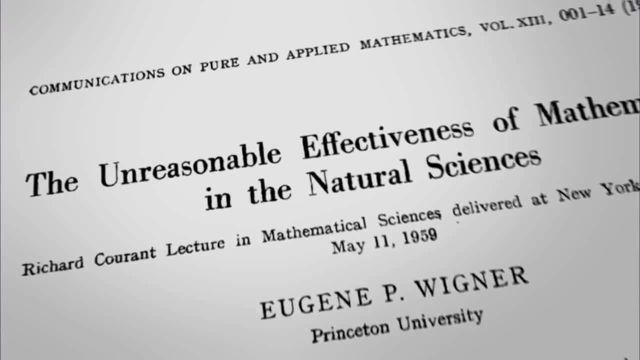 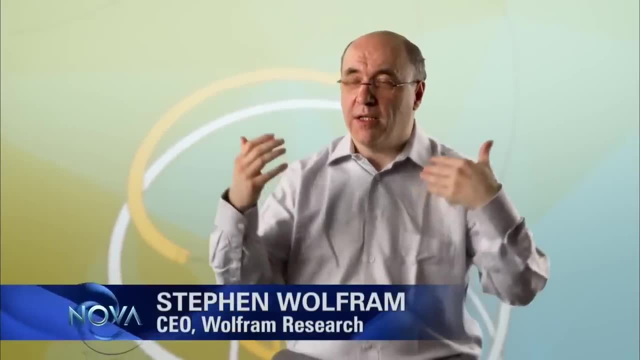 I don't know the answer. In physics, mathematics has had a long string of successes, But is it really unreasonably effective? Not everyone thinks so. I think it's an illusion, because I think what's happened is that people have chosen to build physics. 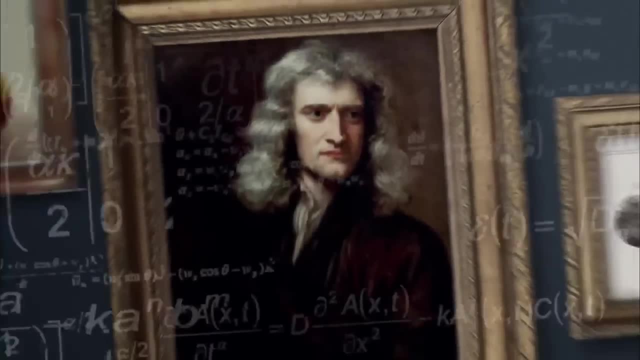 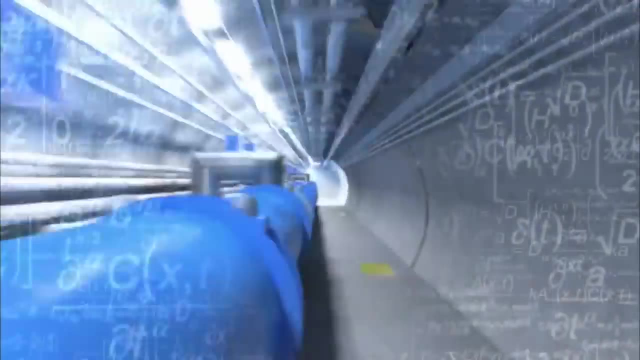 for example, using the mathematics that has been practiced, has developed historically, And then they're looking at everything. They're choosing to study things which are amenable to study using the mathematics that happens to have arisen, But actually there's a whole vast ocean. 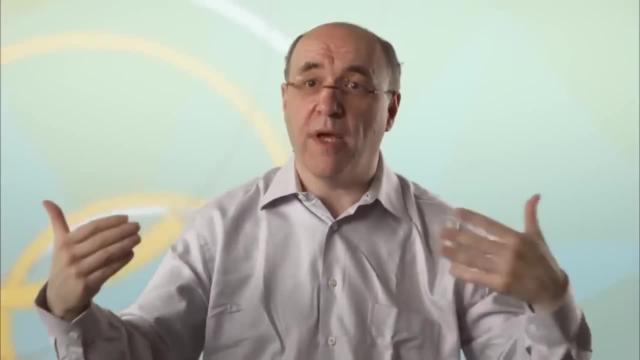 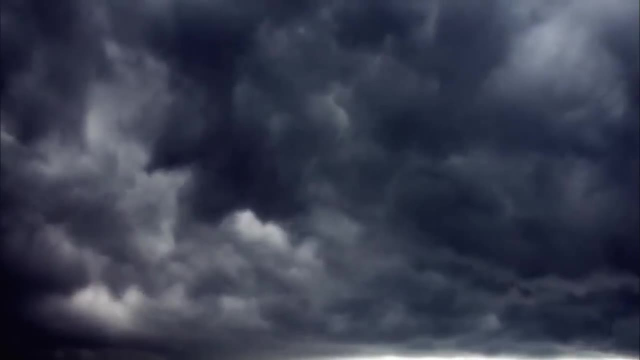 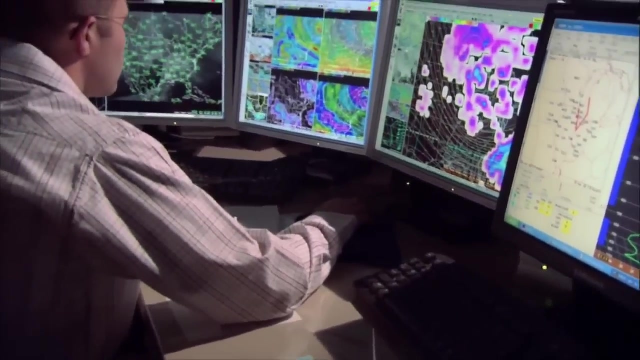 of other things that are really quite inaccessible to those methods. With the success of mathematical models in physics, it's easy to overlook where they don't work that well, Like in weather forecasting. There's a reason: meteorologists predict the weather for the coming week. 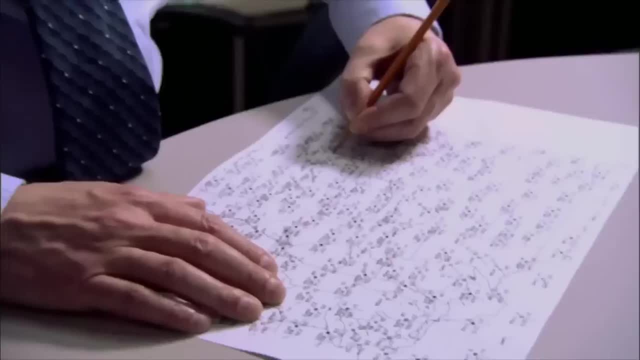 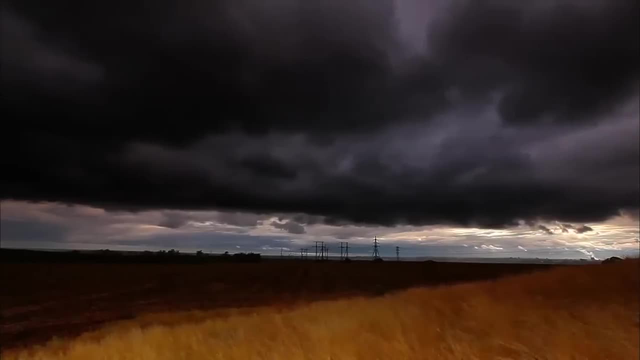 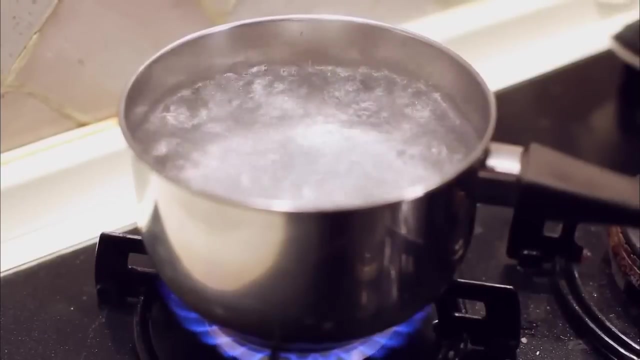 but not much further out than that In a longer forecast. small errors grow into big ones. Daily weather is just too complex and chaotic for precise modeling, And it's not alone. So is the behavior of water boiling on a stove Or the stock market. 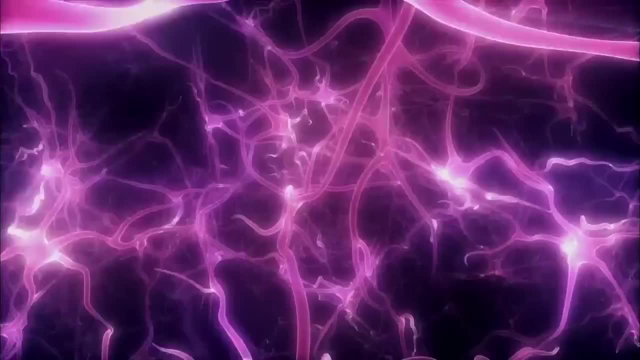 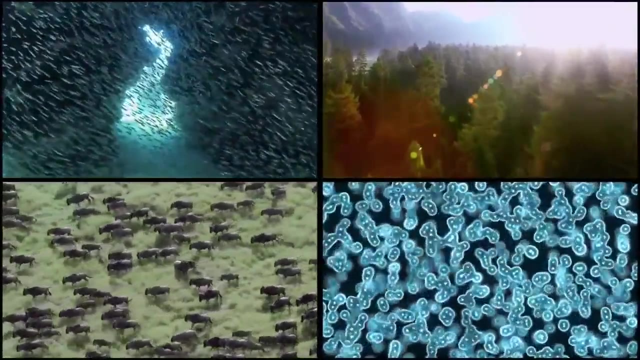 Or the interaction of neurons in the brain, Much of human psychology and parts of biology, Biological systems, economic systems. it gets very difficult to model those systems with math. We have extreme difficulty with that, So I do not see math as unreasonably effective. 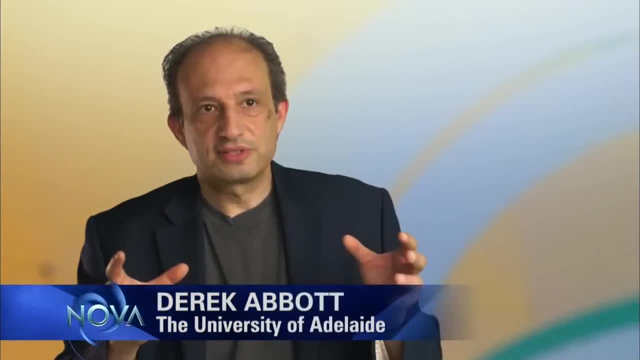 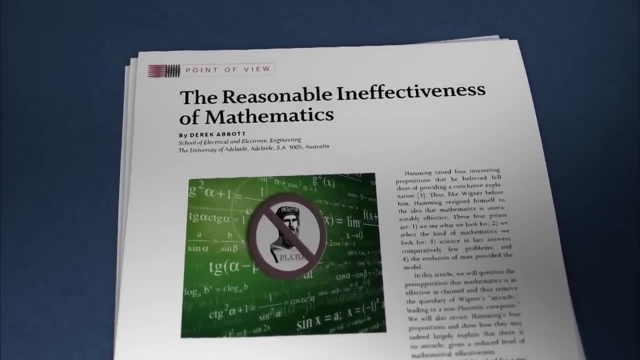 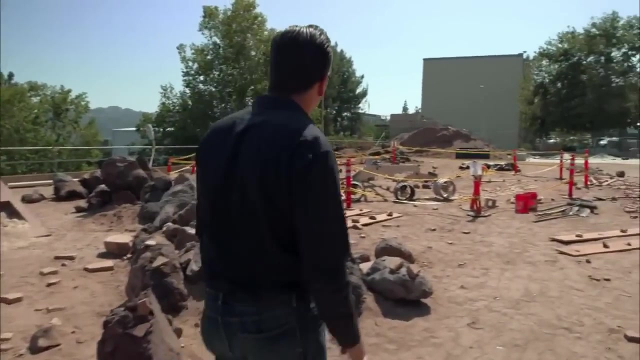 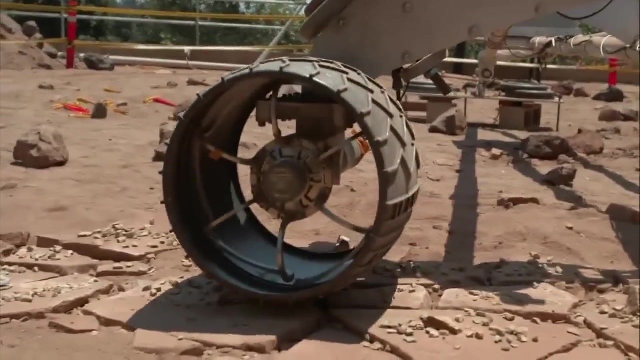 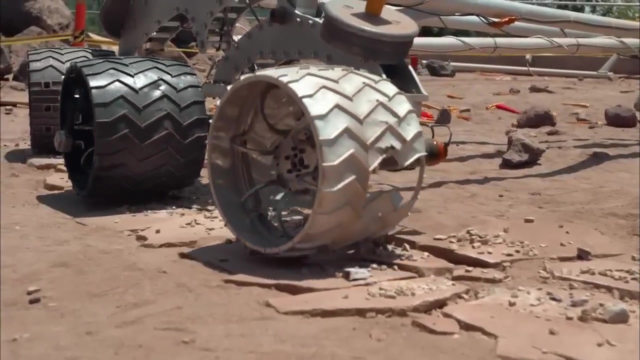 I see it as reasonably ineffective. Perhaps no one is as keenly aware of the power and limitations of mathematics as those who use it to design and make things. engineers, Look at that wheel In their work. the elegance of math meets the messiness. 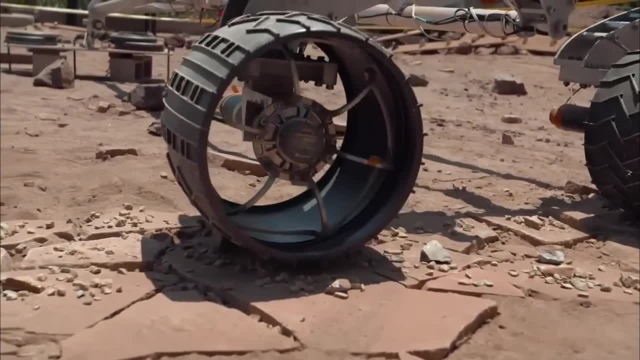 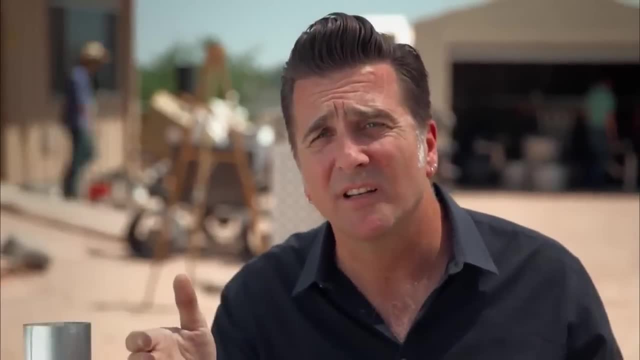 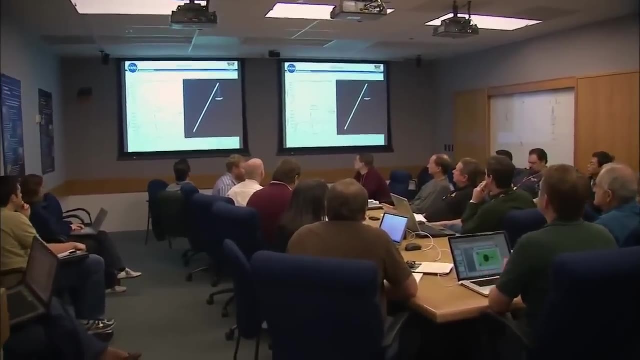 of reality and practicality rules the day. Mathematics, and perhaps mathematicians, deal in the domain of the absolute, And engineers live in the domain of the approximate. We are fundamentally interested in the practical, And so frequently we make approximations. 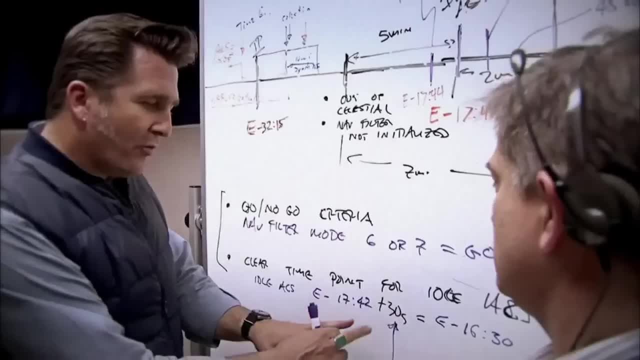 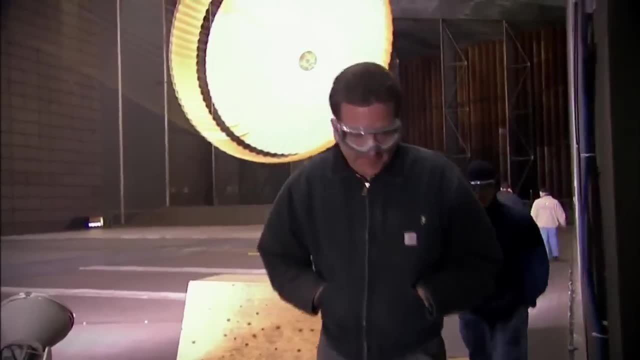 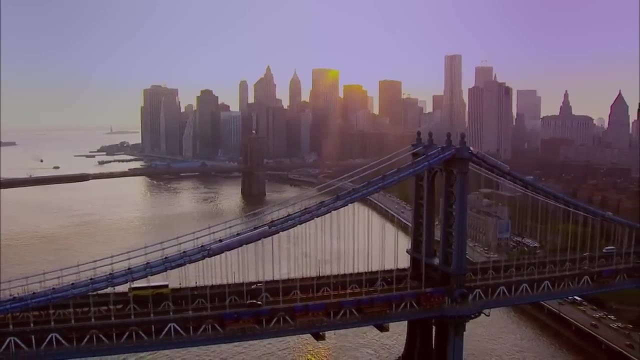 we cut corners, we omit terms and equations to get things that are simple enough to suit our purposes and to meet our needs. Many of our greatest engineering achievements were built using mathematical shortcuts Simplified to give us equations that approximate an answer, trading some precision. 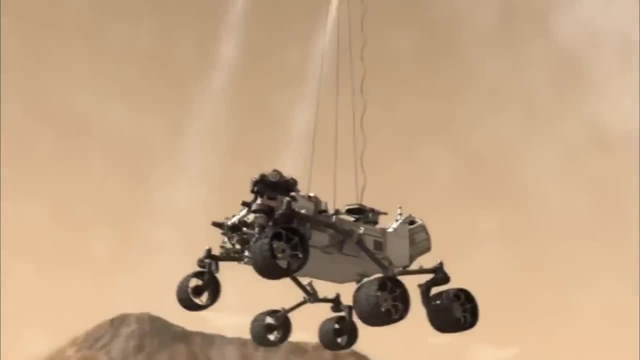 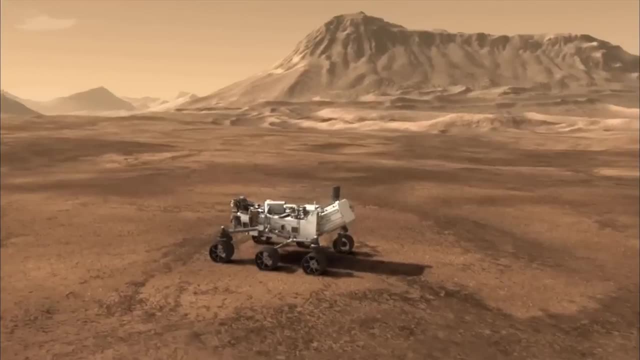 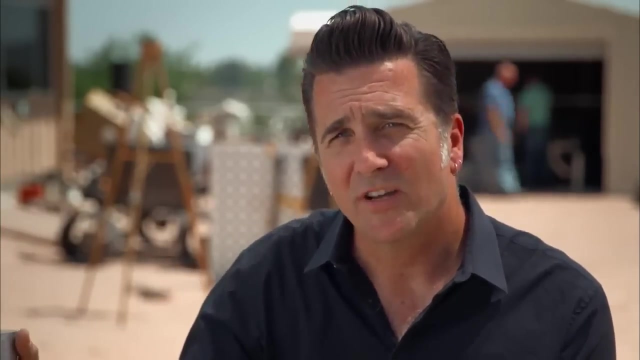 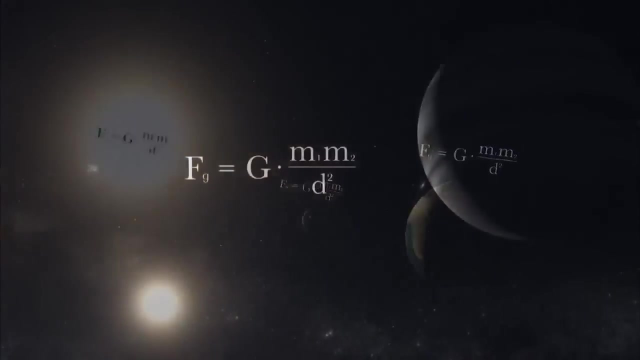 for practicality And for engineers, approximate is close enough. Close enough to take you to Mars. For us engineers, we don't get paid to do things right. We get paid to do things just right enough. Many physicists see an uncanny accuracy. 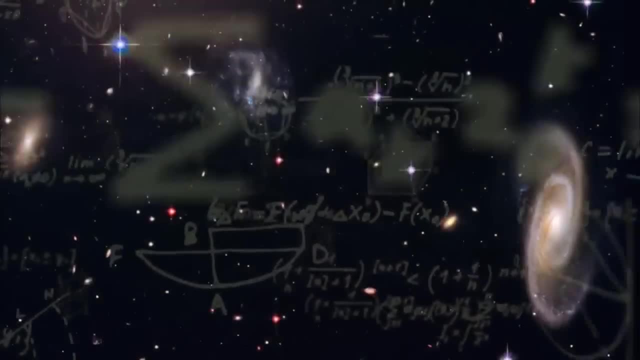 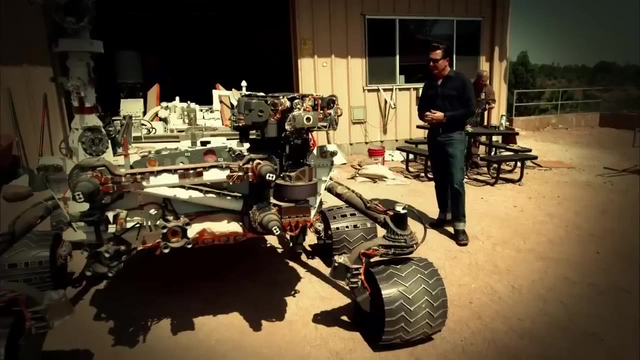 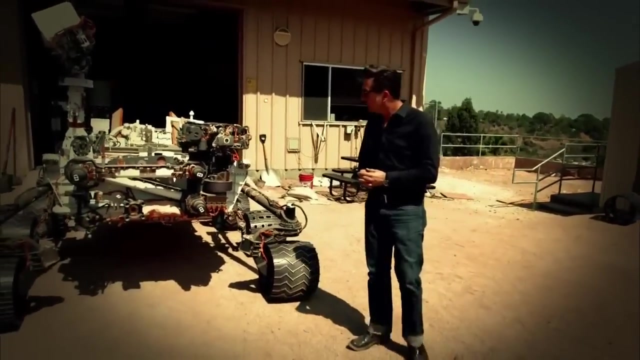 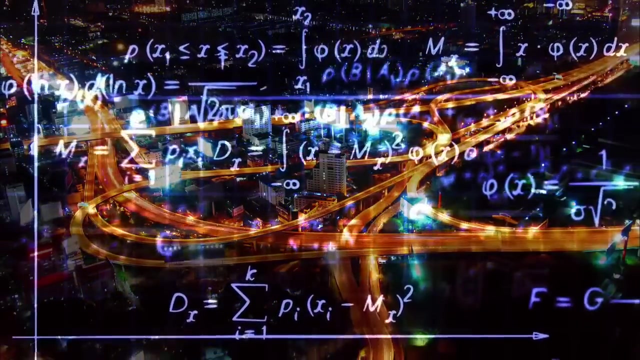 in the way mathematics can reveal the secrets of the universe, making it seem to be an inherent part of nature. Meanwhile, engineers in practice have to sacrifice the precision of mathematics to keep it useful, making it seem more like an imperfect tool of our own invention. 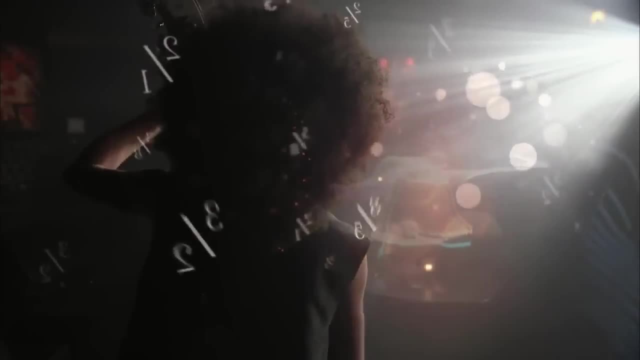 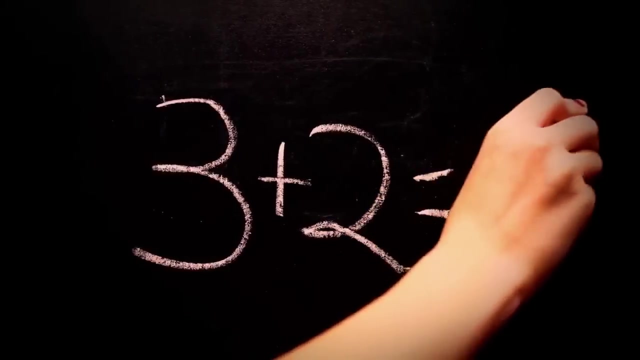 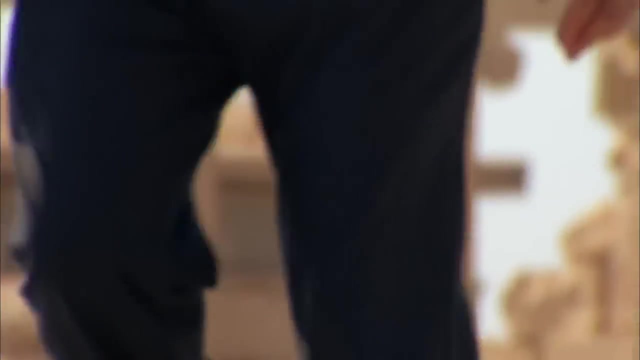 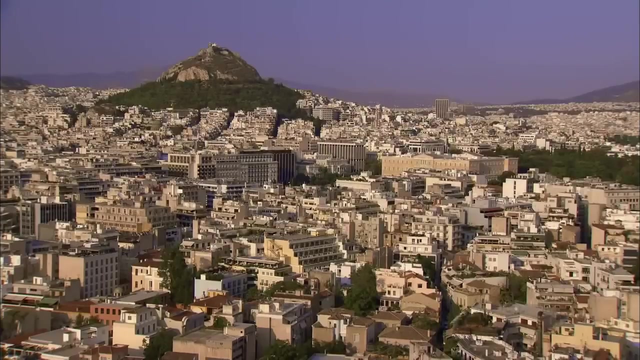 So which is mathematics? A discovered part of the universe Or a very human invention? Maybe it's both. What I think about mathematics is that it is an intricate combination of inventions and discoveries. So, for example, take something like natural numbers one, two, three, four. 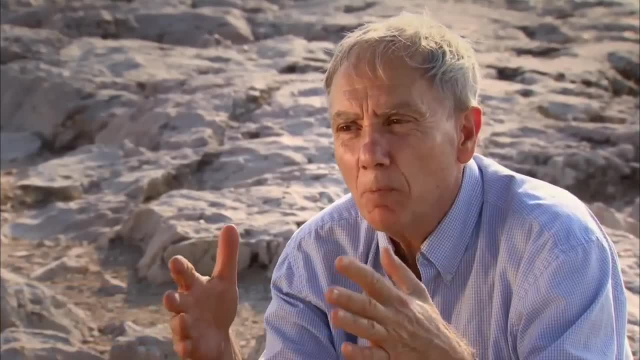 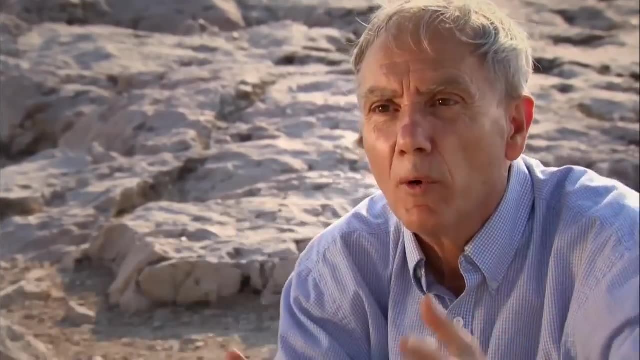 five, et cetera. I think what happened was that people were looking at many things, for example, and seeing that there are two eyes, you know, two breasts, two hands, you know, and so on, And after some time, 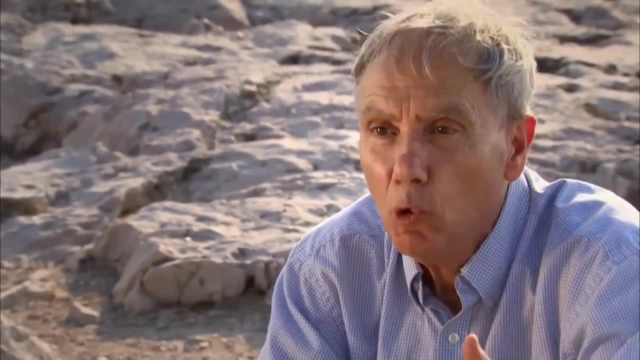 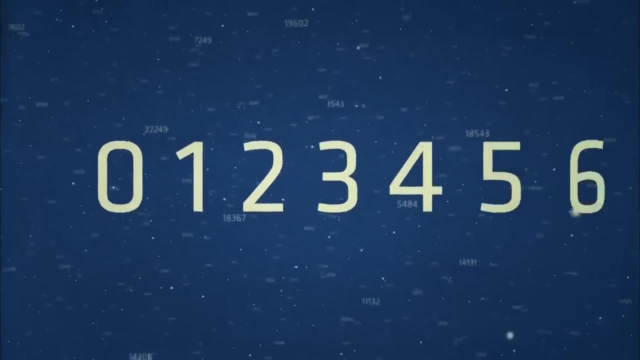 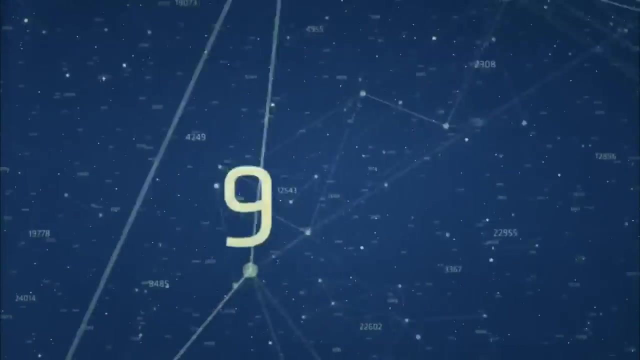 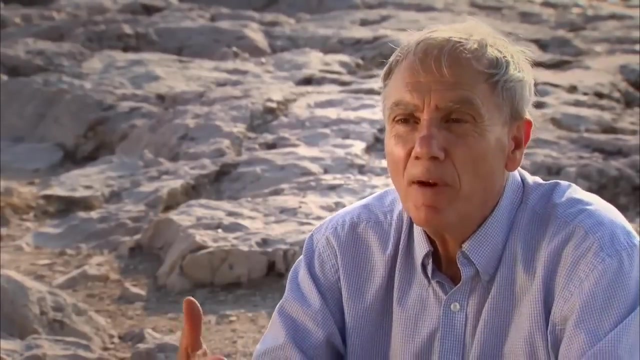 they abstracted from all of that. the number two, According to Mario two, became an invented concept, as did all the other natural numbers. But then people discovered that these numbers have all kinds of intricate relationships. Those were discovered as discoveries. We invented the concept. 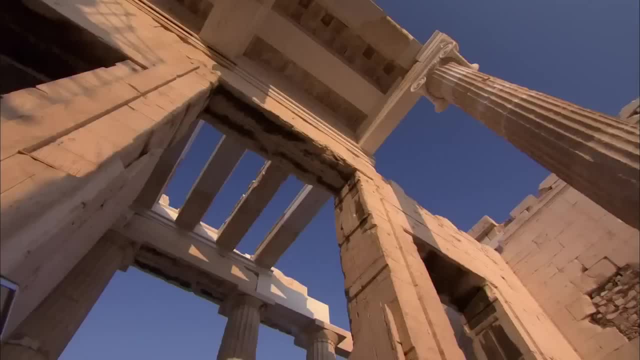 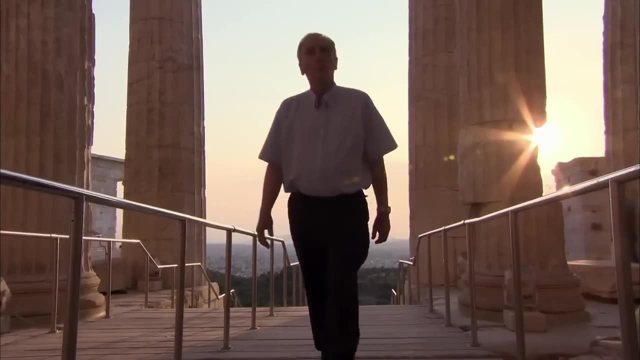 but then discovered the relations among the different concepts. So is this the answer: That math is both invented and discovered? This is one of those questions where it's both: Yes, it feels like it's already there, but yes, it's something. 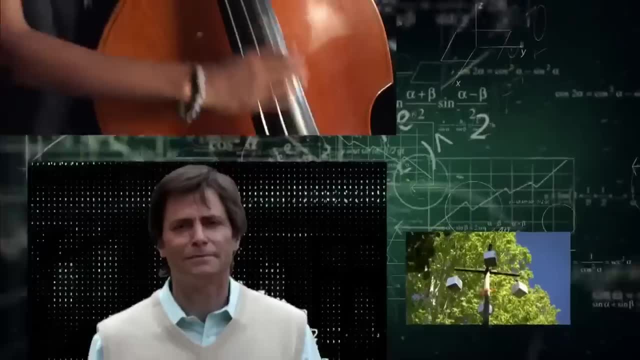 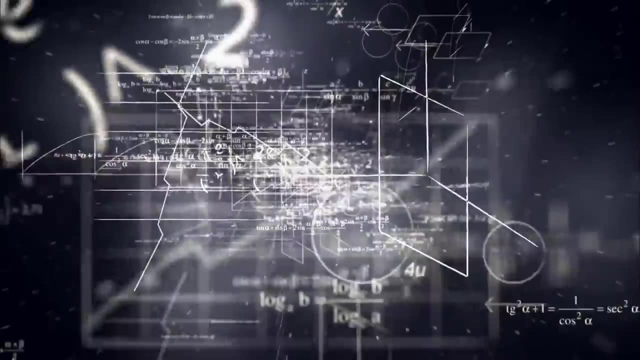 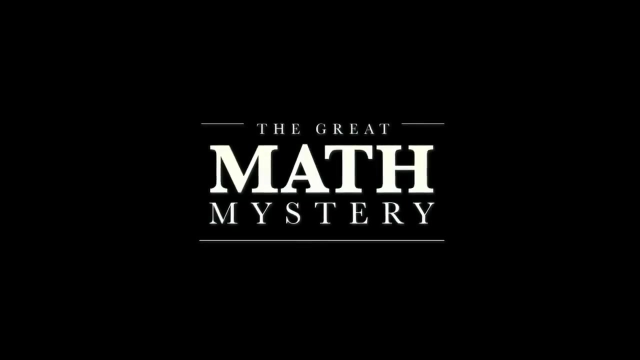 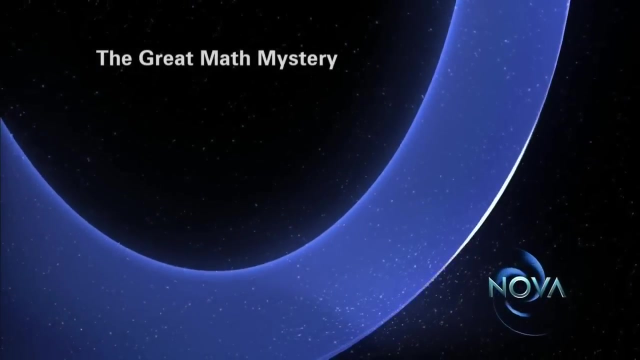 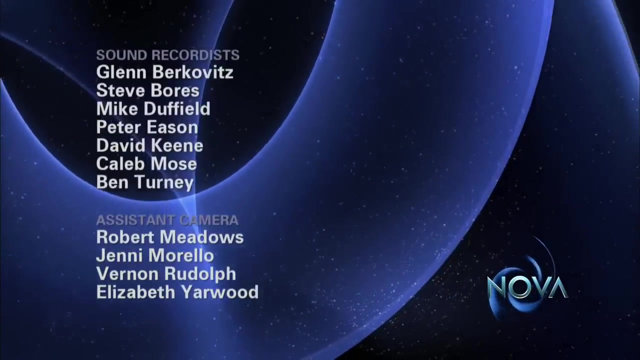 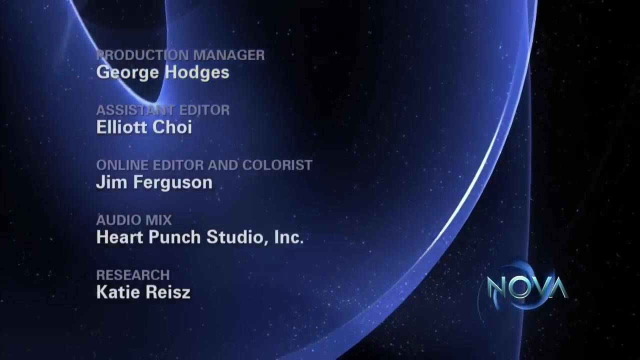 that comes out of our deep creative nature as human beings. We may have some idea to how all this works, but none is the complete answer. In the end, it remains the great math mystery. This Nova program is available on DVD To order.